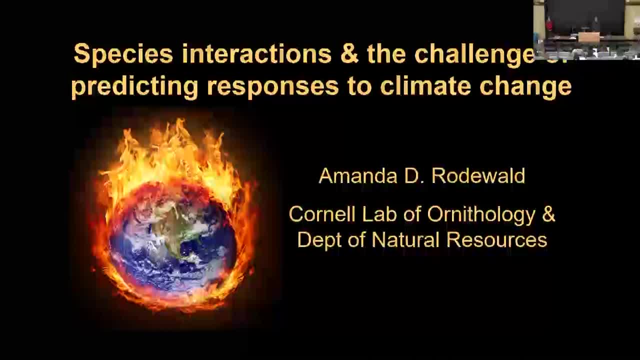 advance understanding of ecology and also support conservation. Her research seeks to understand how global change impacts ecosystems across multiple spatial temporal scales and levels of biological organization, and it touches such sub-disciplines as conservation, biology, community ecology, landscape ecology, pollution, demography, behavioral ecology. 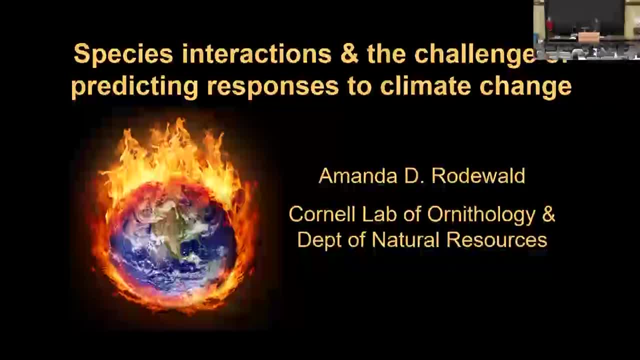 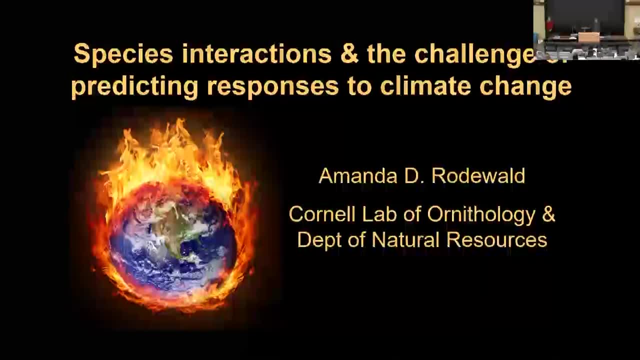 and ecological restoration. She tightly integrates the research and outreach efforts to inform policy and management and regularly interacts with government agencies, conservation organizations and private and landowners. So let's welcome Amanda Rodewald. Well, thanks everyone, and thanks, Peter for the invitation to be here. It's my pleasure. 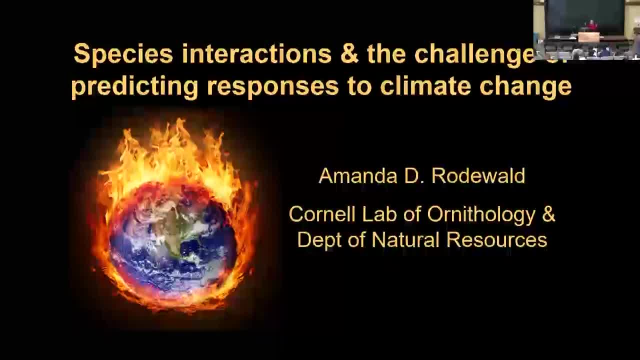 And, yeah, I'll just thank you all for coming into a room inside a building on a sunny and otherwise unseasonably warm day. So, yeah, what I'd like to do is really focus on one of the challenges that we face when we're trying to. 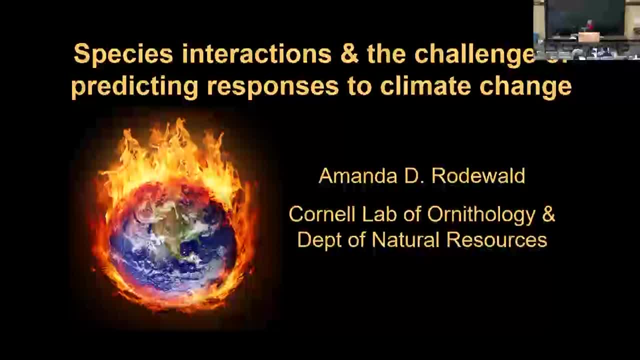 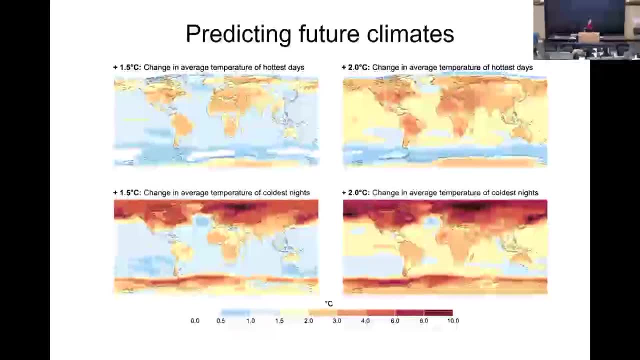 understand and predict how climate change is going to play out. you know around the planet, And so species interactions is what I'll be focusing on. But I first want to put this within the context of just how much progress we've made, just in general, with predicting how climates are likely to change. 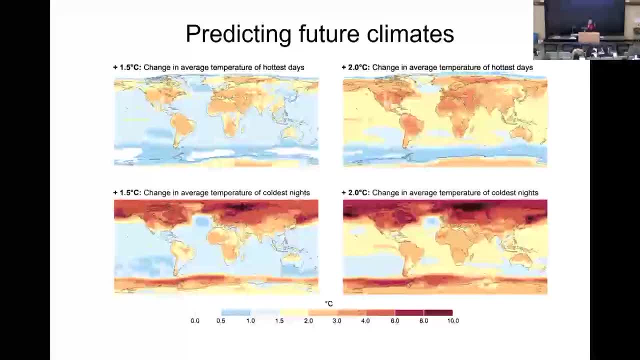 around the world? right, We've. you know. the scientists working in this space have progressed, you know, enormously. We're now at the point where we can run sophisticated models, come up with good predictions for future climates. And there was, you might have noticed, I think it was last week. 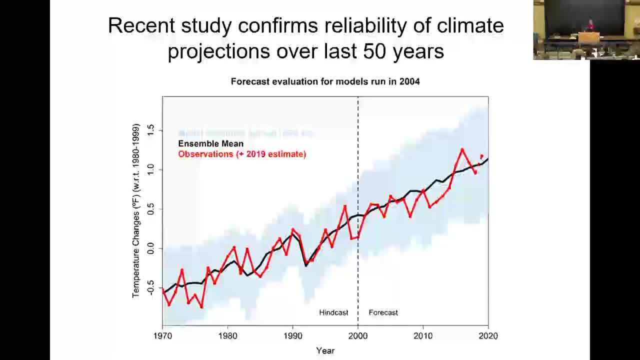 or the week before, there was a study that came out that was evaluating how well did all of those predictions really forecast climates, And it turns out really well. So even projections from you know, 50 years ago, you know, are actually tracking really well with what we're seeing today. 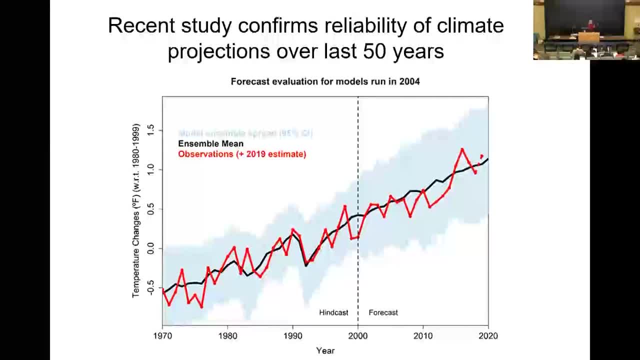 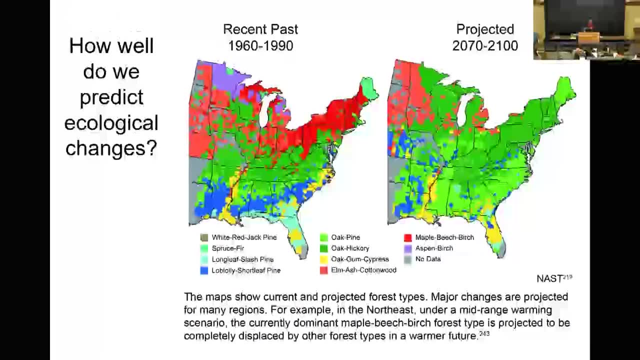 So, although we've really made all of this progress, you know, with looking at the climate predictions, we're still really challenged when it comes to understanding and predicting ecological changes. And so, for those of you who may not know, when we talk about ecology, you know we're talking. 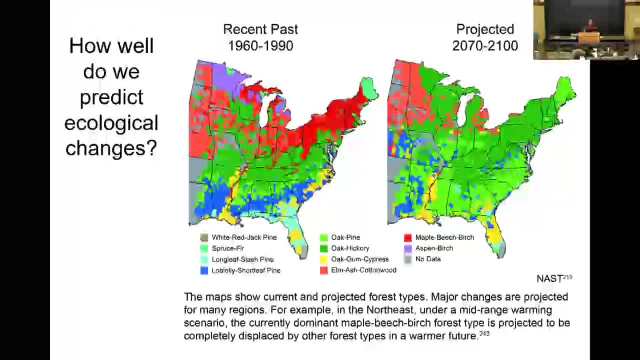 about not only the non-living components of systems, or what we'd call abiotic factors- temperature precipitation, you know- but we're talking about the living components as well, And so here in this slide, what you're looking at is some of the projections that have been made. 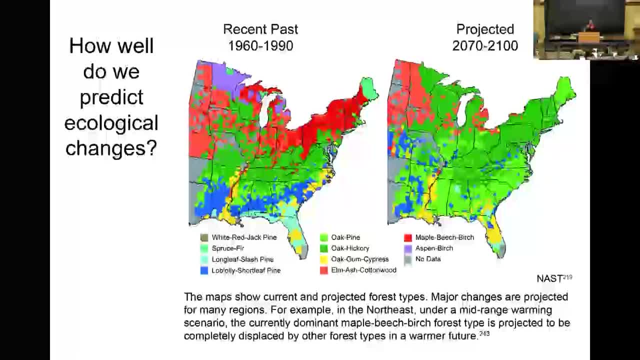 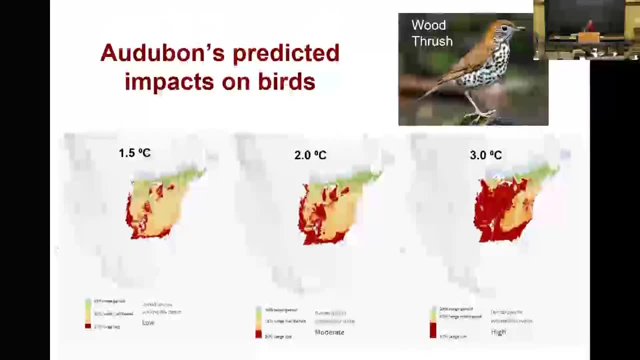 about how forest communities might change. you know how will they shift with changes in temperature and precipitation. We've also seen reports coming out increasingly that are forecasting how different animal species might respond to these changes in climate. This fall, Audubon National Audubon Society, released a prediction of how climate 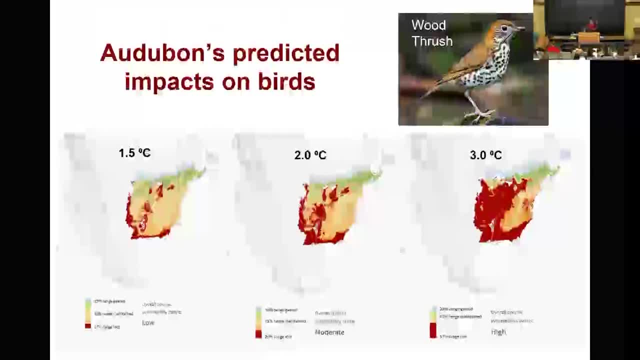 changes are going to impact different bird species, So here you're looking at one example. This is a wood brush. This is a songbird that breeds in the eastern US, And all the colored areas that you see indicate where the bird occurs today. But then where the red colors show where they're, 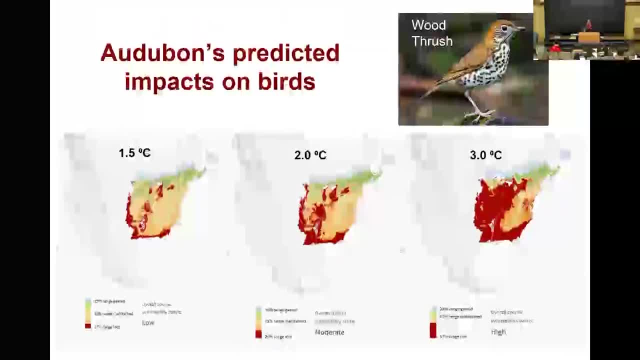 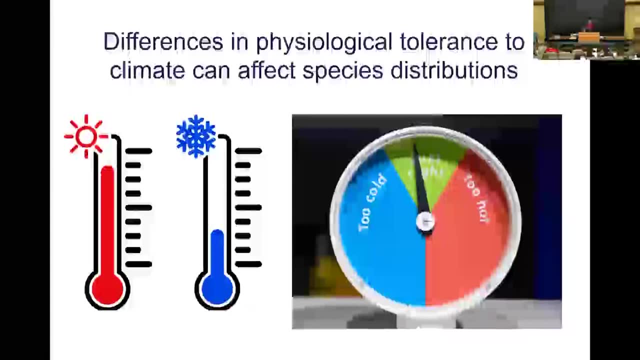 going to lose habitat. Habitats will become unsuitable for this species under different climate change scenarios. Now, how good? are these predictions right? It's true, certainly, that species are going to differ in how well they are able to tolerate different conditions, right? 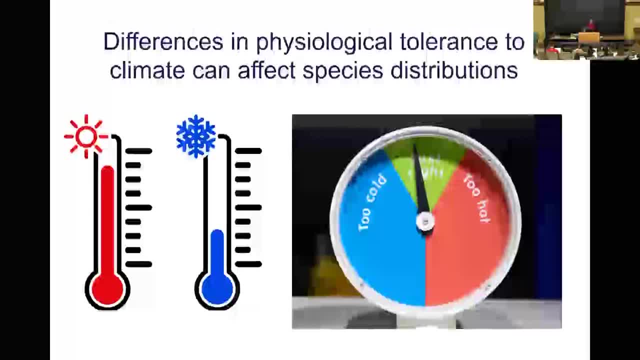 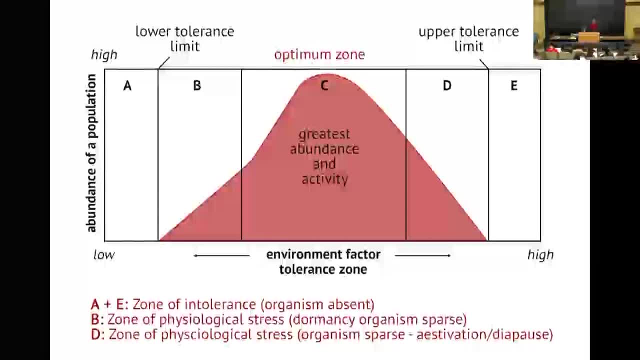 different climate conditions, different, you know, in terms of temperature and precipitation. We know that's the case And, in fact, if we could really think about that for any environmental variable, right, if you think about, you know whether it's temperature or precipitation. 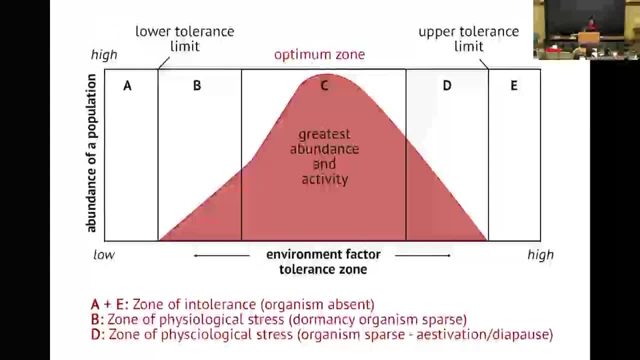 you know, whether you know it's certain kinds of nutrients that species need. you can think about any environmental factor being shown along the x-axis and the abundance of a species which is shown here on the y-axis or the vertical. you know, you will see that all species have an optimum range. 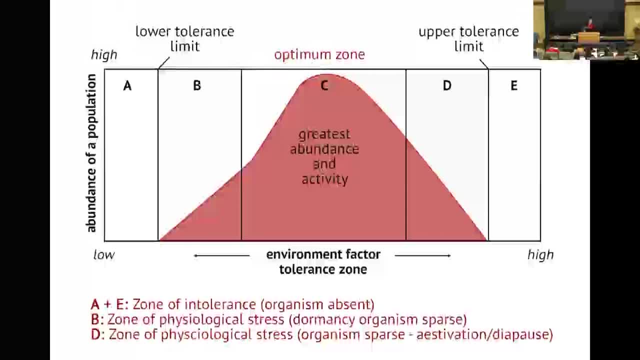 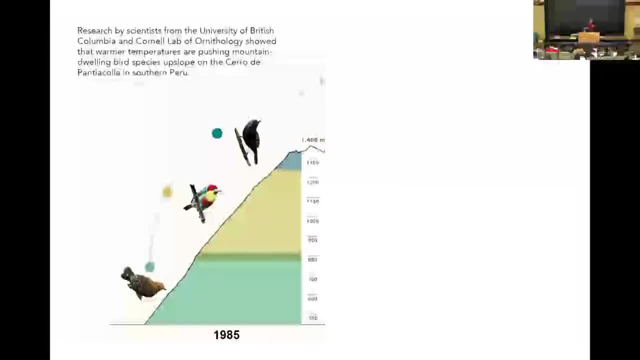 right of where they'll occur. right, It's pretty obvious. But and so too, just as one example, and we do see some patterns that really map on very well to how one would expect different species to respond To temperature changes. So, for example, there was a study that was published a couple of years ago. 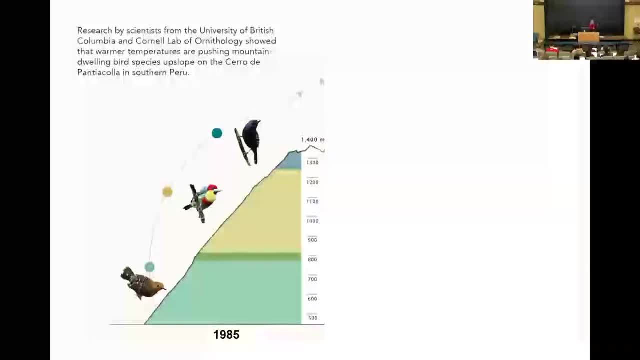 from the Lab of Ornithology. So back in 1985, John Fitzpatrick, who's the director of the lab, and colleagues you know went on an expedition in Peru and they documented where different species occurred along an elevational gradient right- And species tend to be. it's really 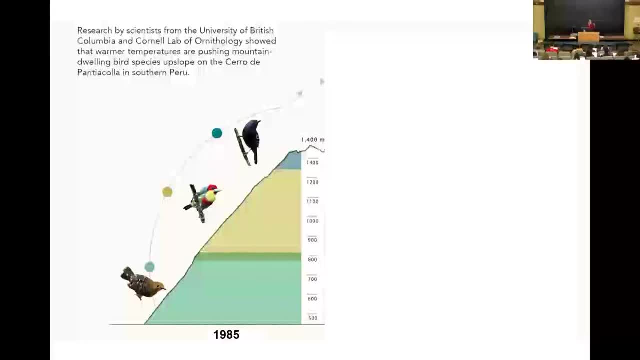 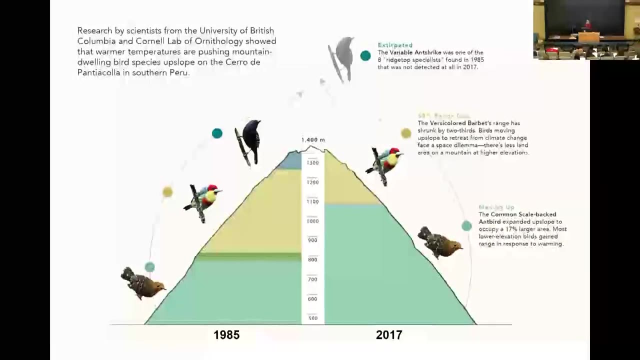 interesting. they can sometimes occur within pretty narrow and distinct elevations, And so in 1985, we'll just look at these three species here- This is how they were distributed along the elevation and mountains. But in 2017, when they went back to resurvey these sites, they found that 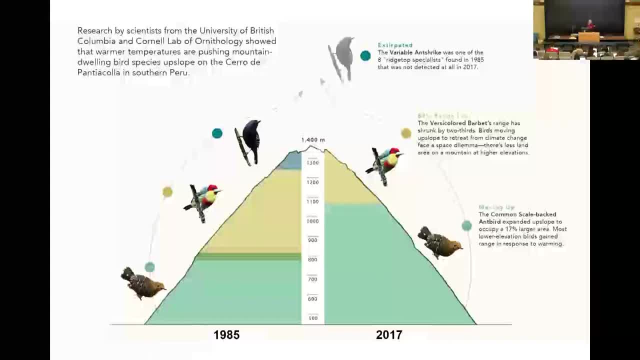 the species had shifted upward with warming temperatures. In fact, that shift upward resulted in the loss of one species. Now there just wasn't enough mountain to go higher in elevation to really track those cooler temperatures. So again, this, you know, this shows- and there are other examples as well- that, yeah, temperature changes or 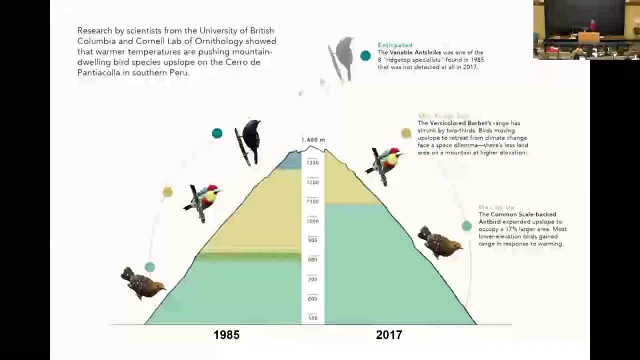 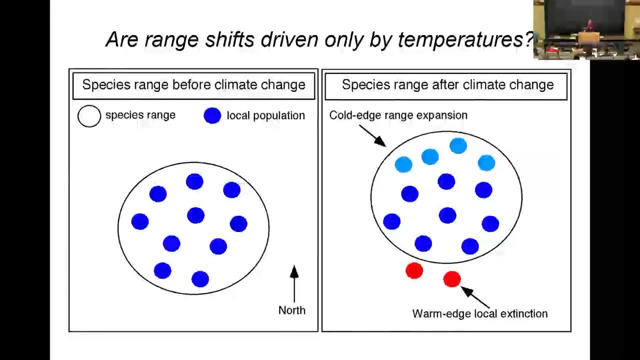 precipitation changes alone do have the potential to just drive changes that we see in distributions. But range shifts aren't always just defined by temperature, right, We don't see this scenario here where you can see with just all the blue dots you know here on the left, right. 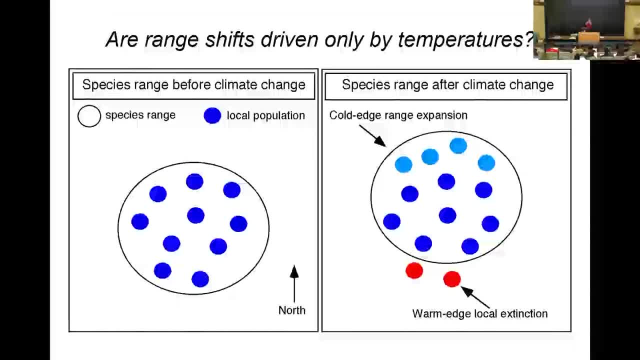 Here on the left, You have a species occurring within, let's say, their optimum zone And as the temperature warms, you'd expect, or they're going to shift to northward Right, And then range will expand into areas where it's cooler and contract where it's warmer. 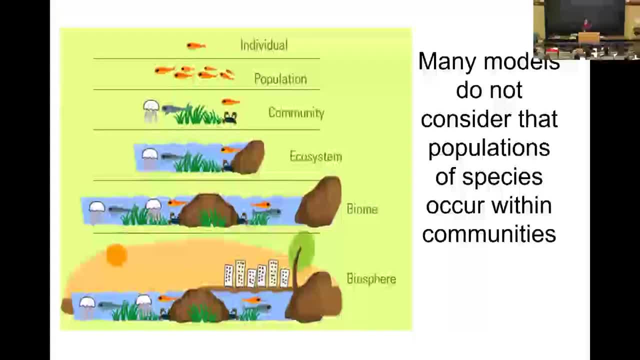 But we're not always going to see this kind of simple pattern, because the reality is that species don't occur sort of in a vacuum, Right, They occur within a community, Then the vegetation doesn't of other species, and so if you haven't been exposed to this, I'll just kind of 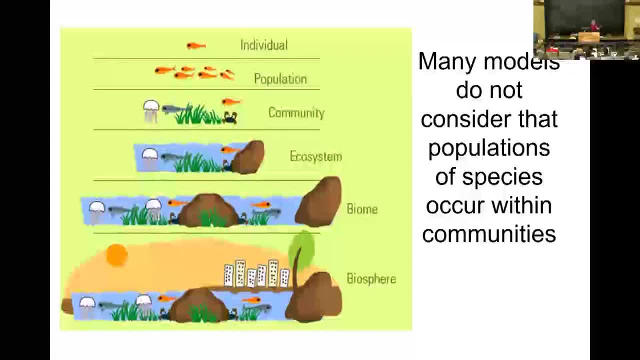 go through some of this terminology right. we can think of an individual, of a from a given species. when we talk about populations, that refers to a number of individuals of the same species within a defined area right for a community. in ecology, we're talking about something very different than people who are. 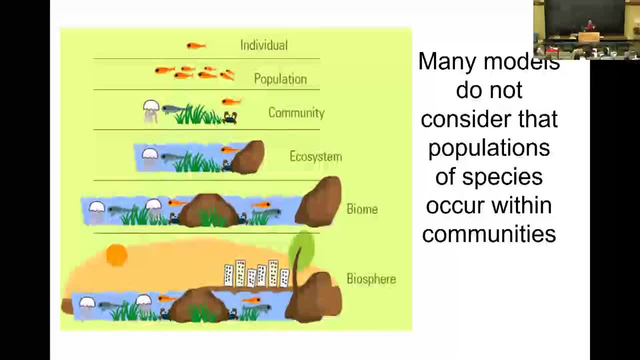 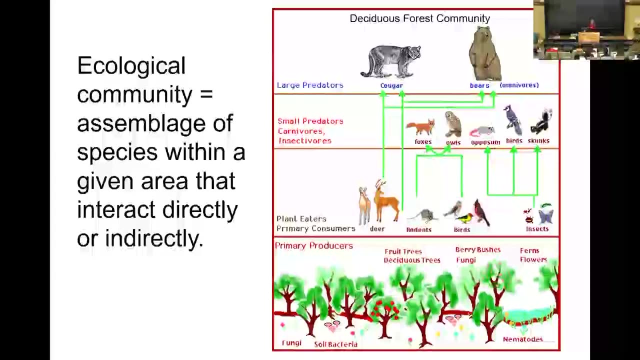 working in more of a social science context or political context might talk about. in ecology, a community means that it's a group of species that lived in a given area and they interact directly, sometimes or indirectly, and so one way to imagine this is like a food web. right here was there's an example of a food. 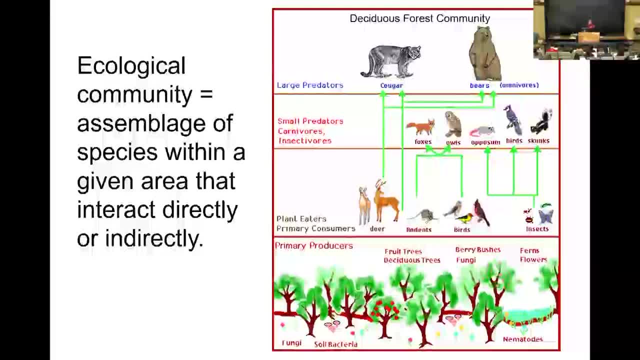 web from Eastern deciduous forests and all of these plants and animals, the fungi, you know, you know, you name it they're. they're all connected in some way again through direct interactions. maybe a predator eats a certain prey species or an herbivore eats a particular plant species, but their impacts on one another. 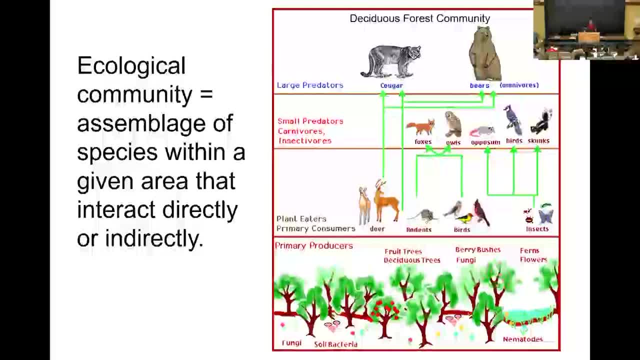 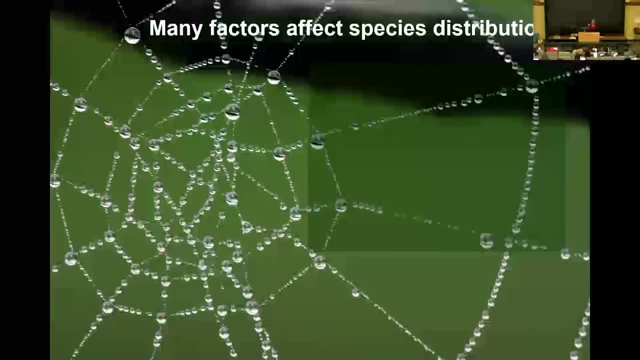 are going to kind of reverberate throughout that food web, and it turns out that there are lots of different factors that are going to determine how species are distributed. right, there are those physiological tolerances that we mentioned already, right, so their ability to tolerate certain kinds of condition: can they handle warm temperatures? do? 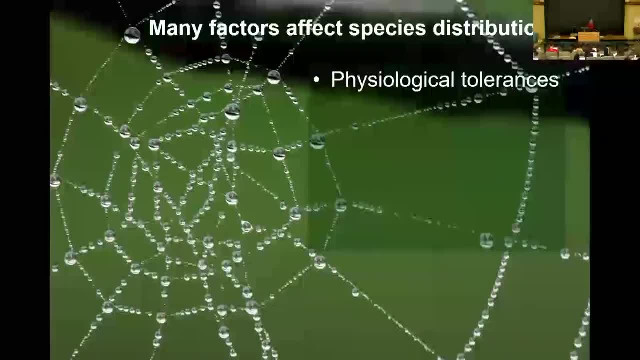 they need wet seasons, you know, can they. are they resistant to fire? moving through a system? you know, lots of different tolerances. there also habitat requirements. right, you're not going to get a desert species, that desert species that's able to, you know, really occur and shift its distribution into forests and 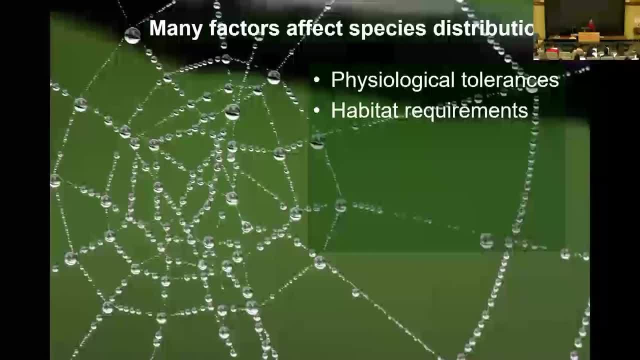 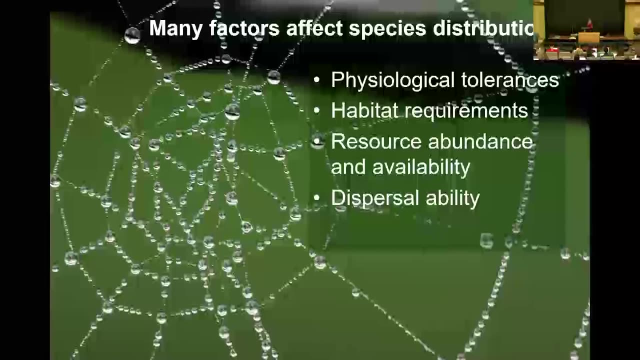 ecosystems, because it's just not going to find it. habitat requirements, the abundance or availability of resources, are also going to determine where a species can occur, as well as their dispersal abilities. so how well can they move right? so you can just imagine right trees that are already established in. 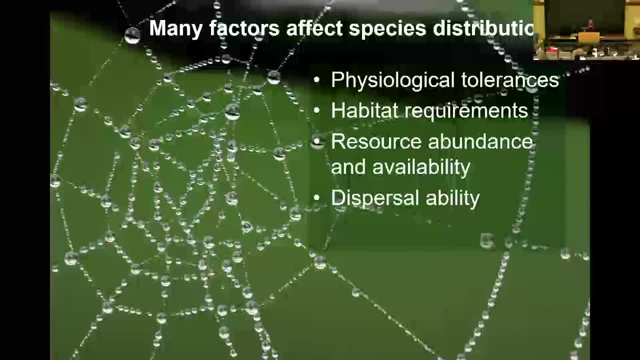 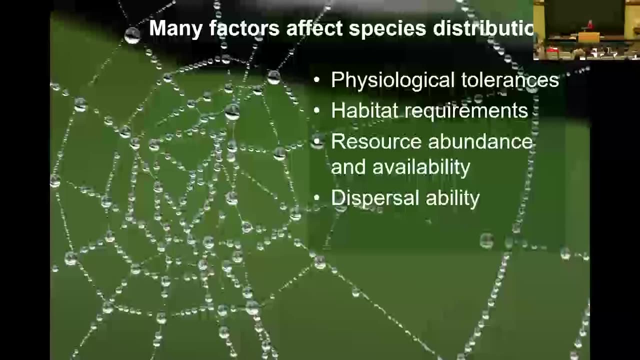 one location. you know they don't have the ability to move in in terms of the lifetime of that individual tree tree only by reproducing. But other species might actually have the ability to track changes in their environment in a much more quick time scale because they're actually able to move themselves. 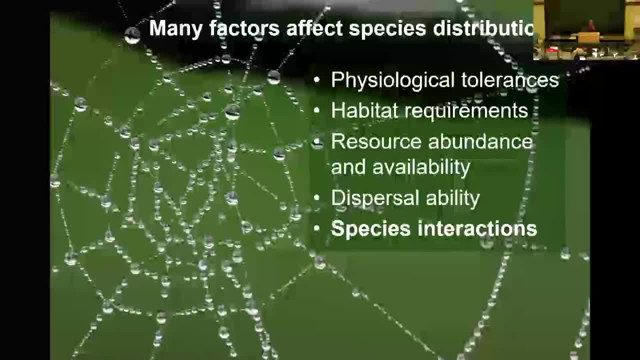 But what I want to focus on today for the rest of the talk is how species interactions can actually play out in ways that can affect or somehow modify the way species are able to respond to climate change, And I chose this spider web just to provide a, you know, sort of this visual metaphor. 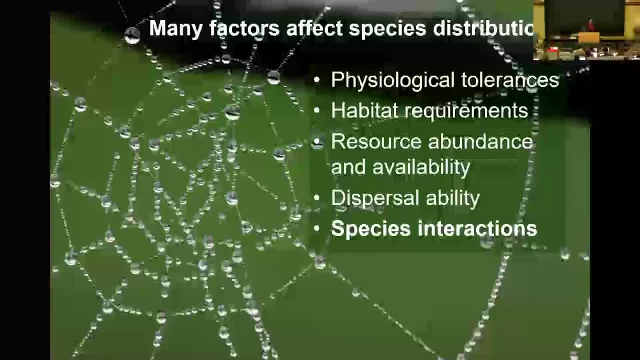 of what a community really is right And how. if we're pulling on, tugging on one of those little web links- you know one of those strands- we're also going to be affecting other ones as well. So that's a good way to think of communities, right? So as temperature might be causing shifts. 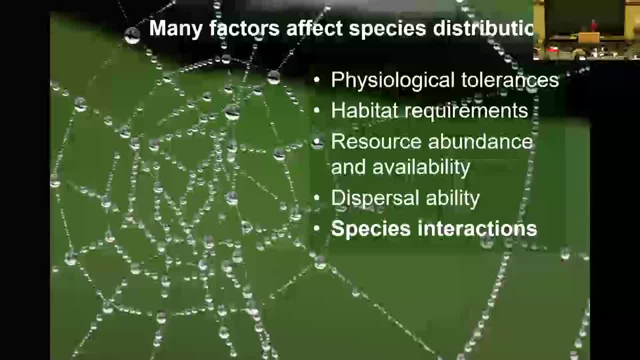 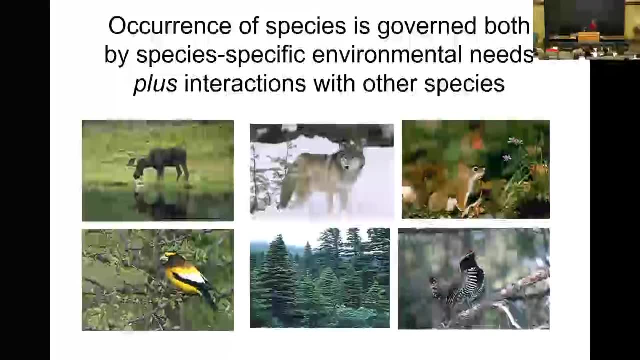 in some species, that's going to cause, you know, effects to others as well, And so, again, the really important point here, which really is the take home message in some ways, is that the occurrence of any given species is going to be determined both by its own needs. 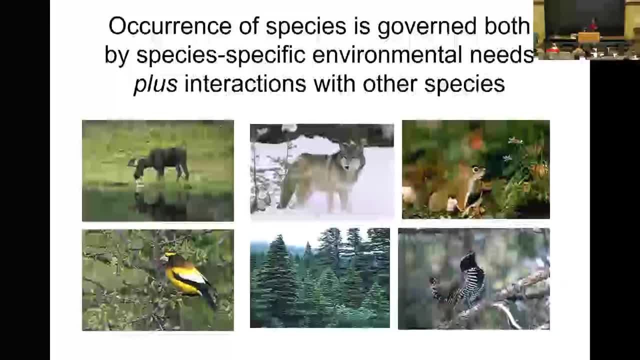 sort of, you know, related to the environment or the resources it requires, but also because of its interactions with other species. Right, Just think of a predator: can't occur in a location if it's not a predator, And so you know. I think that's a good way to think of it. 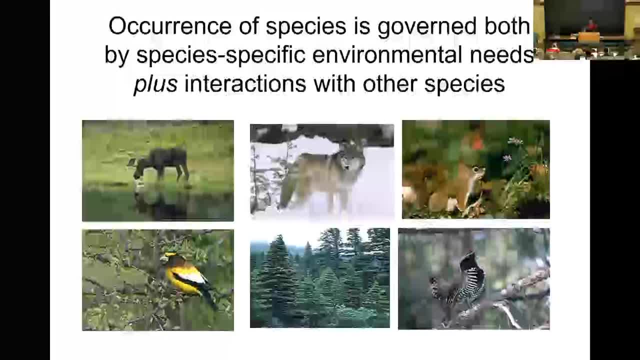 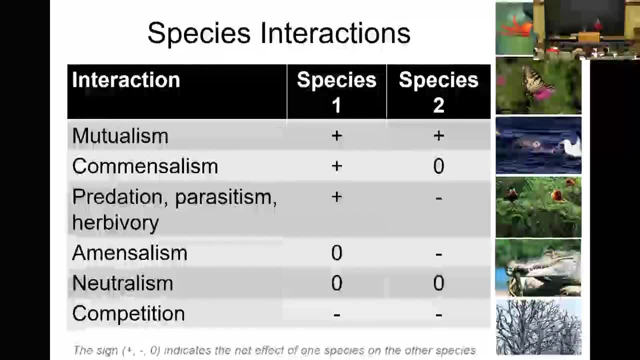 It's prey items aren't there, right? That's the sort of thing I'm talking about here. So, for species interactions, there are a number of different ways that species can interact, And so we'll talk about these just really briefly, And so what I've done is I've put this in a table. 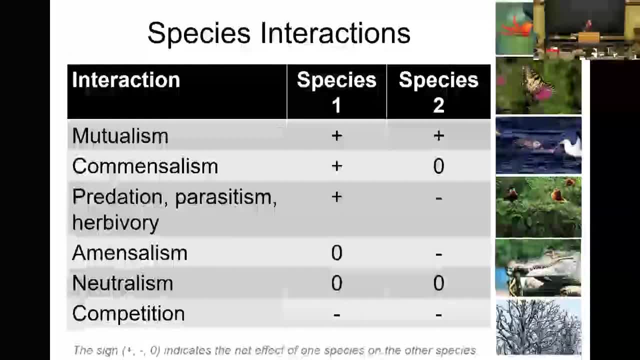 where there's the interaction type, and then we have two hypothetical species next to each other: species one, species two, And whether it's a plus sign. a plus sign indicates that species can interact with each other, And so we'll talk about these just really briefly. 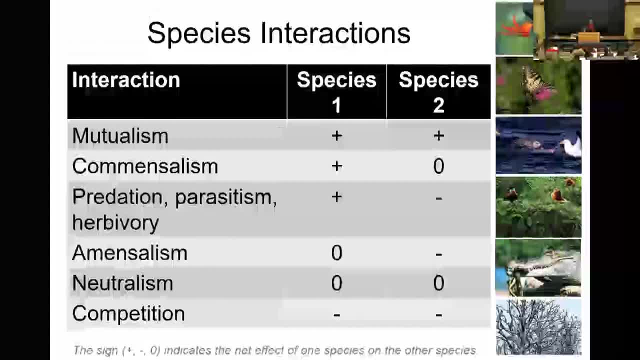 The species benefits from that interaction. A minus sign means the species does not- it's actually harmed in some way by that interaction, And a zero is that it's unaffected. Okay, so for a mutualism. this is a kind of interaction where both species benefit, And so some examples of this are like a: 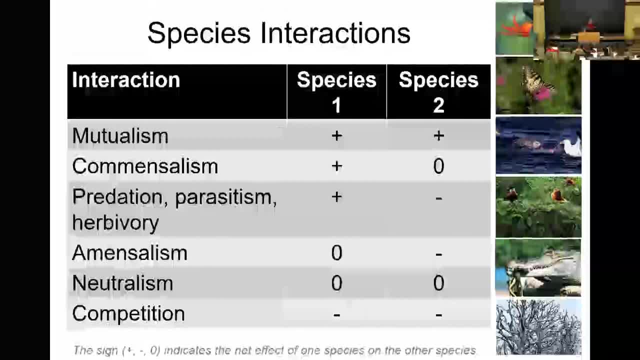 plant and a pollinator right. The pollinator is getting food resources. the plant is getting you know its dispersal, It's able to actually move its genetic materials. Another one would be seed dispersal right. Similar kind of interaction. Commensalism is a little bit more one-sided. Okay, there we have. 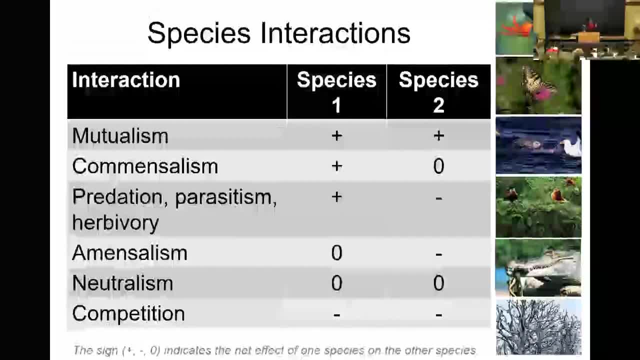 one species benefits, but the other is not effective at all, And so some examples could be: where you have sharks, you know sharks are predators in the ocean, You know if they get a prey species and you know there's the kill, there's lots of little. 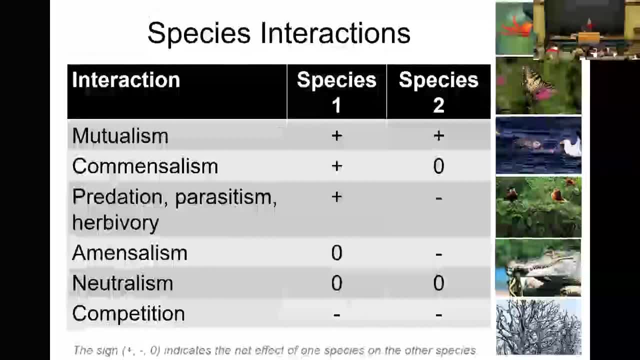 bits of flesh that are floating in the in the water, after you know they consume what they need, And it's not uncommon to see other small fish or birds- you know gulls- coming in to eat those scraps. The sharks don't care, They already got what they needed. They're not. they're not. 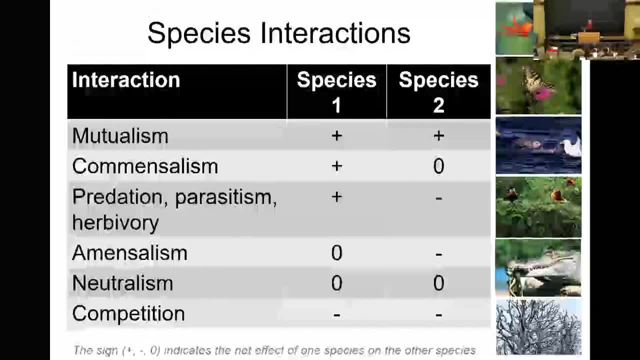 affected at all by what's happening after the fact, But those, those birds and other fish, they're actually benefiting from that interaction with the shark. Another example would be where I work in in a lot of tropical forests, So you'll have monkey troops moving through the forest. 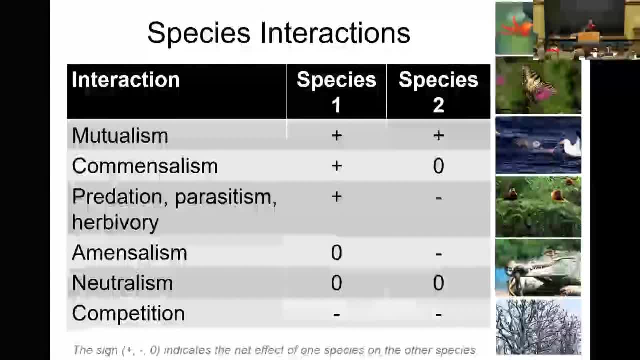 canopy and they're, as they move through, you know, the vegetation's moving and stirring up insects And there are birds that will follow them through the canopy and eat the insects that are flushed. There are also birds that follow along the floor of the forest and eat the fruits. 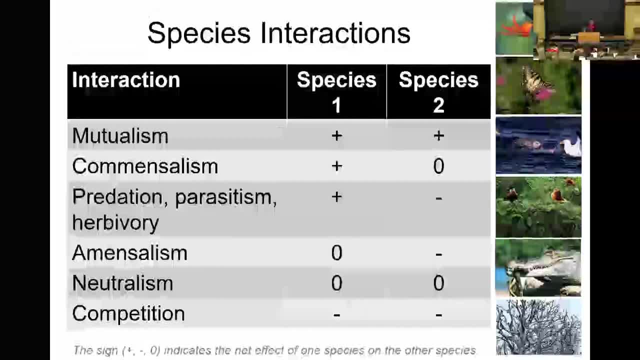 that are dropped, The monkeys don't care, but those other species benefit. That's a commensalism. Interactions can be also very oppositional, right, If we think about predation or parasitism or a bivory. clearly one species is benefiting, right, The one that's doing the eating and the 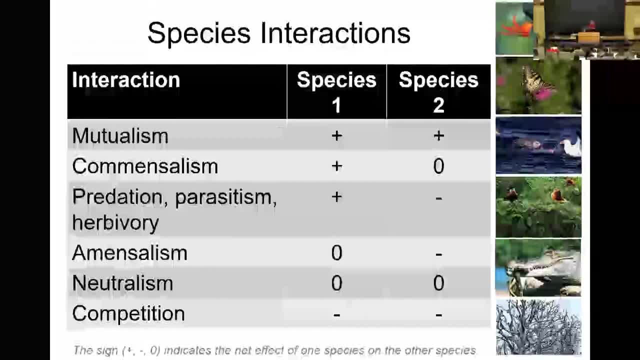 other one is not so much benefiting. right Amensalism is where you have one species that's negatively affected and the other is unaffected. This might be, you know, examples of this are a lot fewer and far between to demonstrate, but this would be where there might be, let's say, maybe a chemical or, some way, one species. 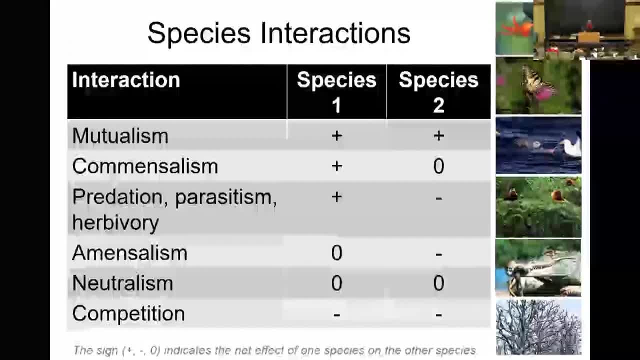 changes the environment that is negatively affecting, you know, some other member of that community. And then neutralism. you know two species pass in the night and very right, no interaction. but we got to put that up there just to be well-read. 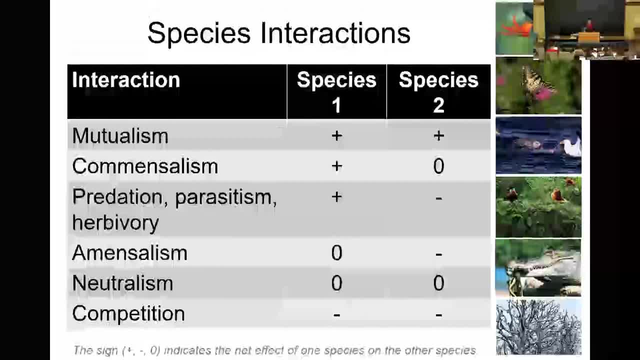 And then finally competition. This is where two, both species, are negatively affected. A lot of times it's funny from a human lens. we tend to think about competition as well. one win and the other loses. But in fact competition both lose relative to if there. 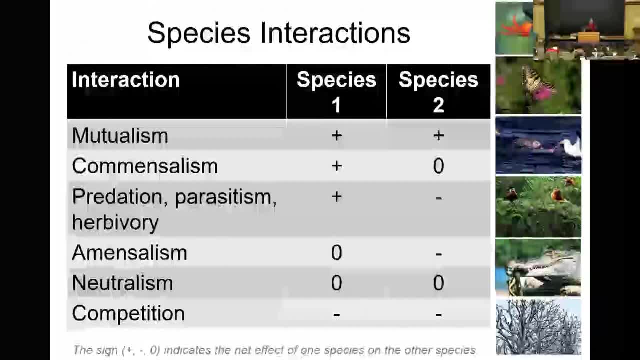 wasn't that competitive interaction in the first place? because even the quote winner is actually spending energy. you know, in that competitive struggle Or isn't getting as much, you know of the resource there would be without that, competitor species there. So when I talk about species interactions you know really there's an 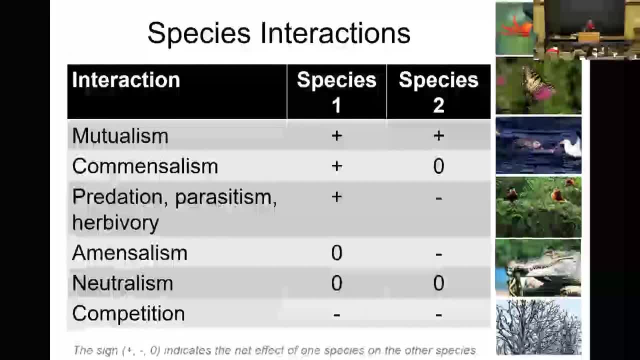 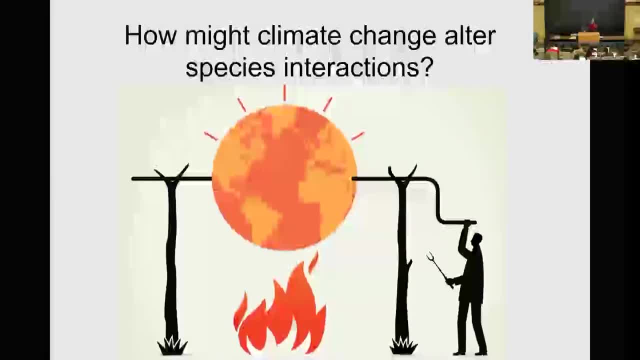 enormous gamut of ways that species are able to interact with one another. So, moving forward, we'll be talking about different examples and ways that those species interactions might be affected by climate change and in ways that can have profound consequences for the environment. So I'm going to start with the first one, which is the 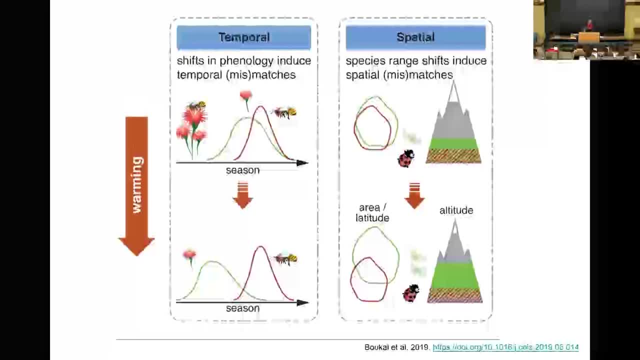 effects of climate change on the environment. And then I'll go back to what I was talking about earlier, which is the effects of climate change on the environment for ecological communities, Two of the ways we can think of this. I guess that people often describe how interactions 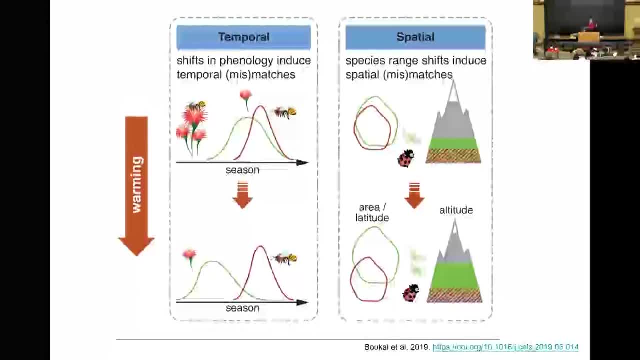 can be affected are in terms of how climate change might be affecting sort of temporal scale or time scale on which they interact. So you might have heard about mismatches in timing. This is what they're talking about here. So let's say you know if you're not sure about climate. 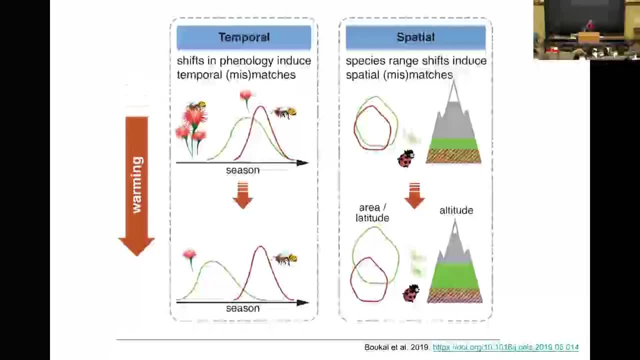 and you have a sequence. two species tend to interact at the same time each year, but when temperatures warm, activity is shifted for one species but not the other. That's gonna be a mismatch. You can also have a mismatch in terms of the spatial extent as well, right? 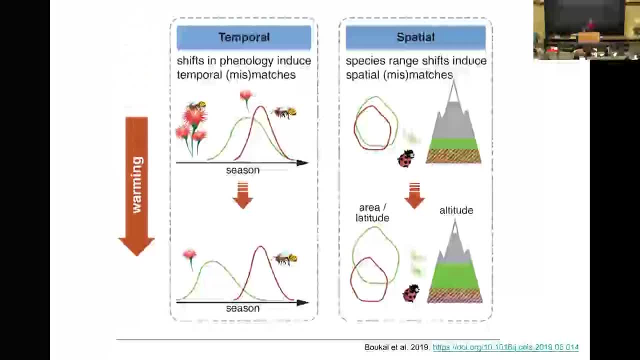 If we go back to that example of birds moving up slope on mountains as temperatures warm, well, if one of those species is moving up slope, but let's say, another one doesn't have the capacity to move, now there's a spatial mismatch, right? 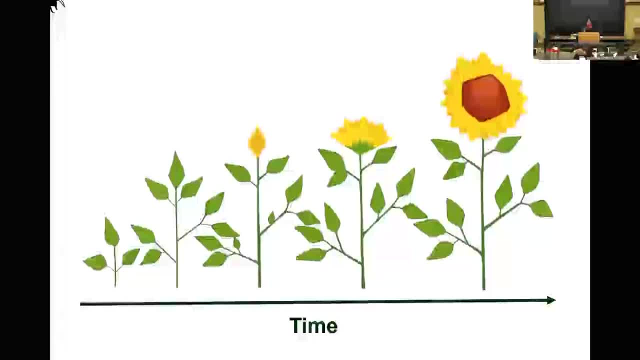 They're occurring in different areas. We can have some examples of these. So if we think about like with a flowering plant across the season, right, It progresses in a series of stages and pollinators have evolved to have the right timing. So a bee's gonna come and it's ready to pollinate the flower. 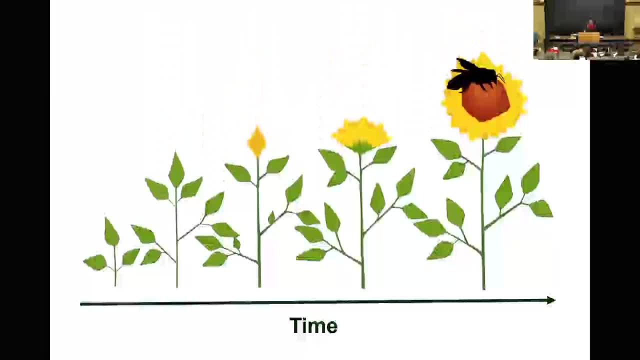 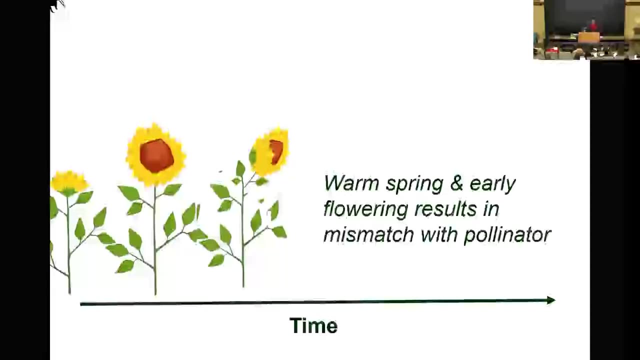 Its activity matches when that flower is ready to be pollinated. But we can imagine that if the temperatures were to shift or to warm such that now that flower is really blooming much earlier in the season, but if the pollinator hasn't changed its activity patterns, 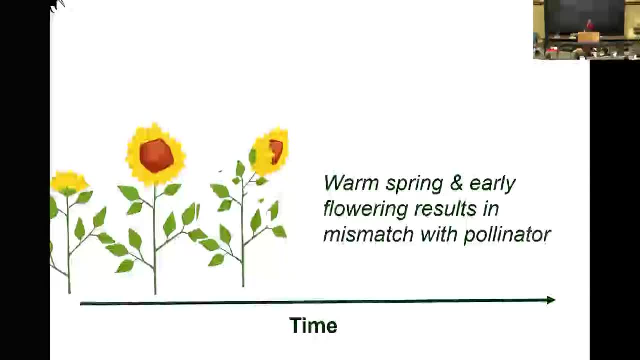 and because maybe it has a certain period of dormancy that it's locked into kind of every year, then it might be that it loses out right, They're mismatched from a temporal perspective And we see evidence of this really from a number of studies. 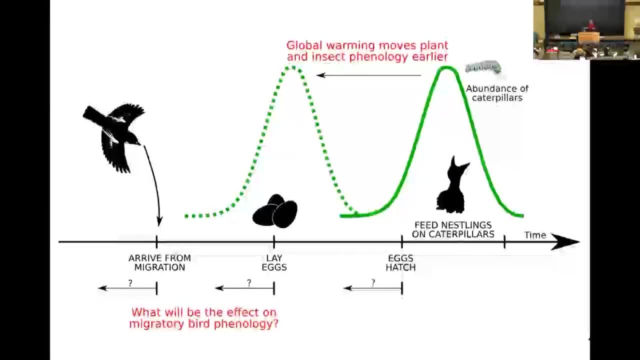 So you can take some of these examples with birds. So with migratory birds, there are different ways or different types of migrants. Some migrating birds only migrate short distances, like American Robin right that you might see during the warmer times of the year when it gets super cold. 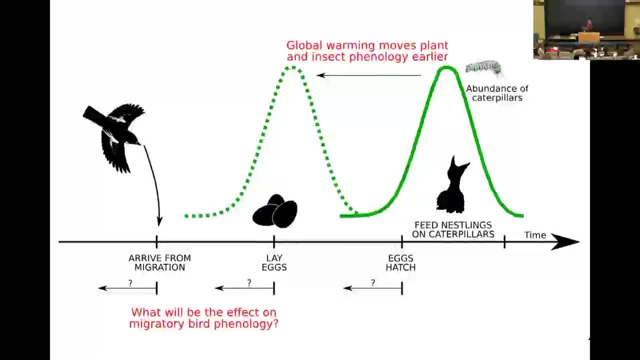 you know it's going to be really, really cold, right, don't really notice it as much. It's able to kind of move with the temperatures because it's not moving large distances. But for our migratory birds that leave the US, you know that winter 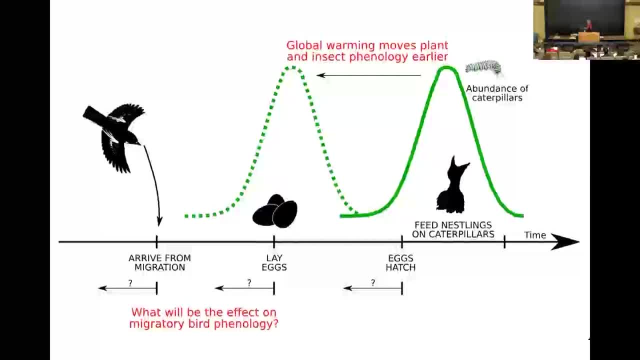 in Central America, South America and the Caribbean. they're far away, right. They don't know what the temperature is up here, So they don't have the ability to just respond. I mean, this would go true for migrants in. you know the old world as well, And so instead a lot of. 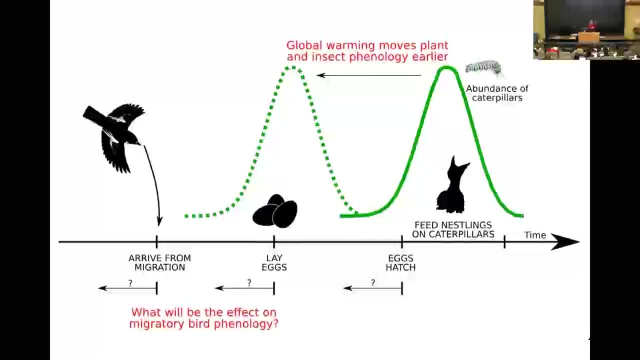 these migratory birds are using other cues, like the day length, in order to know when to migrate, or you know other cues from the environment that aren't related to temperature up here, And so there is this pattern now that we're seeing. is that a lot of the migrating birds? 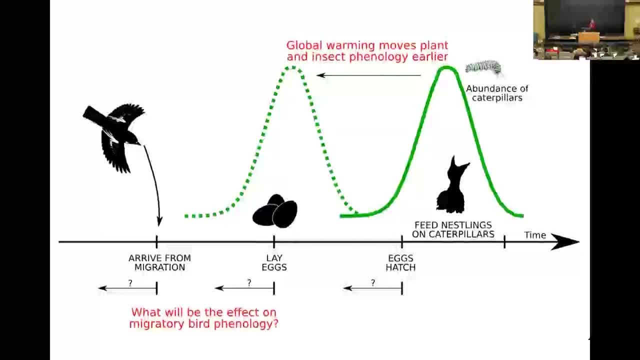 long-distance migrants, although we're seeing some shifts with earlier migratory birds, we're seeing some shifts with older migratory birds. we're seeing some shifts with older migratory birds. we're seeing some shifts with older migratory birds breeding season, they really don't have haven't yet shown the capacity to massively change. 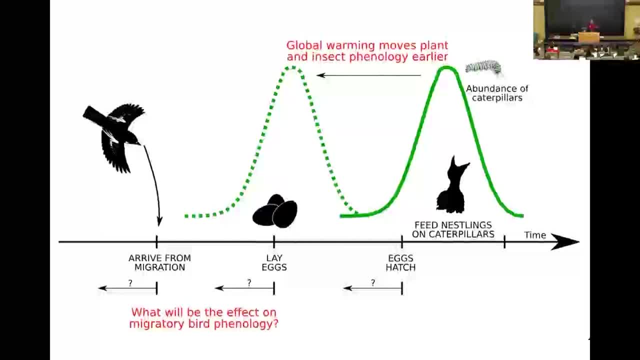 when they initiate breeding, But a lot of insects that they're feeding on, you know, and feeding their young with those, because they're here- do have greater capacity to shift and to advance, And so what we see is this mismatch in terms of when birds come back, they build their nests. 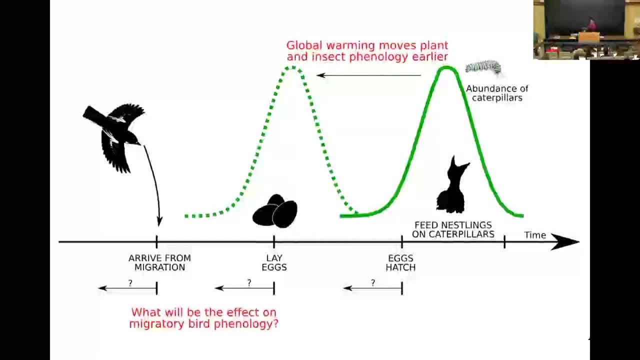 they lay their eggs, The young hatch, they're ready to feed them. It's a time of enormous demands energetically. but dang, the insects already you know hatched and their big population boom already happened. So there's that impact And they've shown that there are cases of these that have population. 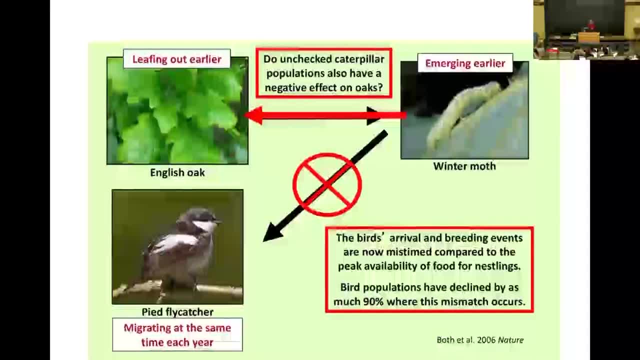 level consequences for the species we're talking about. So in Europe, the pied flycatcher is one that they've shown. It's still, you know, it's still, you know, it's still, you know, it's still. 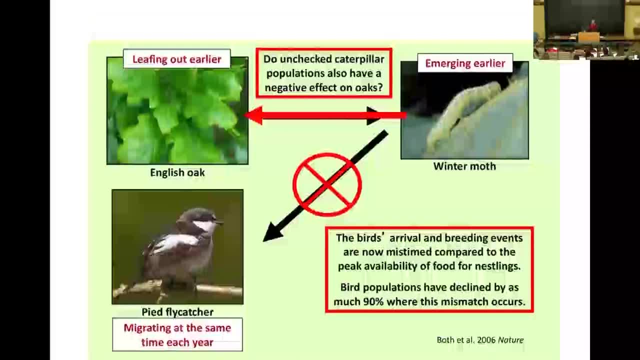 it's migratory patterns are more or less the same every year, but the caterpillars that they feed on are emerging much earlier, And so what happens is that that the food or the resources they require, you know, don't occur now, when they most need them, And that's resulting in this population decline. 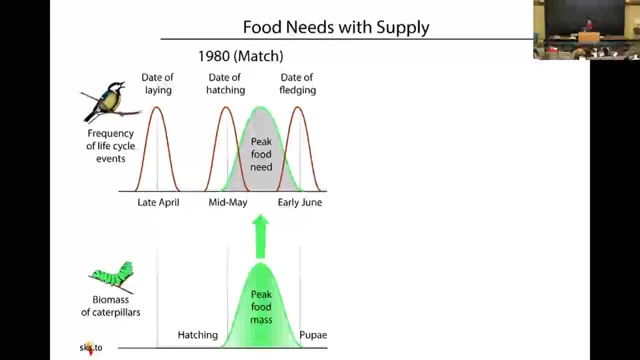 in that species. They've, you know, shown similar kinds of cases for some of the resident birds or species that stay in an area year round, even though they have more ability to change when they're nesting. So here this is, from you know, a graphic showing in 1980,. 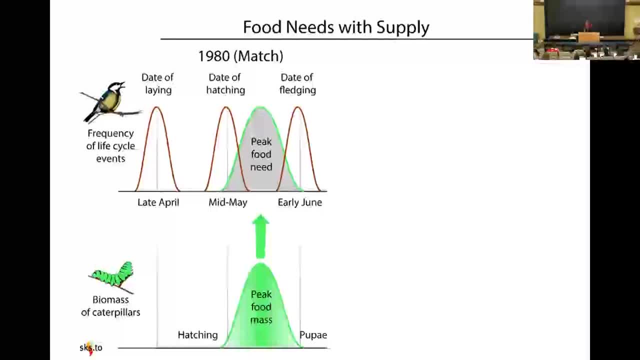 this species in Europe, the great tit, when it was, you know when it typically would lay its eggs, when its young would hatch in mid-May, And then you can see with the green line, when the young hatch, the peak abundance, peak food need, I guess, came, happens right. So right after the 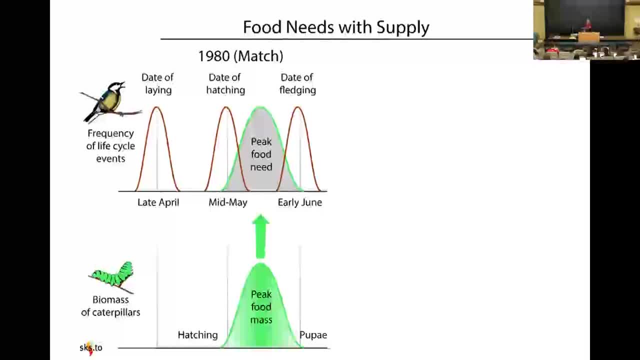 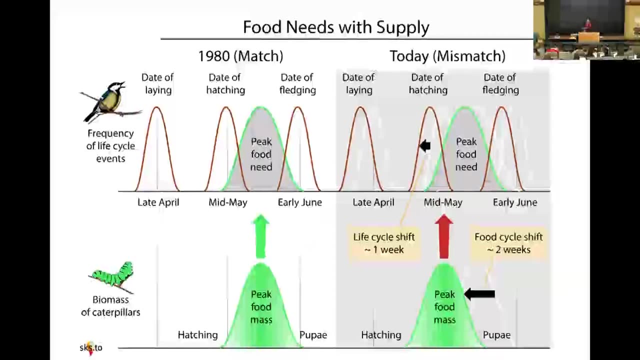 young hatch. that's when the young are begging And that's, historically, when you would have the greatest biomass of caterpillars available, right? These species have evolved in this, in this system, But now what we find is that there is a mismatch, Even though those birds have shifted to laying. 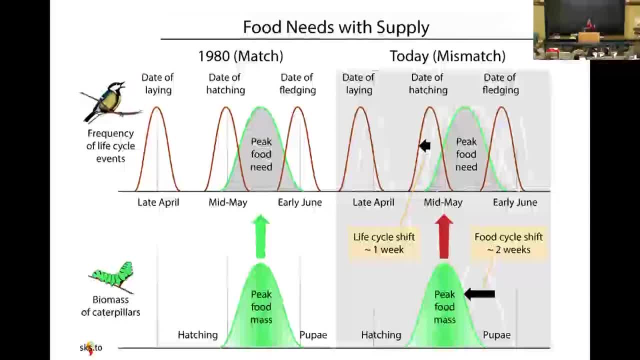 eggs earlier in the season. their young hatches are still, you know, they're still, you know, their young hatch earlier in the season. they're not advancing as quickly as the insects are, as those caterpillars are right, And so there's still that mismatch with food. 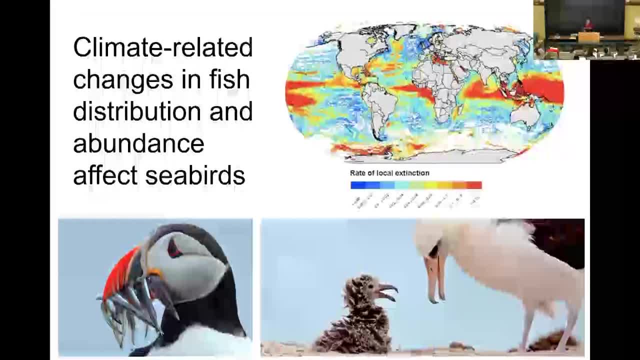 And we can see this across different species as well. right, So seabirds are another group that's really being impacted by climate change, among many other threats that they face, right In terms of the distribution of fish and the abundance of forage fish. you know those are very sensitive. 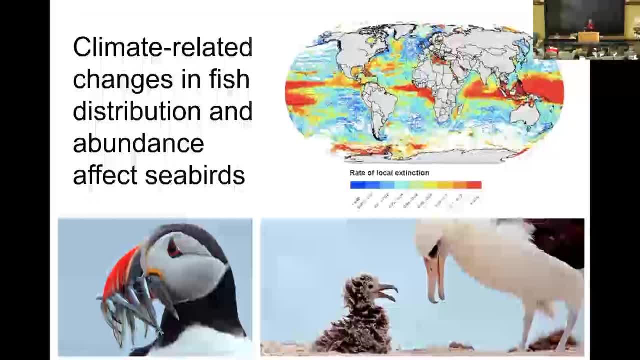 to changes in temperature and other elements of ocean productivity that are related to temperature, And so we find now that there are sometimes some years where seabirds have complete reproductive failures because they can't have access to the food resources that they need for their own. 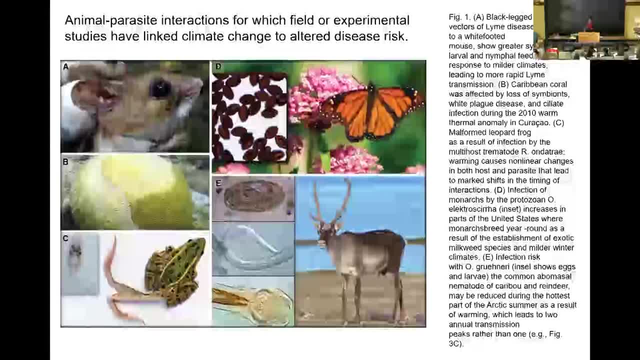 survival and the survival of their young. Some other places where there's been a lot of growing evidence for how climate change can affect the survival of the young is in the United States, And so there's a lot of evidence for how climate change can impact species interactions. 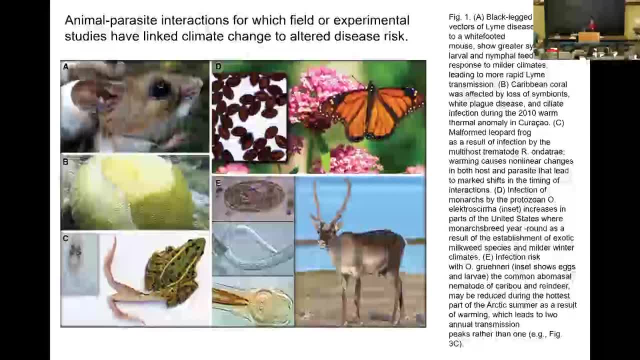 or in the realm of disease and wildlife disease, and in terms of, and especially with parasites. So again there's when you think of the life cycle of parasites, the life cycle of animals. as we start shifting climates, sometimes that can exacerbate the disease risk or, in other cases, 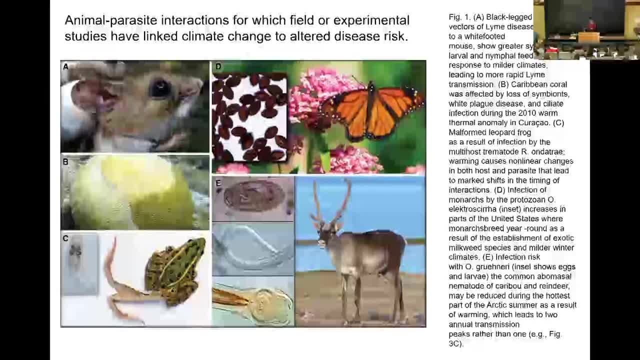 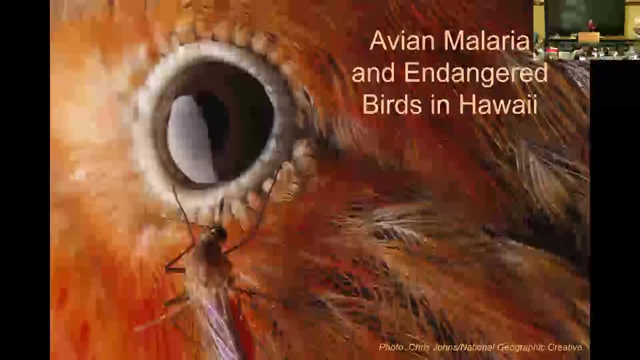 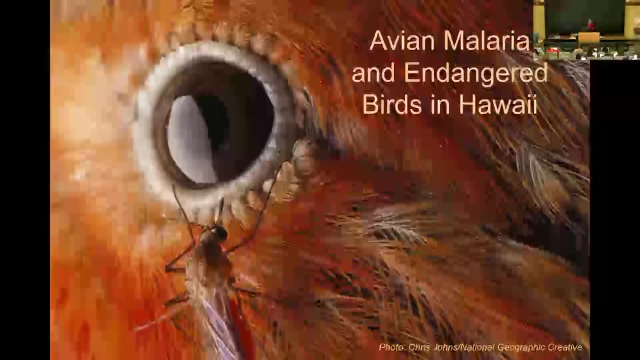 maybe dampen it a bit, And there have been examples again across many different kinds of animals and other species. I'll give you one really interesting example. that's a serious conservation problem right now in Hawaii. So in Hawaii one of the challenges that they face is that avian malaria was introduced. 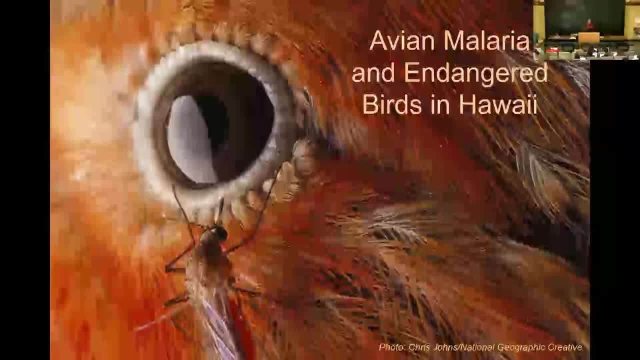 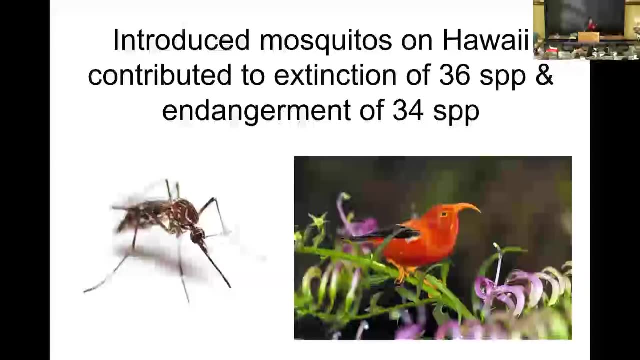 you know back a couple hundred years ago with mosquitoes. So Hawaii did not have native mosquitoes, but they were introduced and brought malaria with them, And so you can much like with any species when you have a naive population. they don't have defenses for a. 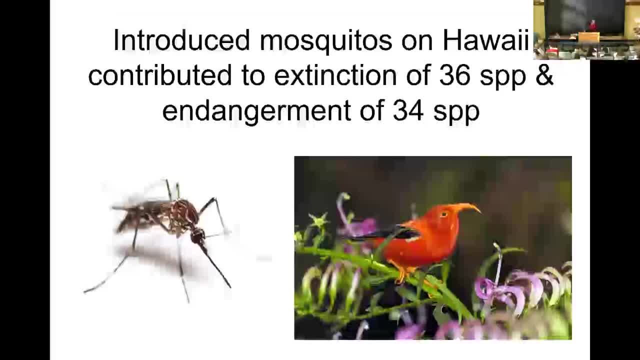 particular disease. they're very vulnerable, And so Hawaiian birds ended up being that incredibly vulnerable to malaria, And so it's thought that introduced mosquitoes contributed to the extinction of 36 species of Hawaiian birds. right, There's a lot of endemic or species that 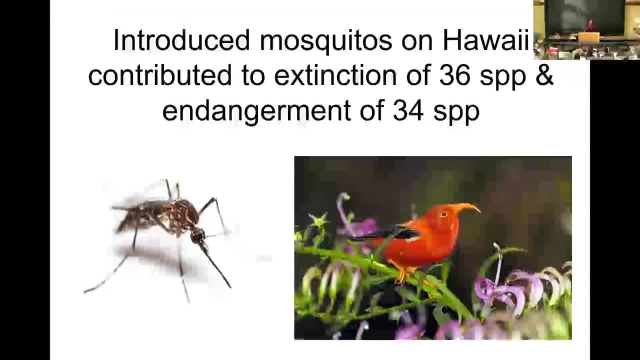 occur only like on islands, And so it's thought that introduced mosquitoes contributed to the extinction of islands. nowhere else that we've used endemic to describe them. So we have extinction of 36 species, but there are 34 more species that are currently endangered, critically endangered. 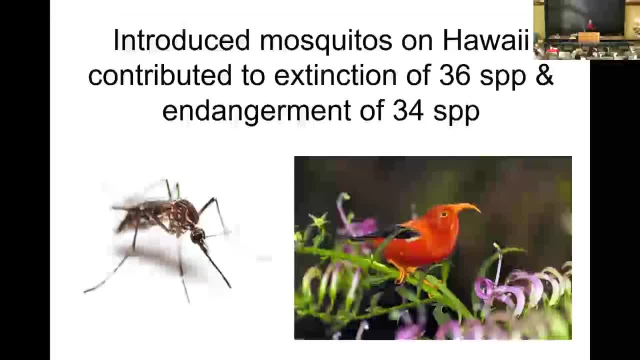 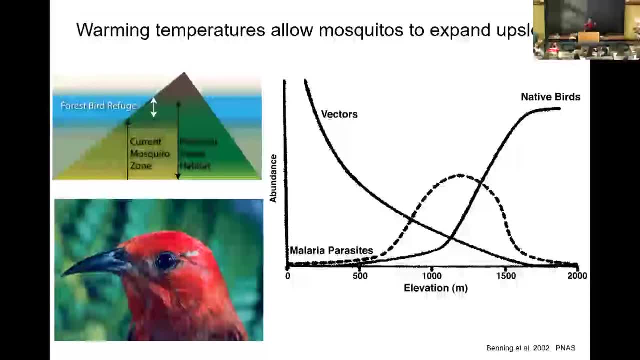 in a large part due to avian malaria, And so what's interesting is that when you look at them, these populations, they only persist in high elevations, right. So Hawaii has a lot to mount and these volcanoes. you have forests along all of these slopes, but mosquitoes are temperature. 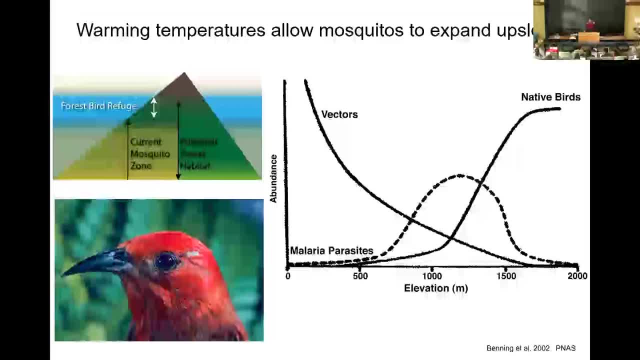 limited there, So they only occur at those sort of lower elevations, lower and mid elevations, And so that provided this kind of disease refuge for a lot of the Hawaiian endangered bird species, And you can see that here on the graphic as well. 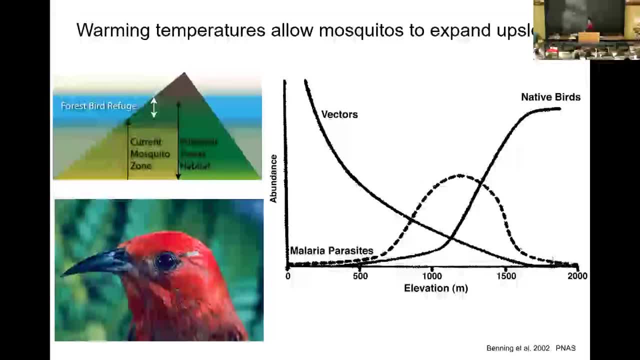 where it's. you know, as you move up in elevation you can see the malaria. right, It's at these mid elevations and then the native birds are up here at the highest elevations. But as climates are warming, as the temperatures increase, now mosquitoes are able to. 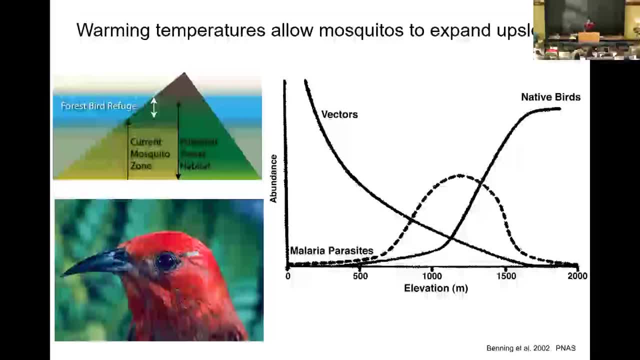 move farther up slope And people are worried that these Hawaiian birds are going to completely run out of the refuge, out of their refuge from the disease. What might be? if you're interested in this, there are some folks in the vet college that are actually working on this now. a new postdoctoral 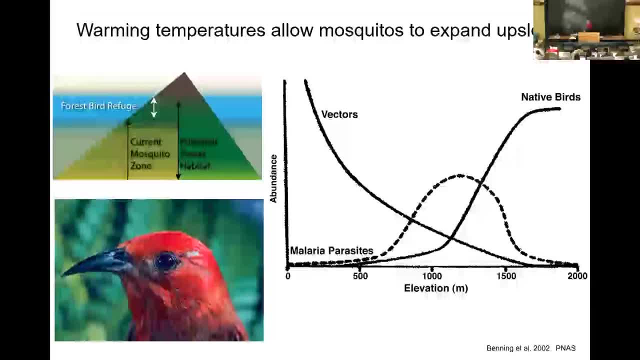 researchers working with collaborators. I just heard a talk last week and they're trying to come up with ways to modify the mosquitoes, you know by inoculating them with a different virus or bacterium. you know, in a way that they're trying to tackle the problem in that. from that, 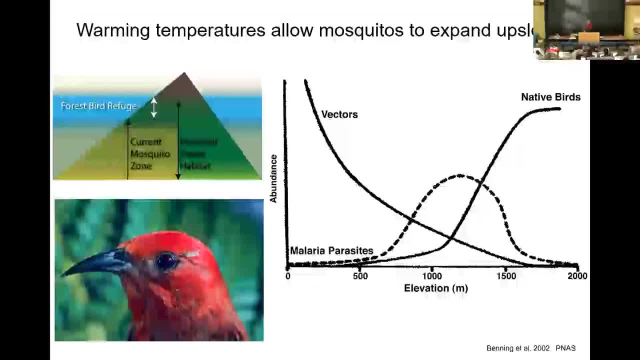 sort of perspective. But again, this is here fundamentally right: this disease, this parasite, it's an interaction right with its host that is being affected by the temperatures right, And you can imagine, for a lot of these bird species they've also evolved to be important pollinators. 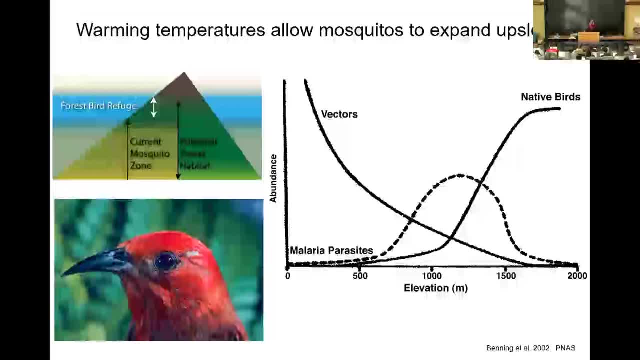 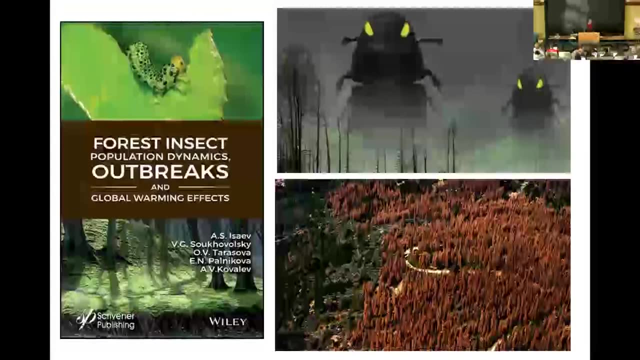 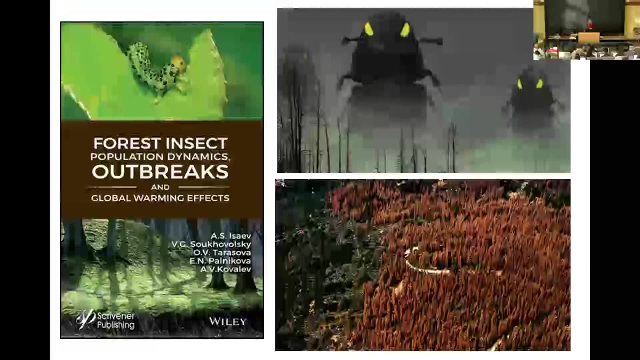 or seed dispersers of plants. If we lose them because warming temperatures now allow mosquitoes to invade their refuge, we are also likely to see consequences for other species in that community as well, And similar. in a similar vein, right outbreaks, pest outbreaks, are another interaction you know that is likely to be affected by climate change. 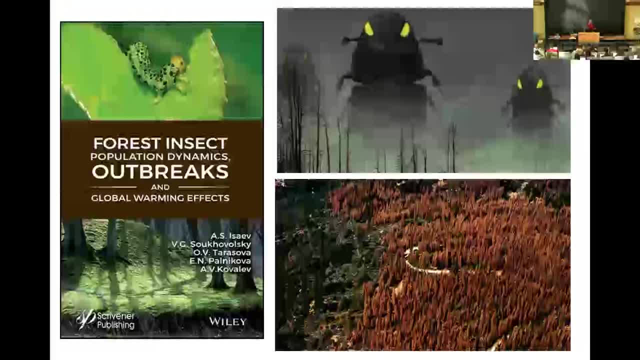 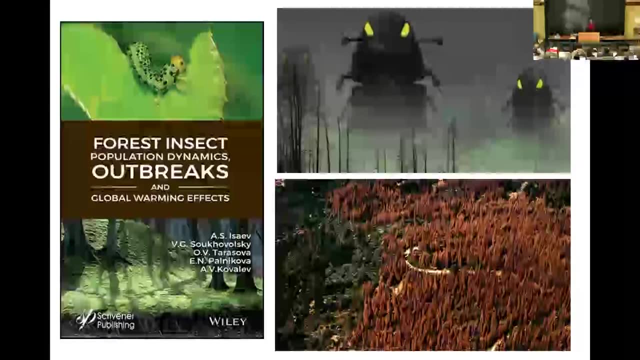 And we're already seeing evidence of that. You might have heard of some pests in forests, like the pine bark beetles, that they can be eruptive in terms of their outbreaks and can cause enormous- you know- mortality of trees in certain areas. 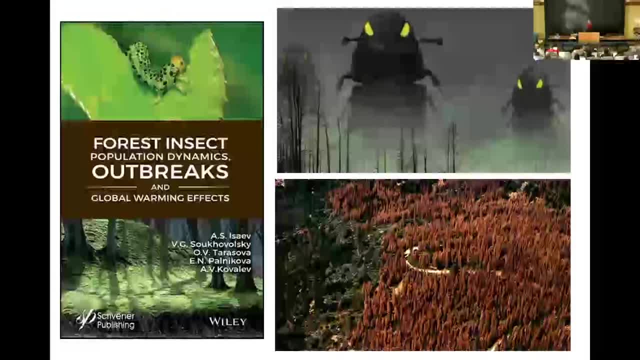 Now these insects are native in many cases. you know for native insects, you know they've evolved in that system, But when we start changing, you know the, the temperature, the levels of precipitation that can stress trees out more, so they're more vulnerable to being killed when there is an outbreak of the pest. 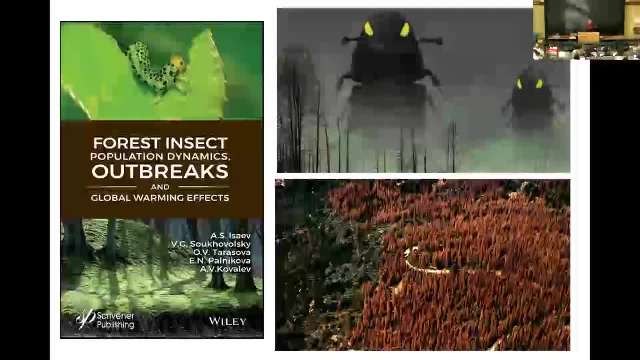 And it also it facilitates greater numbers of those pests because they're not dying over winter right. Usually those cold temperatures might knock back the insect populations a bit every year, so the outbreaks aren't as bad. So we are seeing much more extensive outbreaks. 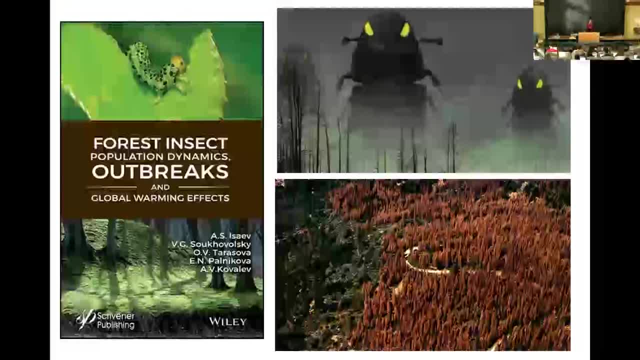 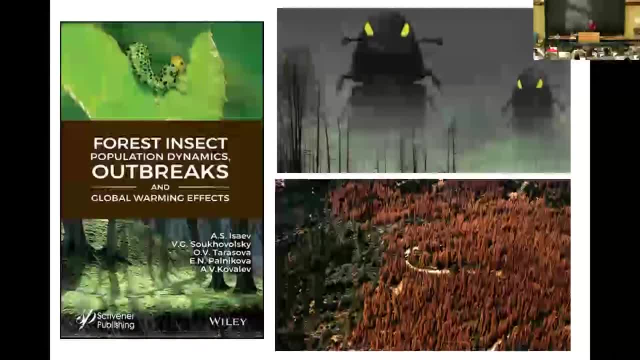 And, of course, as those forests end up dying, you know, in larger spatial, you know extents than we've seen in the past, that's going to have a much greater impact on those ecological communities. And, of course, as those forests end up dying, you know, in larger spatial, you know extents than we've seen in the past, that's going to have a much greater impact on those ecological communities. 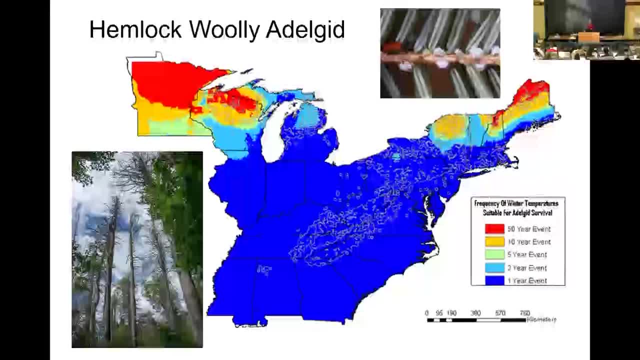 And, of course, as those forests end up dying, you know, in larger spatial, you know extents than we've seen in the past, that's going to have a much greater impact on those ecological communities. communities You might have heard of this species- hemlock, woolly, adelgib, or I guess you might have. 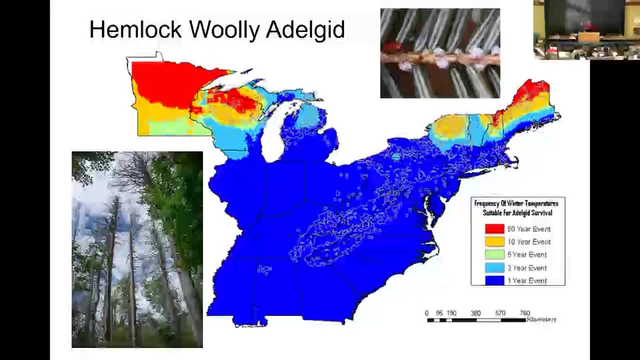 seen- you can even take a step back- the hemlock trees that are in this area. So we're really lucky. in Ithaca a lot of our gorges have these beautiful hemlocks. It's a specialized community that actually occurs, you know, up and throughout the east and up and down the Appalachians. 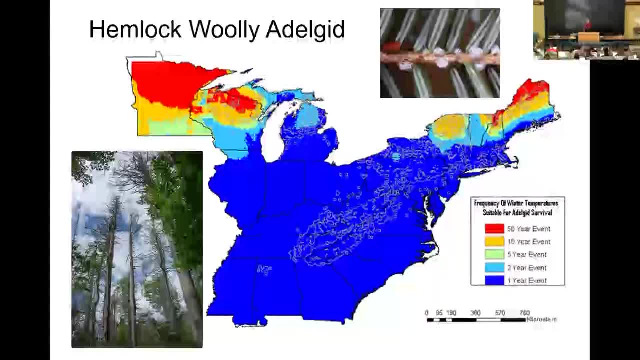 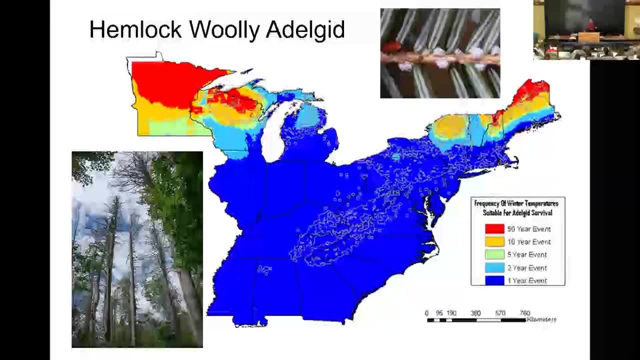 Unfortunately, there's an invasive bug, the hemlock woolly adelgib, that was introduced, that has been decimating and entirely wiping out in some regions. hemlock stands right so it attacks the, the hemlocks, but one of the what? what? historically? what we've seen is that the 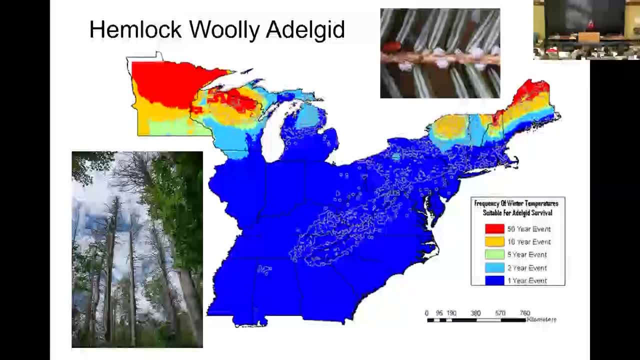 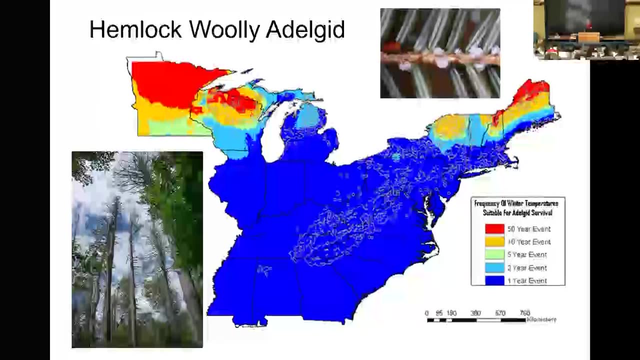 adelgib has been limited by winter temperatures, and so here in this graph, what you can see is it's showing that where the adelgib occurs, relative to how often it's basically a winter, is suitable for its survival. So blue areas show where, every year, basically, 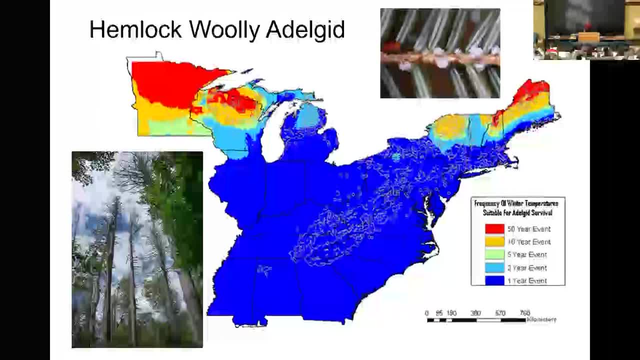 these, these adelgibs can survive, and so that's where you get, you know, really a lot of mortality. It's only when you have still has winters that are severe enough to really kill them As they're overwintering, that you don't see as much mortality of hemlock stands and not 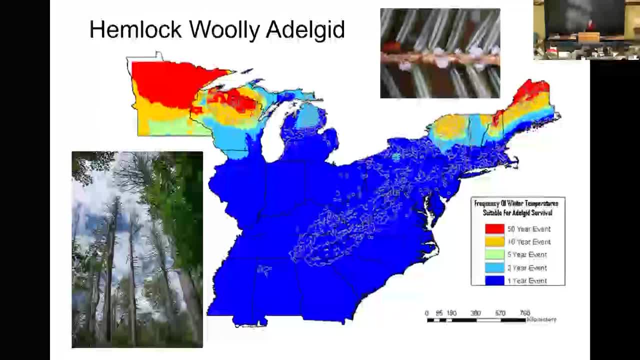 surprisingly right. that's moving north, You know, as temperatures are warming, so too is the range of the hemlock woolly adelgib, and that has a lot of consequences, you know, for you know other species in those communities, species that have, you know, evolved to specialize on hemlocks. It can affect. 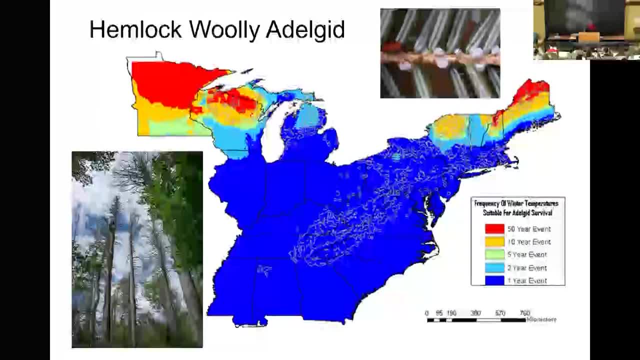 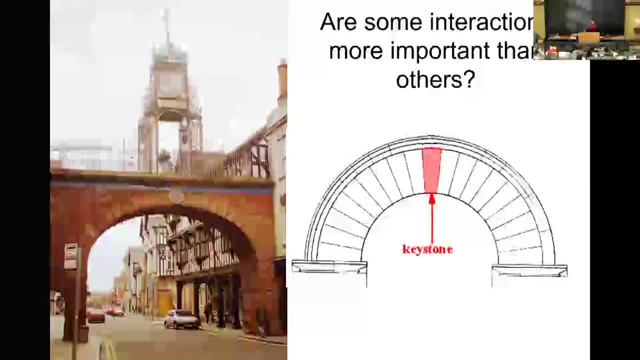 you know all sorts of other ecosystem processes, So we're really lucky in Ithaca. So, yeah, that just gives some examples of the different ways that when we start changing climate, we start changing the nature of ways that species are able to interact, And so we don't have a complete understanding of how all species interact. so that's really difficult. 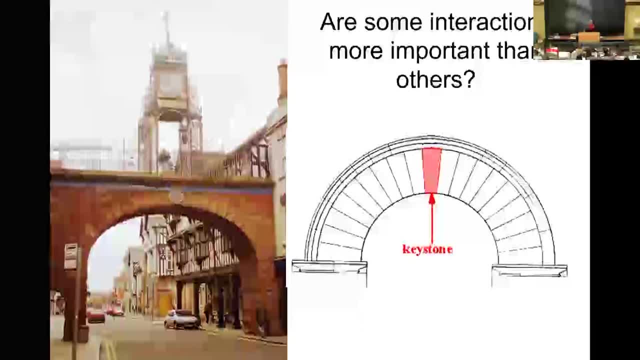 to predict them. you know where we're, how ecological communities are likely to exist or to change. One of the things that makes it even more challenging is that we know that some types of interactions are more important than others, and we- this is, there's a word- we. 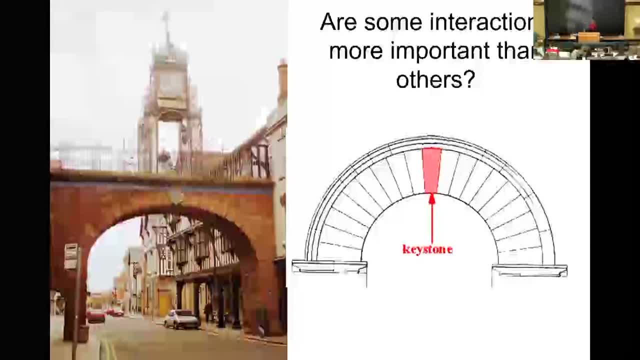 use for this in ecology and it's called a keystone species. and a keystone species is one that has a disproportionate effect on that community structure and organization, relative to how abundant it is or its biomass and the word comes from. you know the keystone species, You know that this is a keystone and an arch. right. You pull out that one keystone. 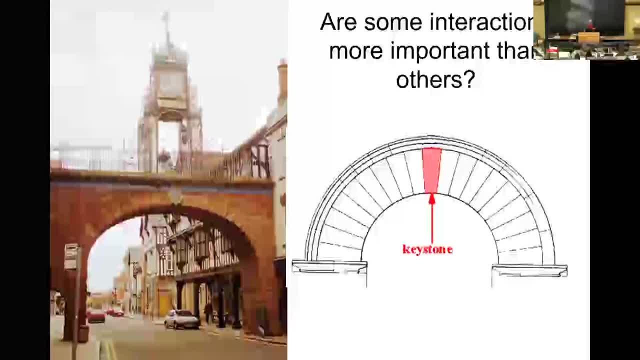 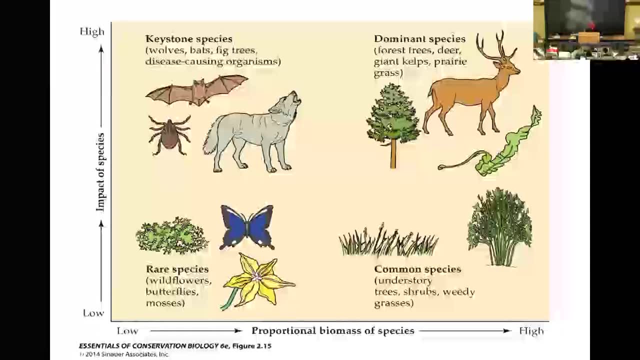 and the whole thing crumbles. and that's the same idea we get with certain keystone species. If they're removed from the system, all bets are off, everything can change. And one way to think about them. I find this, this particular graph, helpful, So it's showing on the 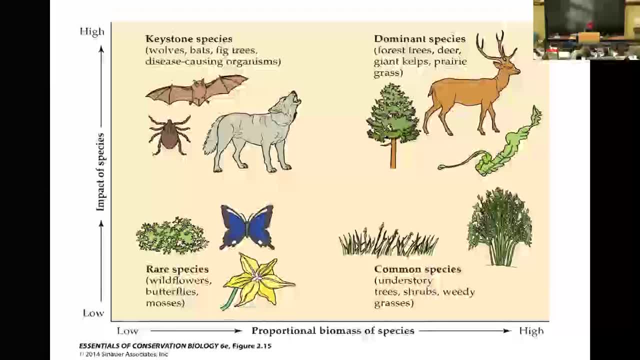 excess axis, the biomass of species, proportionately, And then on the y is the impact of that species. So for some species that are really dominant in a system, well, it's kind of a no-brainer that they're going to have a big impact, right, We think. 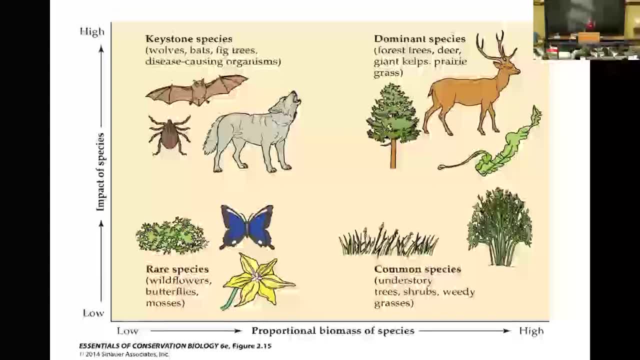 about deer. well, yeah, they're like everywhere. they're overabundant, they are having enormous impacts on our ecosystems here. But a keystone species is a little bit different because it's impact and it's disproportionate to its abundance or biomass in that system, And I'll give you some examples. So one of 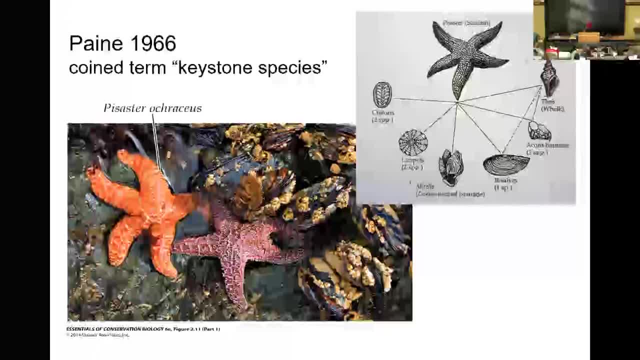 them is just the species for which keystone species was coined. So back in 1966, Robert Payne, at the University of Washington, he had been studying intertidal communities and so along those rocky ocean ledges, you know, in the Pacific Northwest, And there are lots of different. 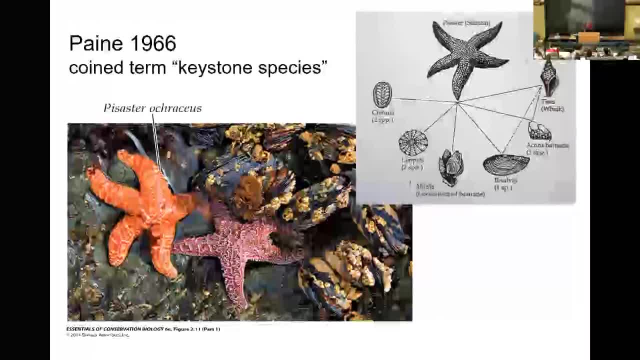 mussels and you know other mollusks that occur in those areas. And, the key thing, they're all competing with each other for space. You know barnacles and mollusks they attach, and so they're they're competing for space. The starfish is a. 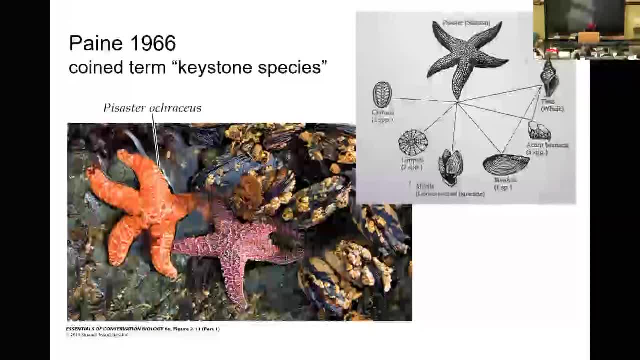 predator. It comes in and it will eat some of them and by doing that it opens up space, And it opens up space so that not only the most like, dominant and competitive species, but also the most dominant and competitive species in the world are able to persist. You can imagine if you were to leave that intertidal 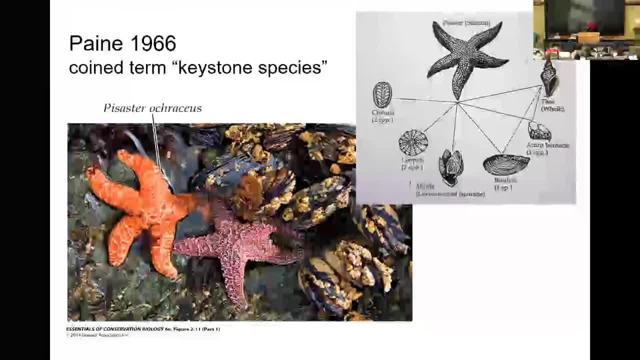 community. eventually, maybe one or two species takes over everything, Kind of like how zebra mussels might be doing, you know, in some of the Great Lakes, But with starfish, because they're removing some of those really abundant and really 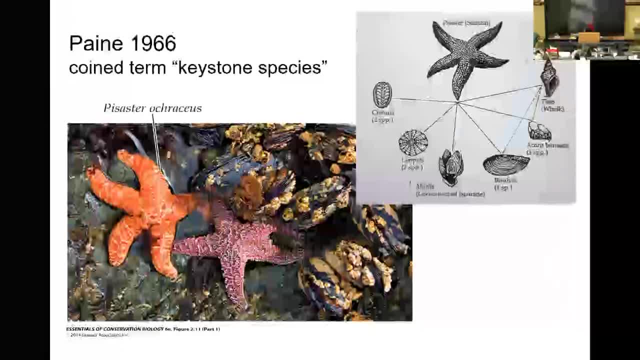 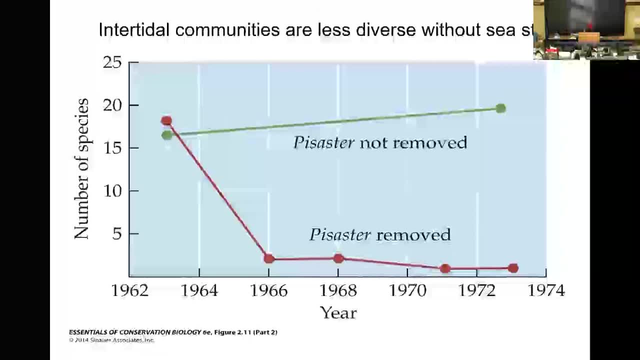 competitive species, it allows less competitive ones to coexist. And so they found this is the case, you know, if you look at where, when starfish, you know starfish, that's the genus, or sea stars, I guess, were removed. you have, you know. 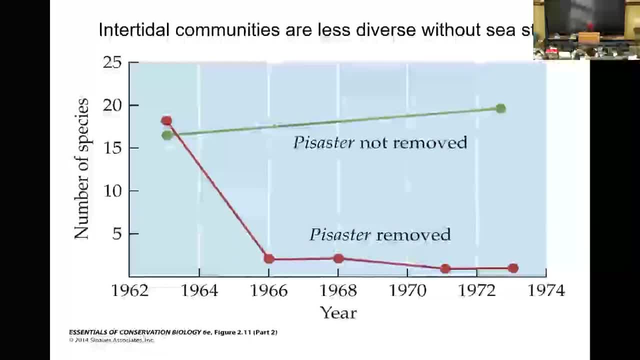 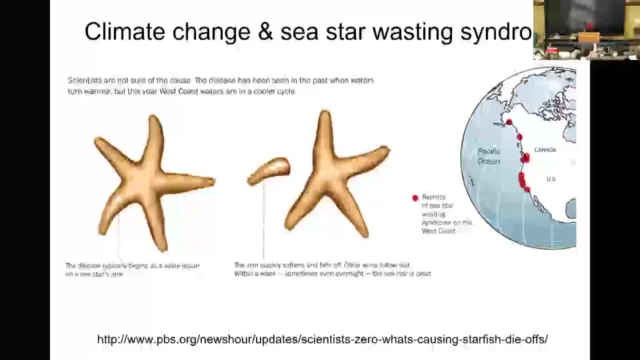 very low numbers of species, Only a couple, persist in those intertidal zones. But when you retain the sea stars, well then you have a much more diverse community. So to go back to climate change, then, well, one of the issues that 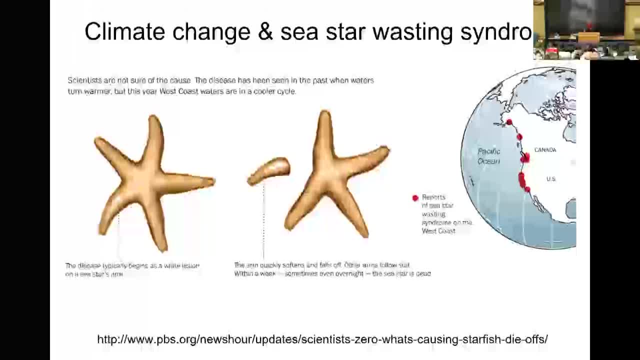 we know is is happening now in the along the Pacific Coast is that the likestars are reducing. So what we're seeing by that is that there's a disease, There's a sea star wasting syndrome- Not quite sure of all the causes- and 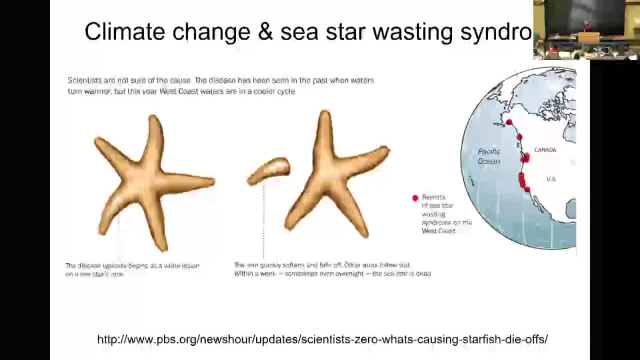 drivers of it. Drew Harvell and the EEB here actually studies this. But we know that as temperatures are warming in the ocean, we have much more outbreaks of this wasting syndrome. So again, temperatures are affecting the species and it's a vulnerability to disease. 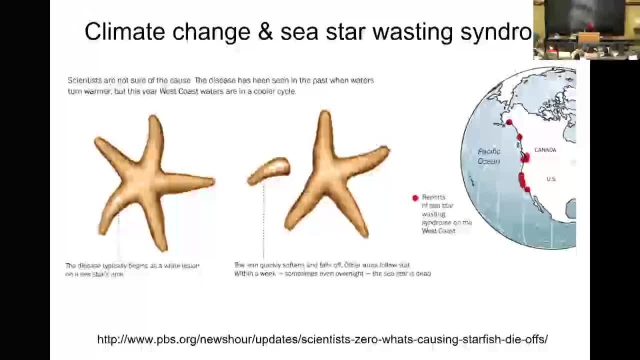 it's a game changer for those communities. Again, this really illustrates again why it's so important to think of all those species interactions, right? Because if one was just considering, well, I don't know what might intertidal communities look like in a warmer. 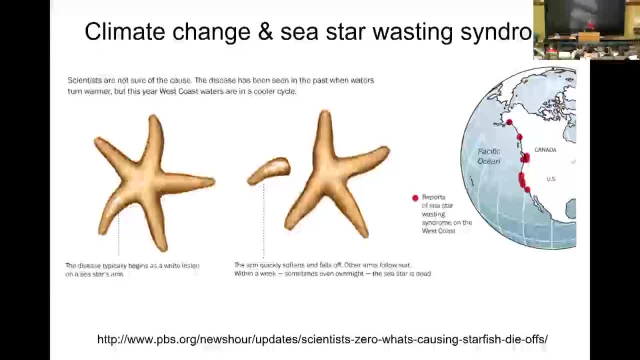 climate And you just plot it out- Well, what's the tolerance of different species to different temperatures, and kind of map out how they shift. It might look straightforward, But if you miss that, sea stars have to be there in order for that community to persist. 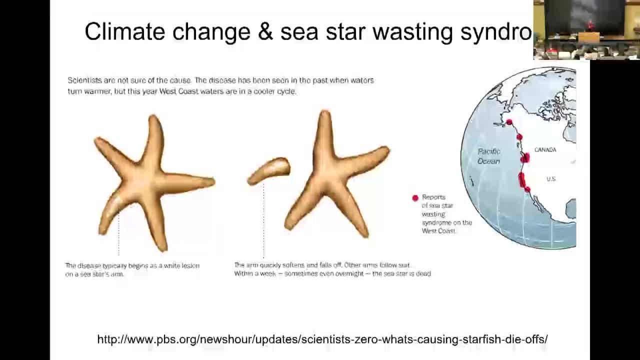 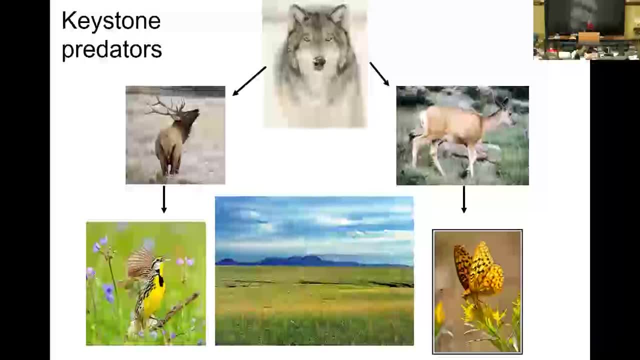 and to maintain those interactions. well, all bets are off there. So other examples of keystone species include other keystone predators like the wolf. That's a good example. right Studies you might have heard out in Yellowstone National Park found that when wolves were removed then you have increases in some of the ungulate. 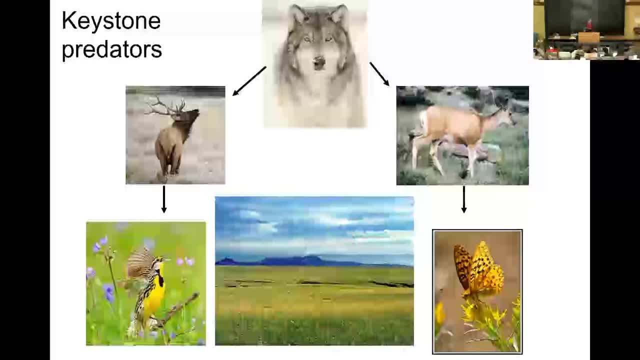 population, And so that's a good example. And so that's a good example, And so that's a good example. And also changes in their behavior. Without a predator, they can just sit in one spot and just kind of munch down the vegetation all day long. When there are predators, they're on the move a. 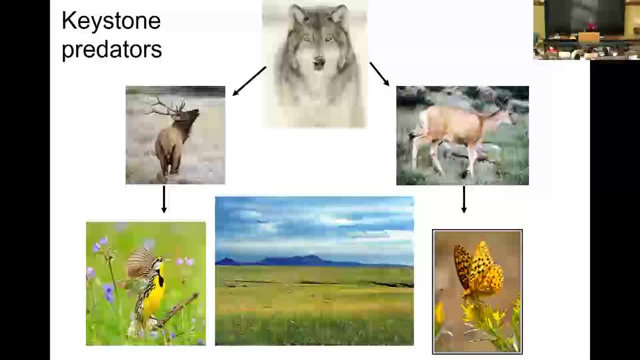 lot more and less likely to have really strong impacts than any one specific location, And so those changes, those ungulates then, are having then enormous effects on the plants and then, indirectly, the birds and the insects that use those plants, And so that's a good example. 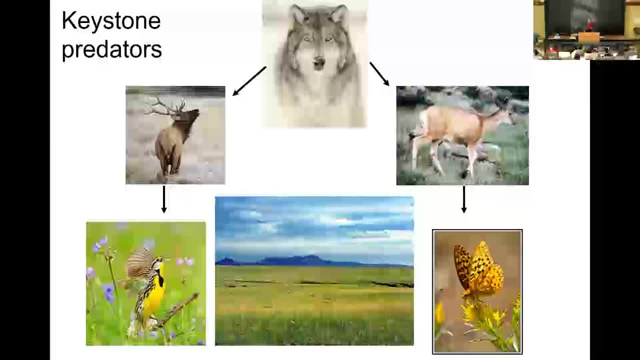 And so really that wolf is a keystone species that really helps maintain the communities in that entire system. And so, again, when we start losing some of these predators, because maybe they're more vulnerable to changes in temperature, precipitation or other consequences of climate, 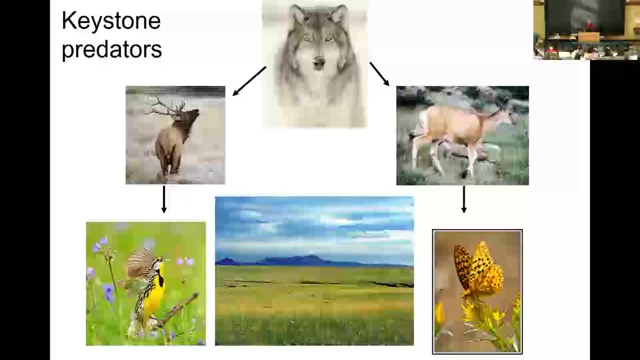 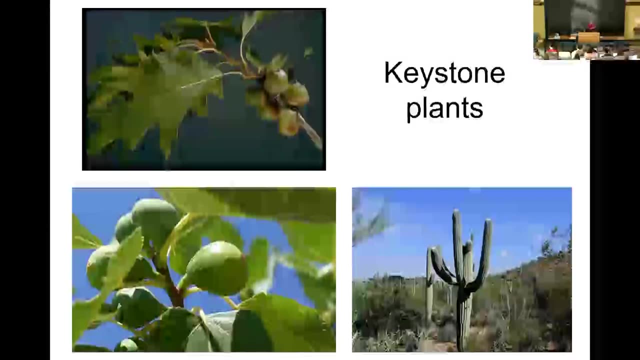 change we might be, you know, really causing, you know, in much greater amounts of change in those ecological conditions, And so that's a good example. And so that's a good example. And so then, if we have any more species- there's still a lot- we still have the possibility that maybe a little. 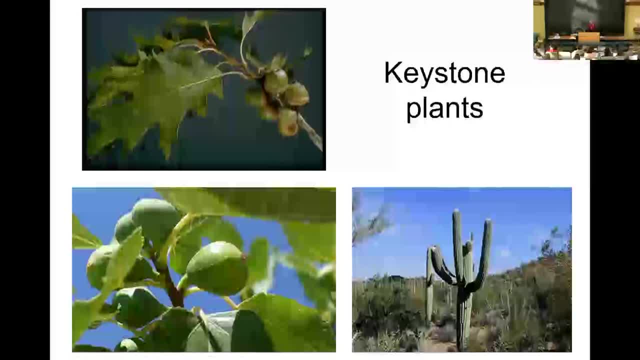 more back in our normal days, that the effect of the plants on our owniecities and our own habitats would not be knocked back as quickly as the effect of the plant scout or the effect of our ownecities changing. Did you hear it? 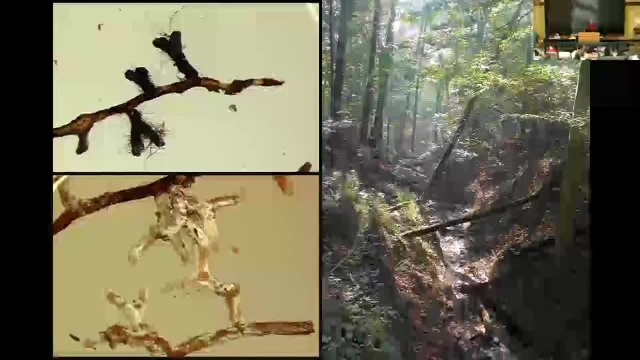 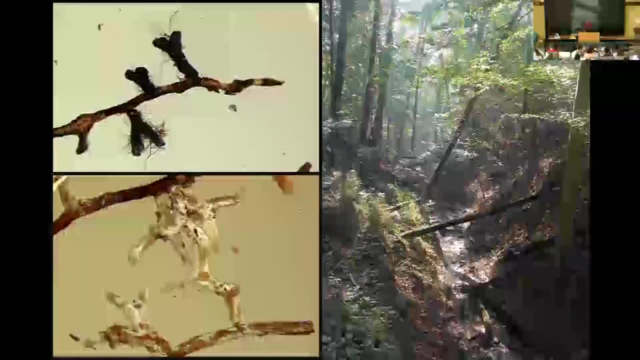 — it can be kind of cryptic. You might not even know about it. This is a picture. you're seeing mycorrhizal fungi, which is actually mutualism between fungus and algae, and mycorrhizal fungi help. They're in among the tree roots and a lot of. 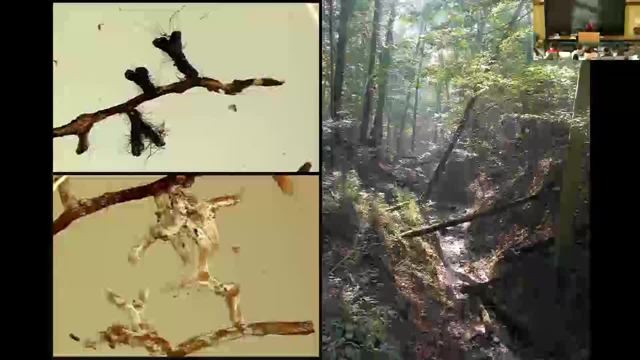 plant roots and they help them to, you know, uptake to absorb nutrients, right. So this is. and they found that for some forest types you really can't even regenerate a good forest without the appropriate mycorrhizal fungi And so 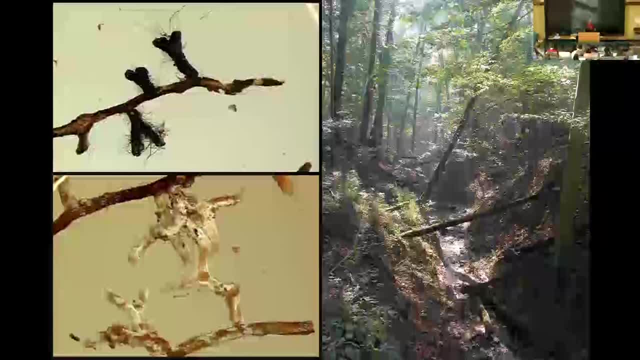 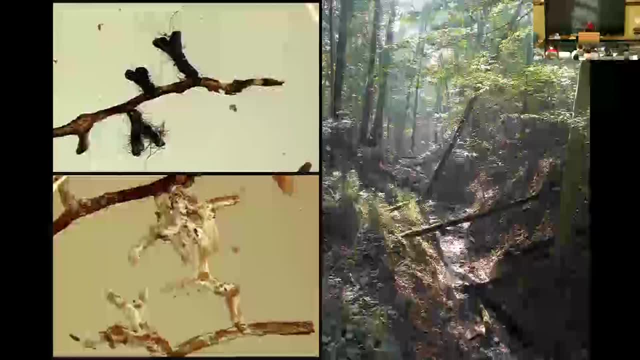 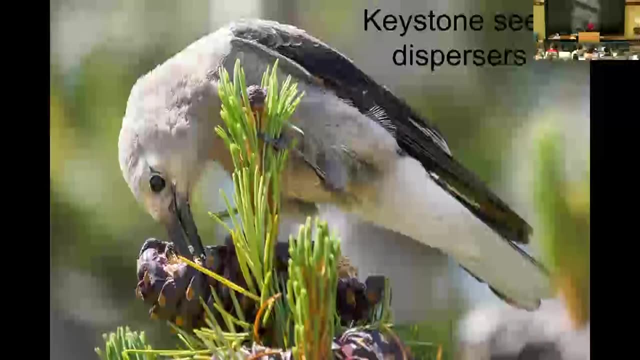 these are again species that are occurring within the soil. We may not even be aware of how they're responding to climate change, but if we lose them, we could lose the entire forest ecosystem. There are keystone species that are responsible for seed dispersal that are being affected by climate change as well. 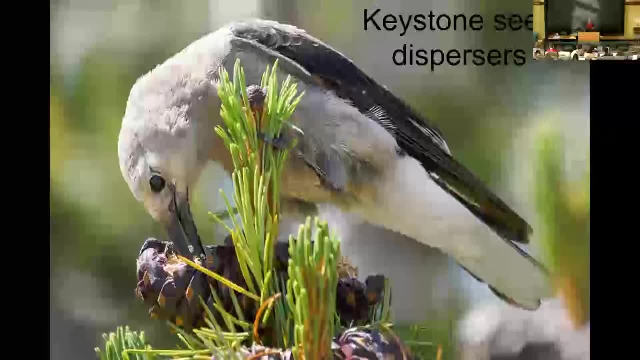 So Clark's nutcracker is one that is responsible for seed dispersal that are being affected by climate change as well. So Clark's nutcracker is one species that is responsible for dispersing the seeds of whitebark pine. It's a really tight mutualism and climate change is affecting both the 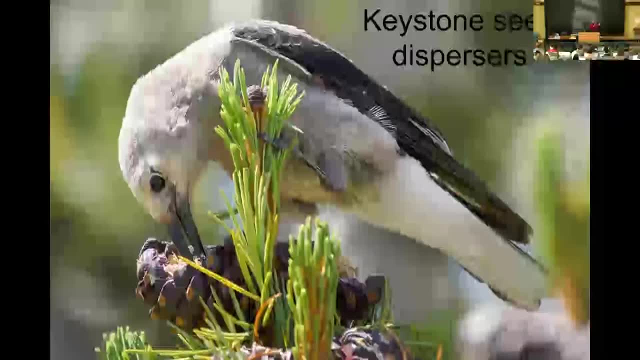 distribution of whitebark pine, you know, and so it's actually ranges shrinking. That's affecting the Clark's nutcracker. but the Clark's nutcracker is also being affected by climate as well in ways that might affect its ability to. 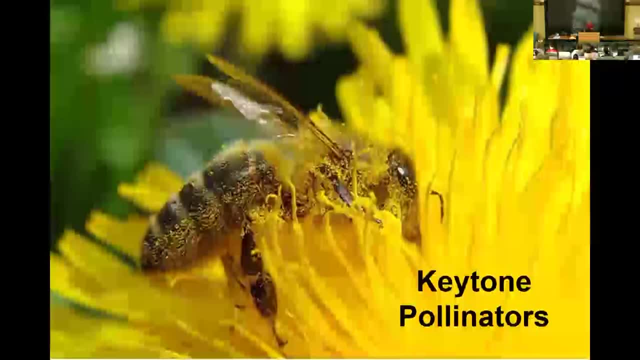 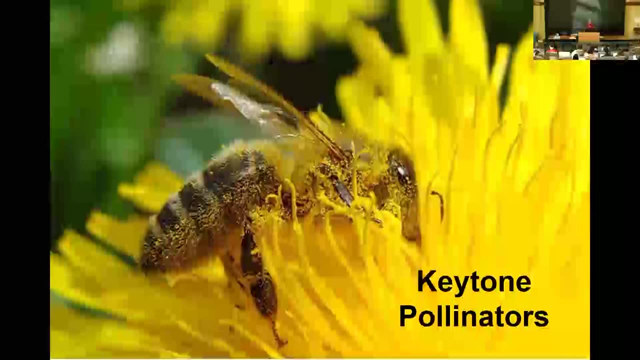 keep dispersing seeds of whitebark pine, Same with keystone pine, Same with keystone pollinators. We've already given some examples of that, but whether it's a bird, whether it's an insect, you know. again, that's, if we lose one species. 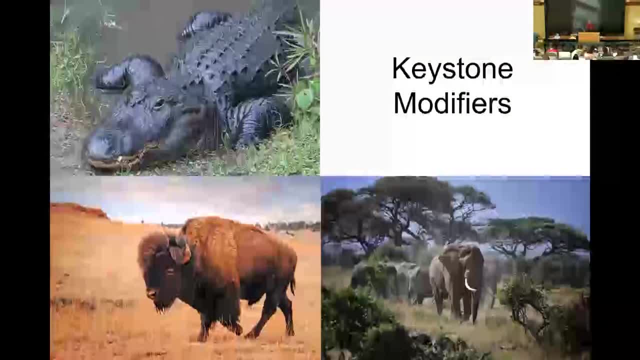 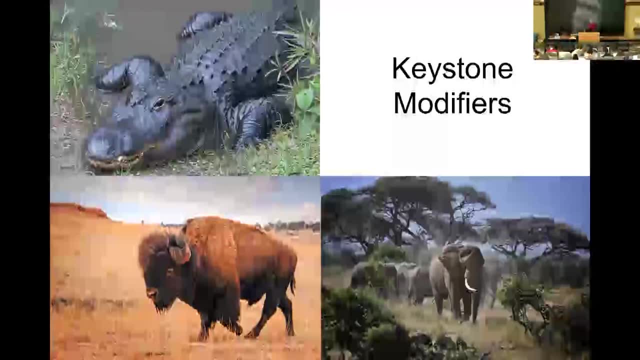 we're likely to see consequences with the other. I wanted to just spend some time on modifiers as well. This is a group of species that's really interesting, where they're actually modifying an environment that makes it suitable for other species. So with alligators. 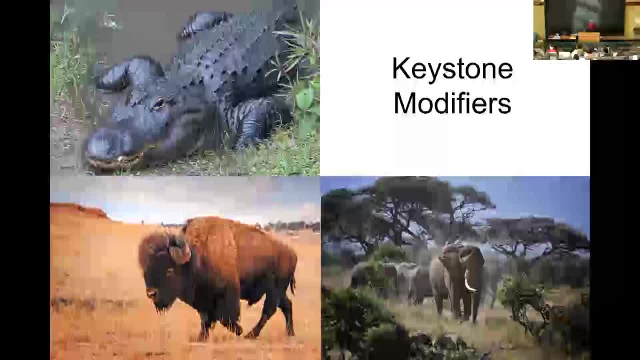 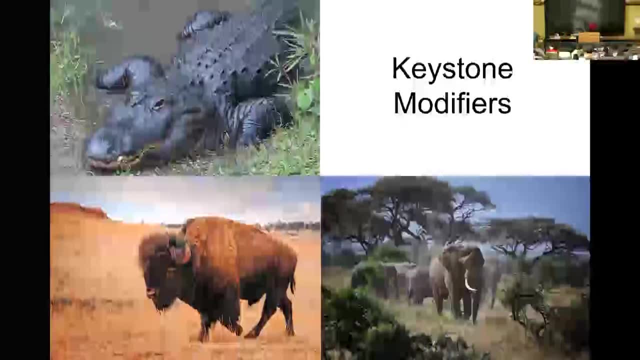 we know from studies that alligators and the wallows they make open up some vegetation-free areas in the marshes where they live, and that allows you know habitats for species that like a little bit more open water, And so you'll get. 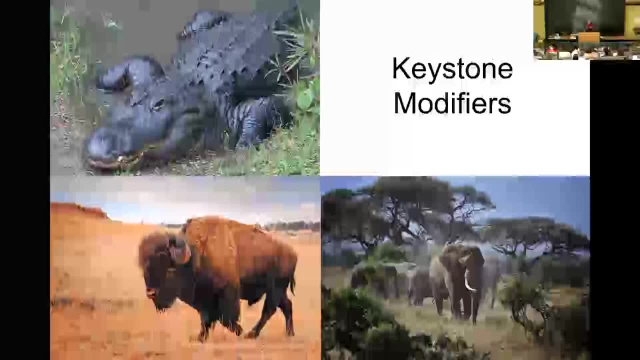 you have different species that are present in marshes with alligators than without. Bison. also, you know, are keystone modifiers because as they're grazing on rangelands they're not going to be able to get to the bottom of the marshes And you know they're changing the plant species composition in ways. 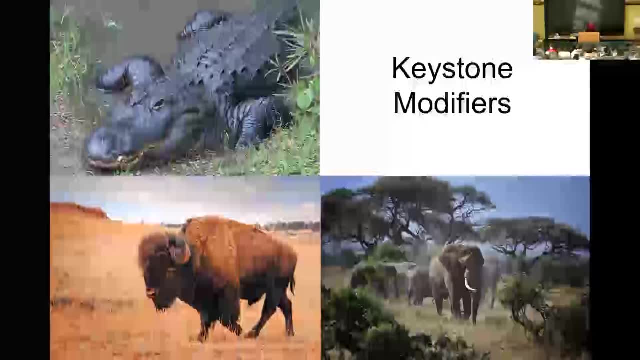 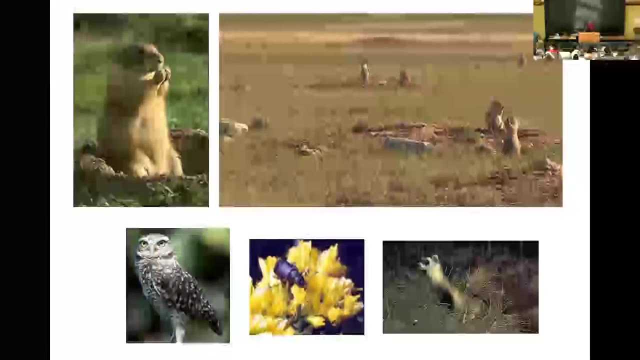 that allows more diversity as a whole, Elephants- you know another example where they're ripping up a lot of vegetation. they're a disturbance force and other species use that kind of disturbed or in a successional habitat. Just another couple examples I thought you'd find interesting, like prairie dogs, towns in. 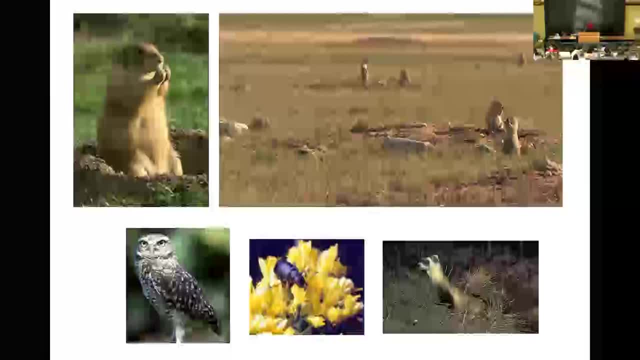 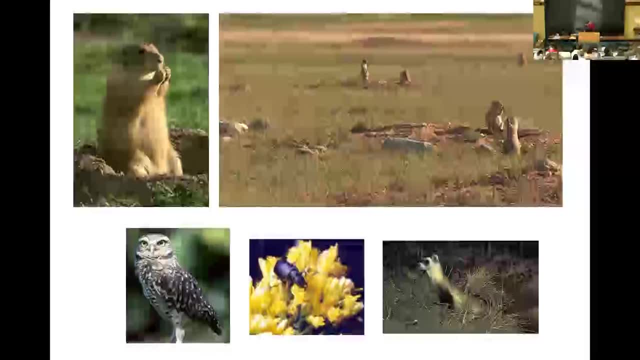 the in the western US. So prairie dogs, you know that I mean. even though a lot of ranchers might not so much like them because of their effects, they actually are providing, you know, habitats for other species. We know that burrowing owl, black-footed ferret, an. 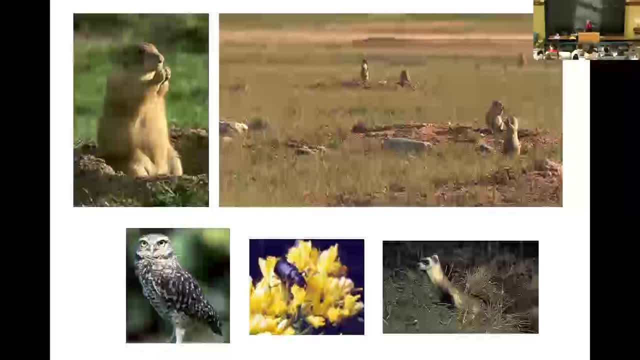 endangered species. they're using those prairie dog holes and colonies you know for their to provide. you know whether it's nesting or roosting, you know their dens as well. And then, because prairie dogs will clip the vegetation right around the 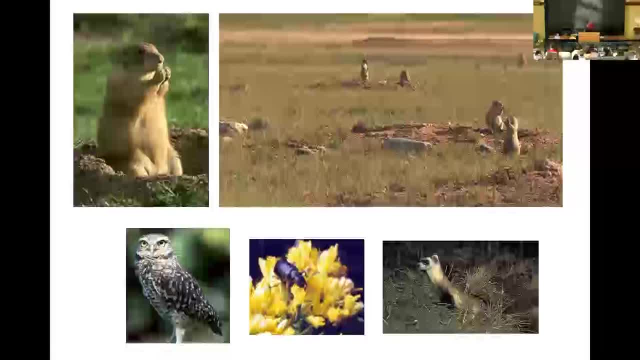 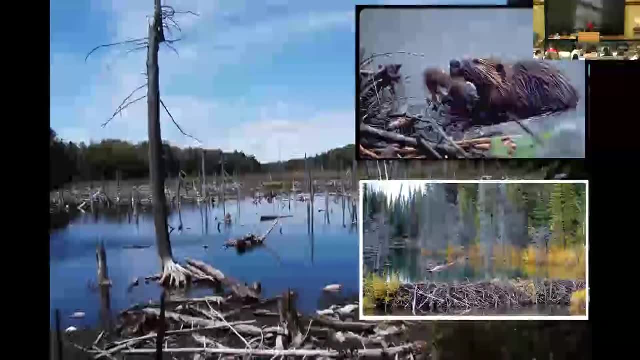 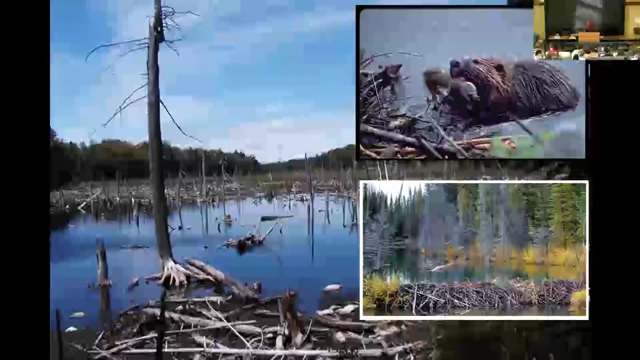 entrance to their holes so they have better visibility that affects the plant community. So again, you have more diversity and greater numbers of insects. Beaver is another example of a modifier around here, though you know we talk about different disturbances that are really important in parts of ecosystems. 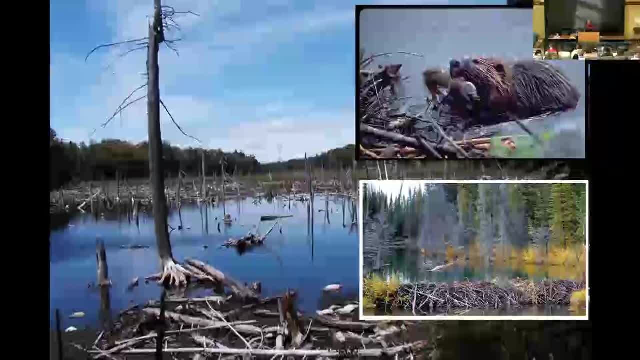 And in the Northeast. beavers are the world's largest NSA Vegel Species and even in the Northeast They do have more diversity in greater numbers of social- are actually one of the most important disturbance agents. So they come in, they'll cut down trees. 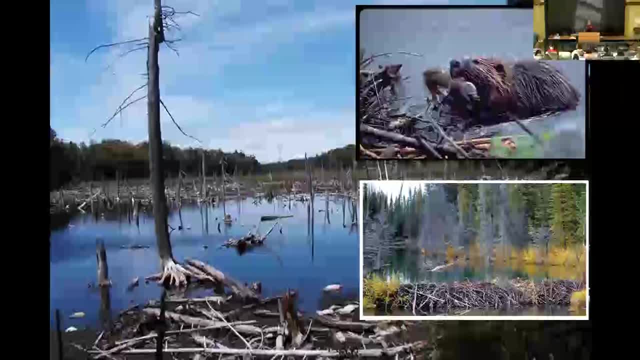 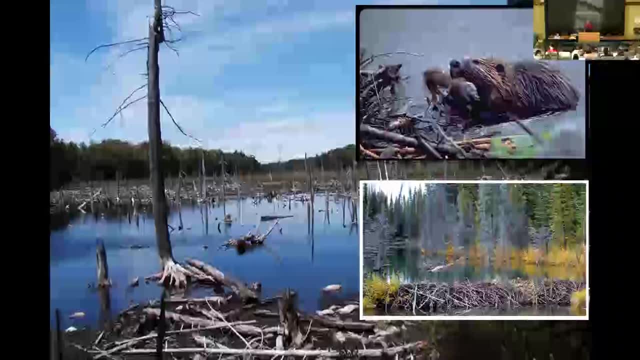 they build their dam, it floods, And so you first might get a wetland or a pond. eventually the dam breaks and then you have a meadow and ultimately forests regenerating in those areas. So there are many different communities that are associated with those different stages. 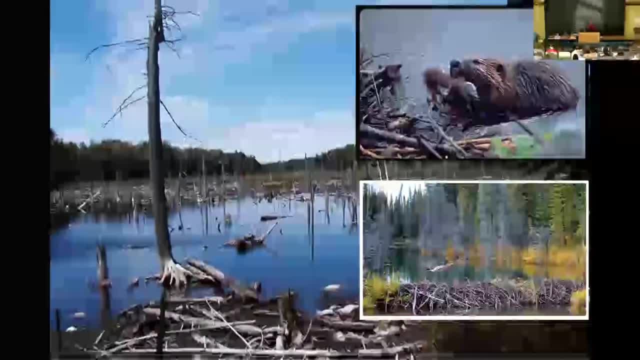 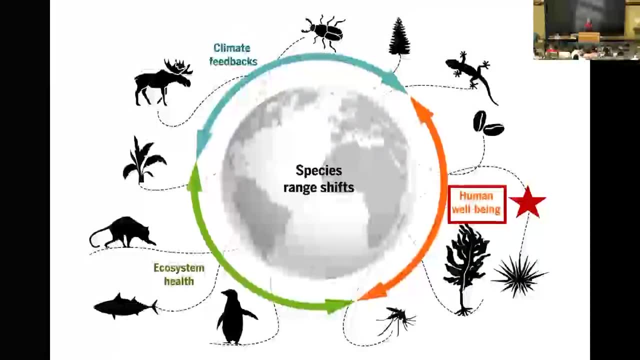 that could, in theory, be affected if you lose that one species. So again, the point here: the take home message is just that, with a lot of the predictions that we're making about changes to ecological communities, we have not progressed this far when it comes to understanding. 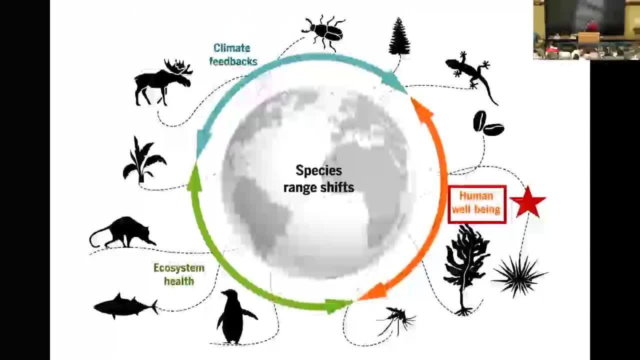 how interactions might change, And so some of the examples that I'm sharing is really meant to kind of impress that sometimes, just when you tweak some of these interactions, you can have really large consequences, And we don't have complete knowledge of the way species interact. 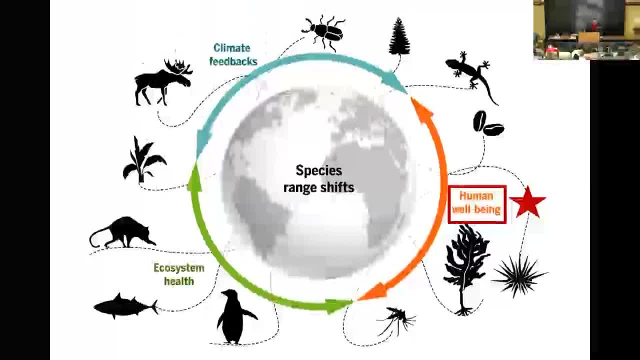 or how communities are gonna be affected when those interactions change, And so this is a great role for those of you who might be interested in ecology and biology to explore. I wanted to just end, too, with some of the ways that these changes can affect our interests as well. 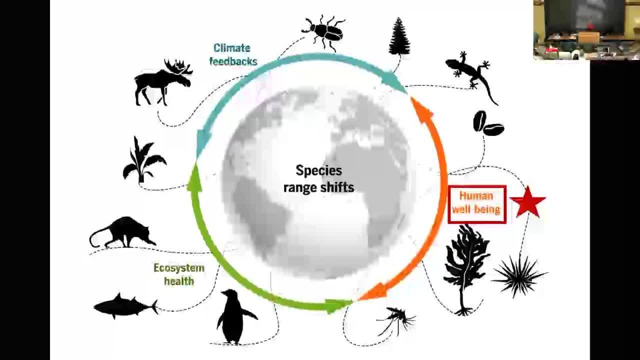 right, We know that we're part of the ecosystem as well, So changes that are happening, we're not immune from them, And so for human well-being, just to kind of bring this home, I mean, you've probably heard of the pollination crisis. 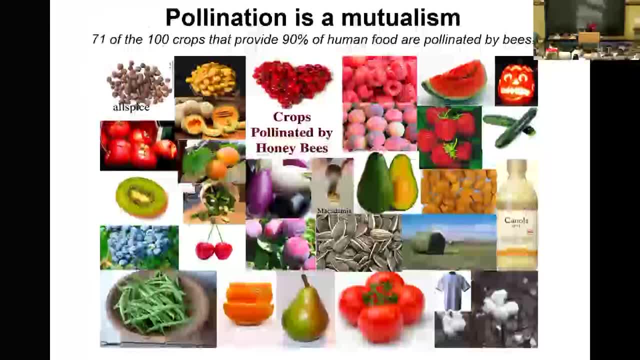 People are really concerned with declines of pollinators because when you look across the food security, think of food security- most of the crops that we depend upon globally are pollinated- Are pollinated by bees. So if we lose bees, 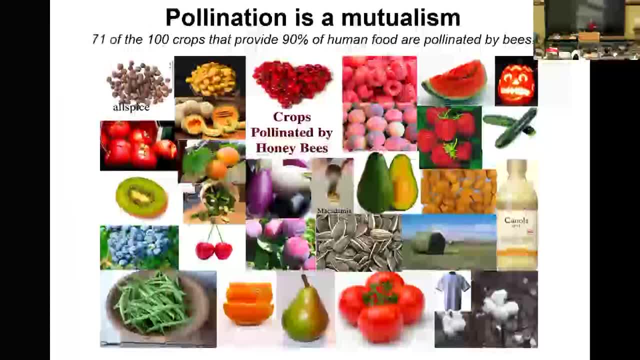 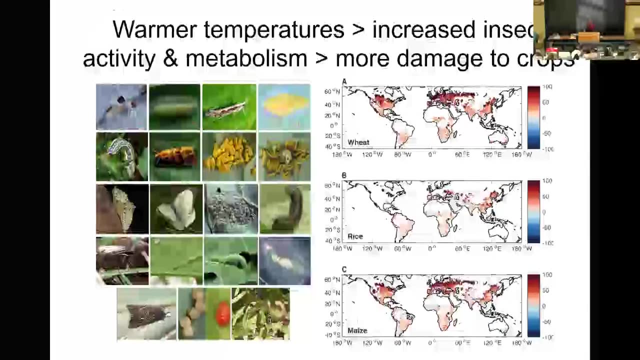 if they're affected by comets, certain species or in certain regions, that has the potential to dramatically affect the abundance of certain foods. There's been some research too, showing that with insects, their metabolism is oftentimes related to the temperature. 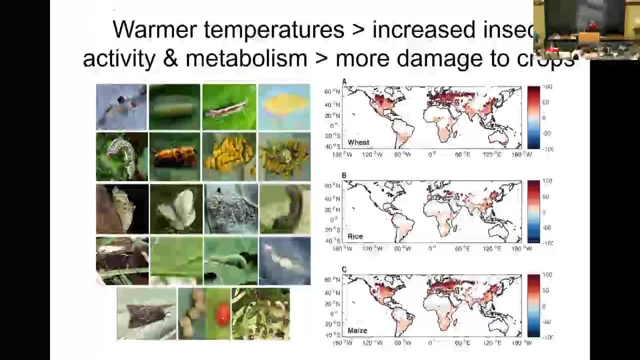 the ambient temperature, And so as temperatures warm insect metabolism, so their energetic requirements are going to increase and their activity levels increase as well, because they're cold blooded, And so they've projected, then, how warming temperatures will affect some abundant species. that can damage crops. 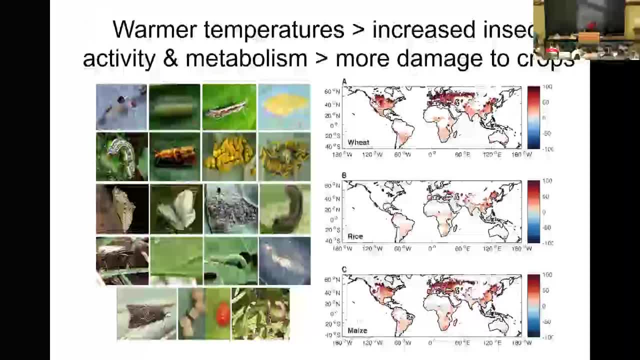 and actually showed how that might play out in terms of affecting production of wheat, rice and maize or corn. And so the red colors on these maps show where you're going to get increased damage to crops And the blue is where you'll get reduced damage to crops. 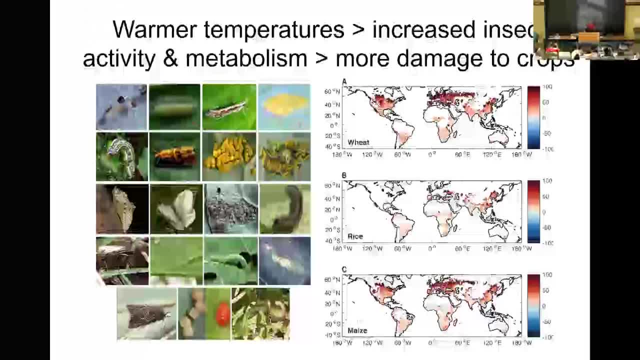 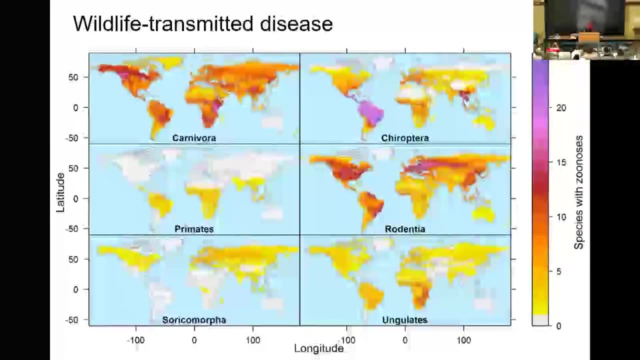 But you can see for most of them there's a lot greater damage that we're expecting from increased pest activity than gains we'll get from it. And the last human example I wanted to provide was related to disease, And it's a good time. 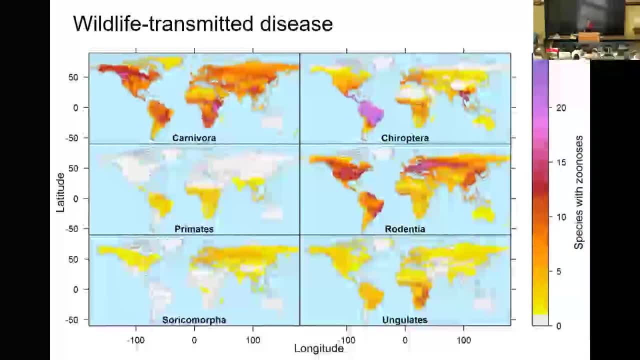 We're thinking about coronavirus now, recognizing how vulnerable human populations are to different disease outbreaks, And there are many different diseases that are transmitted by animal vectors, And so this was just showing- this was from a paper showing the number of species that carry diseases that could impact humans. 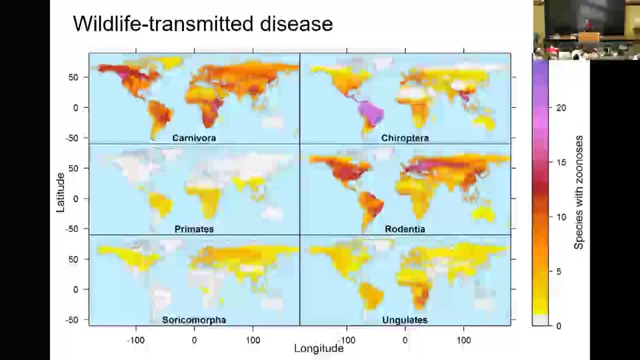 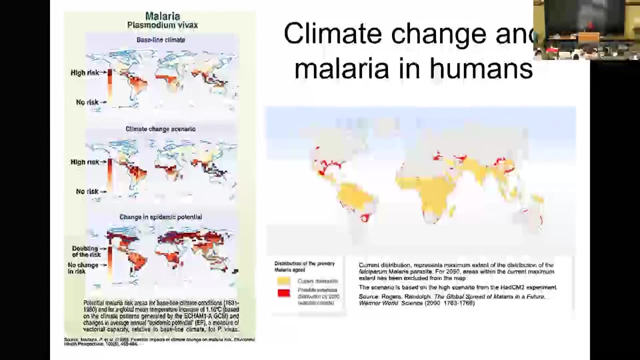 Around the world. So, whether it's, you know, carnivores or bats, primates, rodents, shrews, moles, and then ungulates, you can see- And malaria is a good example of where they've actually shown- that changes in temperature are going to affect. 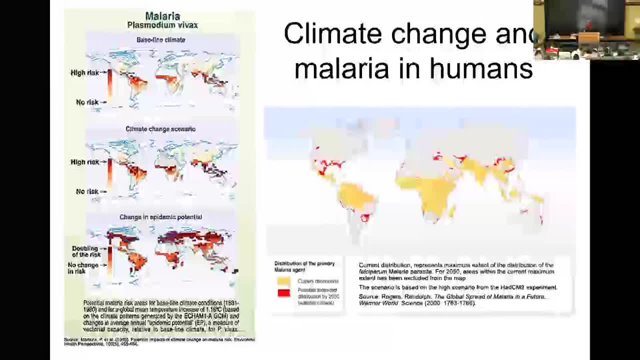 the distribution of mosquitoes that carry malaria And that is going to affect the risk or vulnerability of different human populations to malaria, And so on. this the maps. there you can see areas where they're expecting that you're going to see far greater increases in risk. 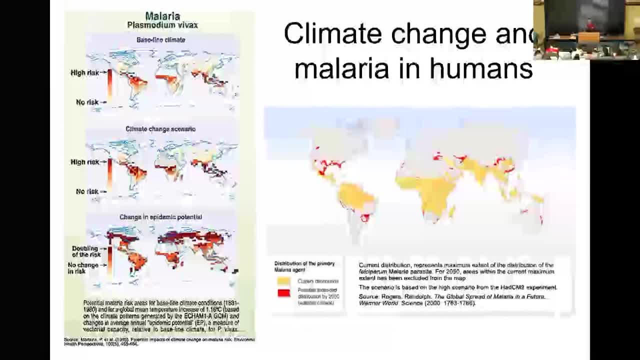 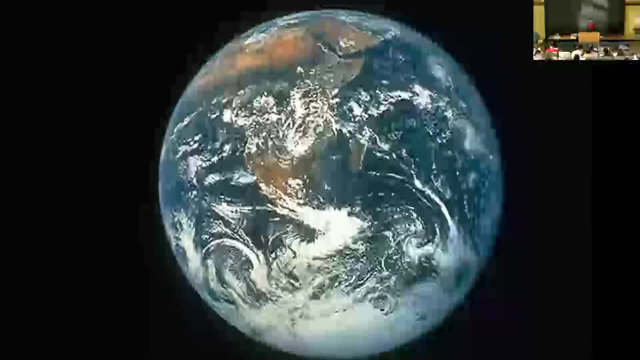 sometimes up to doubling the risk of an epidemic of malaria occurring in the future. Again, that's fundamentally a species interaction. So with that, you know, I think now we can open it up. I know you know Peter asked we have to have some time for questions. 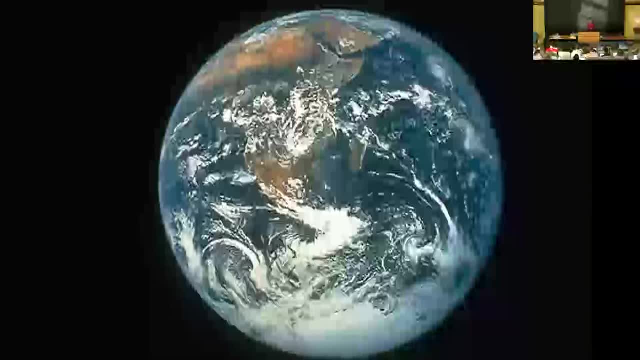 Hopefully. I'm, you know, happy to talk about any of these examples We can go back to if you have a question about a specific slide. So yeah, thank you. Yeah, Yeah, sorry, Last part, Where? what species? 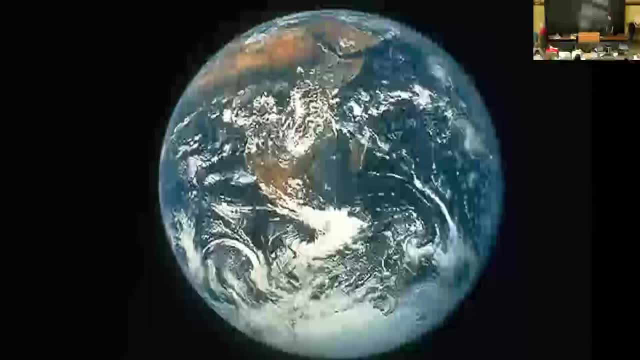 So the question was: are there examples of when, like a non-keystone species, might actually sort of transition to become a keystone species in a given environment with change? And I think offhand I can't think of an example, but that would certainly seem to be a possibility. Right, If you lose some species that are really maintaining that community. it could be as a community shifts, a different predator becomes really important or a different plant really becomes the base of that maybe entire food web. But yeah, that certainly would be a possibility. 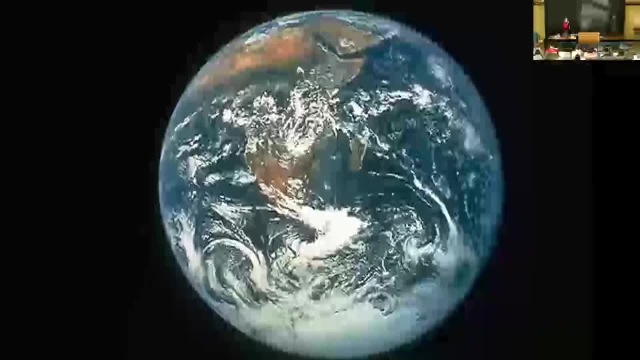 I'll have to think of some examples. Yeah Yeah, So sorry, I couldn't bring the speaker. If you have a question, raise your hand and I'll bring this microphone to you, And then also remember if you want credit for your question. 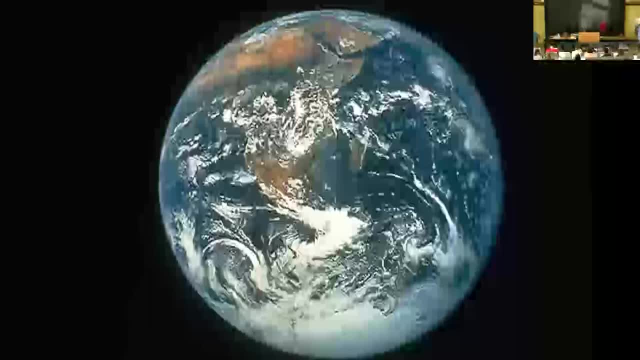 come up to me afterwards. Okay, I know you talked about temporal and spatial kind of resilience. Do you think any species that have like a faster reproduction rate or, like you mentioned, insects that are more resilient- more resilient to the effects- is that because their life cycle is shorter than maybe the birds? 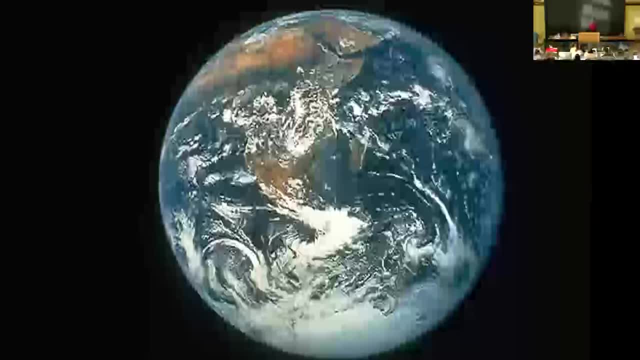 or does that play into it at all? Yeah, So that's a great question. And so, right, when we think about different sort of life history strategies of species- you know, historically we talked about them in a really simple way- 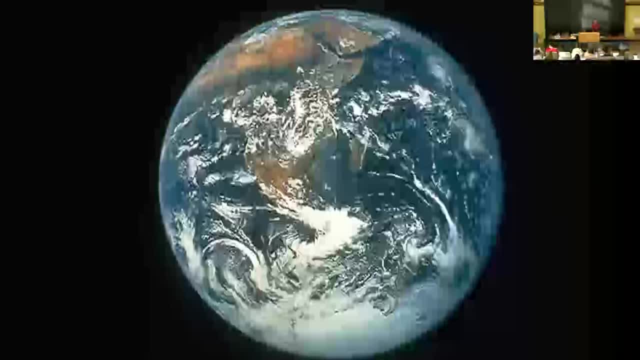 like our selected species, species that have they reproduce quickly, they have short lifespans, they have they have the potential for really rapid increases in populations but also really fast crashes. So insects, small mammals, you know, those are good examples versus like K selected species. 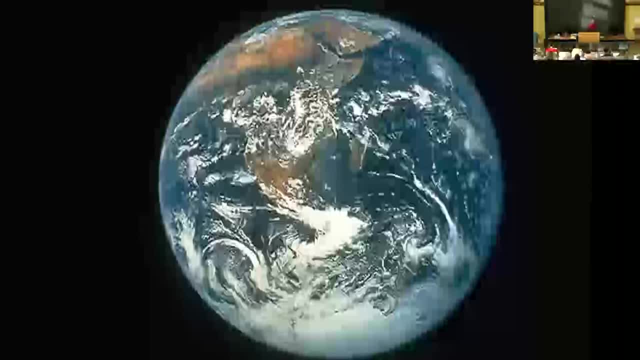 People would talk about them that are more long lived, low reproductive rates, but because they're long lived they can sort of endure bad conditions, let's say. So that would be like you know, whales and elephants and pandas, or you know. that are, that are on that spectrum. So in general, yes, one would expect that species that have greater reproductive capacity, you know are able to to both, you know have produced more young that are able to disperse, but also, when the shorter generation times are going to, you know, just all else being equal, should promote the ability to adapt right to the natural selection to act on those populations than for long lived species. But there are lots of different nuances, right, And so, like the adaptive, the adaptive potential of any given population is also going to be related to the amount. of genetic diversity, which is related to the size of the population. So there are all sorts of other factors that one would need to consider. but yeah, that would certainly, you know, can certainly be one right. Small populations, low growing populations. not much reproductive potential. Yeah, they're a bit more hamstrung when it comes to the opportunity to really track a rapidly changing environment, Specifically speaking to the bees. do you know any research that's currently being done of trying to help with it? 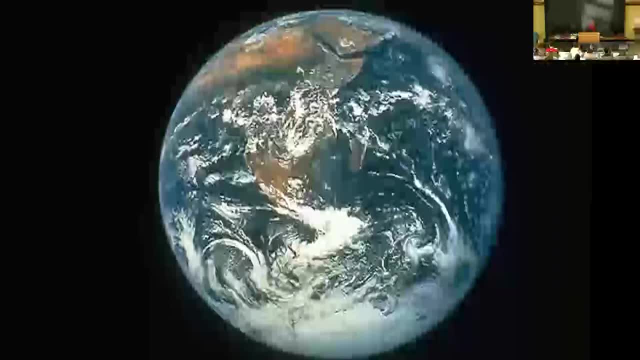 Because obviously the issue that if we lose the bees then we lose most of our food sources. So I was just curious if you knew any potential research Right. So that yeah, Yeah, Great question. So with the bees just sort of writ large and pollinators. there's a lot of attention right now going into, you know, pollinator populations. So again, this is I don't. I'm not deep in that world, but my understanding is that they're sort of too general. They're probably way more. 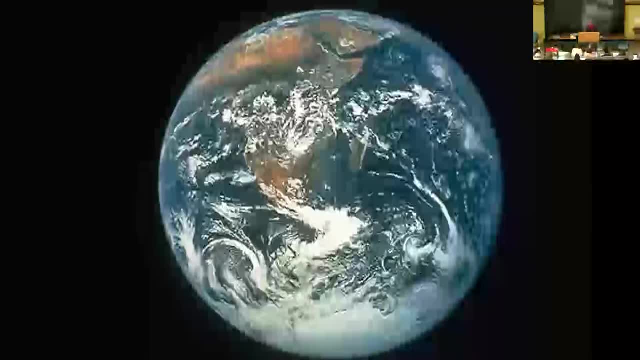 this would be oversimplifying, But in my mind there are sort of two general tracks. There are two general tracks of the kinds of solutions people are talking about to deal with the pollinator crisis. One is actually looking at some of the 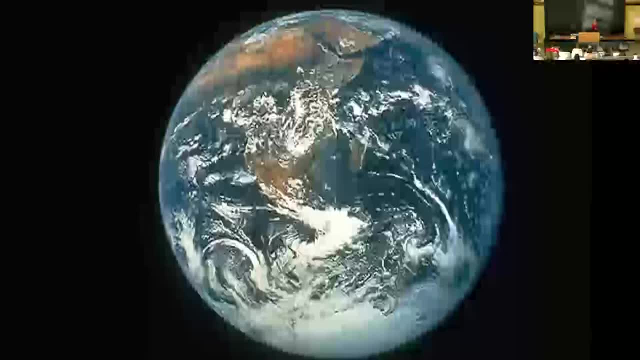 like the disease, like the colony collapse. What are the drivers? Where is that? How can we actually manage that disease or reduce the vulnerability, reduce the spread? So it's really that's kind of a disease focus and how we manage and transport colonies. 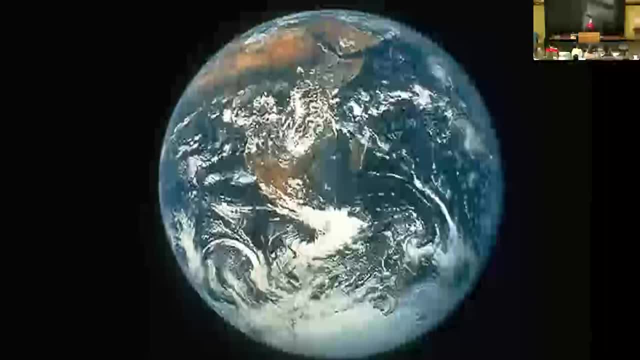 right How we're managing those. One is related to the habitats and how we're managing those, And so there has been a lot of research showing that bees not surprisingly need, like diverse wildflowers, you know, diverse plant species. So in a landscape, 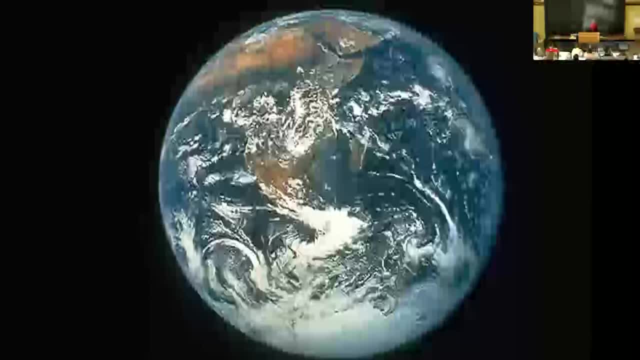 in some of our like Midwestern landscapes, where maybe it's a sea of corn, you don't. you have farm, you know. edge to edge cropping, you know. so there's not hedgerows that are available anymore, You know. 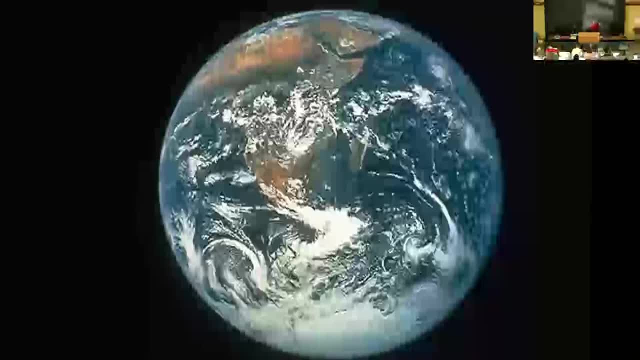 it's a very homogeneous environment. Those are really bad for pollinators. Well, it's just about any other life other than corn and maybe people at that place. But so there people are also looking at how can we actually design and manage habitats and landscapes that are more supportive of. 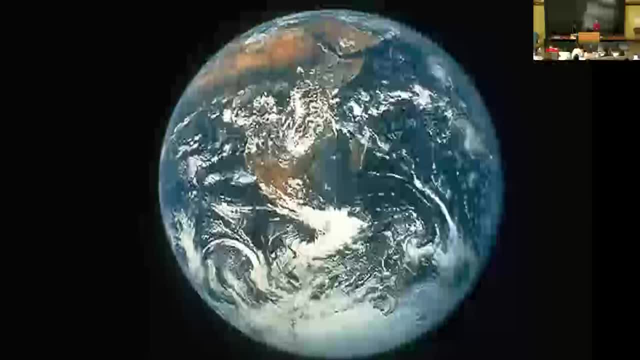 you know, survival of of some of these bee populations In terms of temporal and spatial mismatch. do you think that there's any solution, especially with the birds and other insects? You mentioned how the insects are able to adapt faster than the birds are. 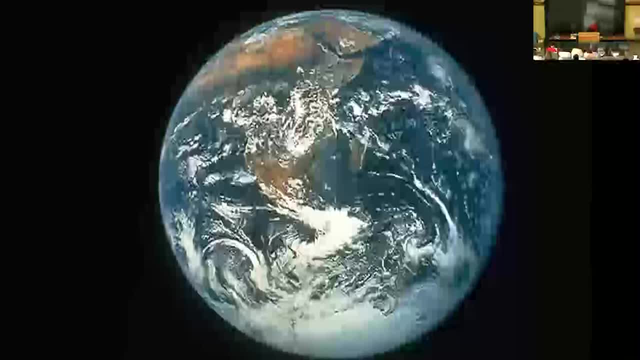 So is this going to be a cycle that can't be avoided, or is there some solution to this? Yeah, I'm not sure of any. I don't think I've heard of any interventions per se that are that are being attempted to try to help close the mismatch or the timing. 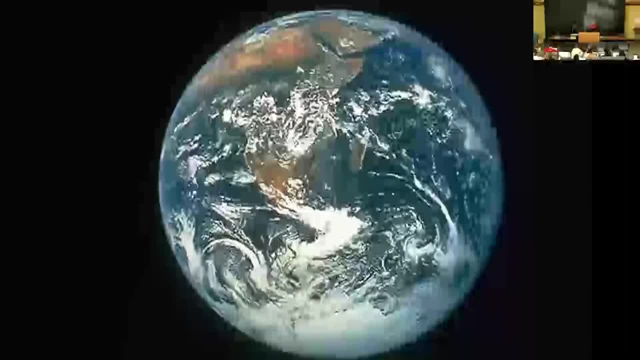 of those events? What? what? one of the? yes, I'm not sure. I think generally for those kinds of things, you know the, the idea is protecting as much habitat as you can across as broad of a range as you can. 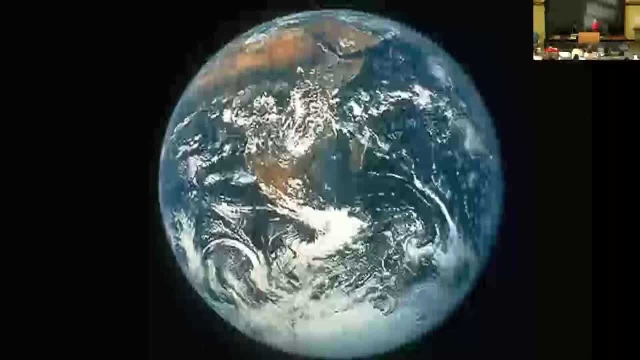 So you're capturing sort of different temperatures, you know so maybe there are some places where that mismatch is less likely to occur. in general, Again, these are sort of indirect strategies. to maintain, you know, large kind of healthy populations of these species is another way of. providing I don't know some insurance. I guess in some ways, because, again, the more individuals you have in a population generally, the more genetic diversity, which means that you have more diversity of exactly when they nest, the timing. 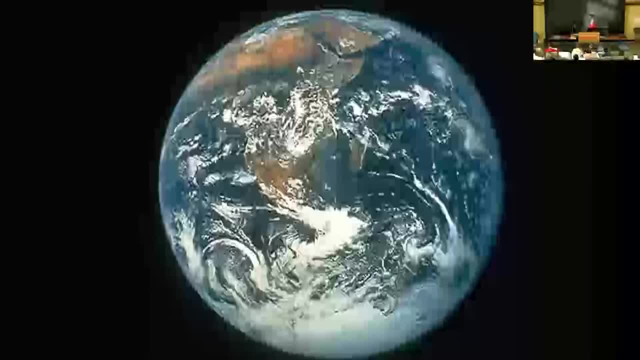 you know their ability to adjust, And so if we can maintain populations that are diverse enough genetically, then there's greater chance that they'll be able to adapt in ways you know over multiple generations to track those changes. But yeah, 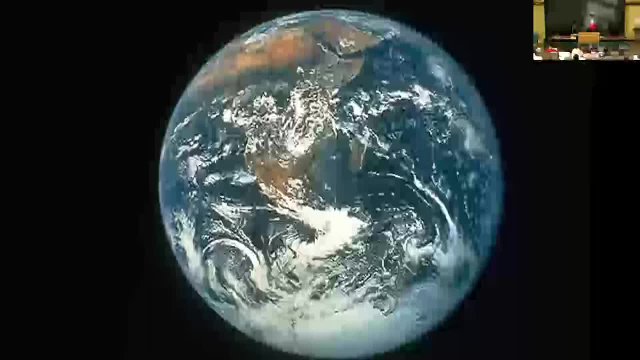 I'm not, I'm not sure if any interventions for those temporal mismatches right now. You mentioned about the increase in effectiveness of certain diseases And I was wondering if you knew of any specific cases where you've seen, if you knew of any specific cases where humans almost struggled to keep. 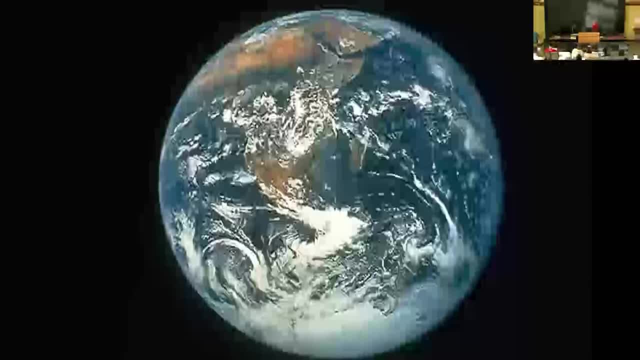 up with these changes or where, like, mutation speed of these diseases has kind of increased So new diseases have come up faster, to where the point where humans can't keep up Right. So some of the places where, like in terms of like, shifting and changing climates and the disease and changes in land use. you know one of the. so a lot of these disease outcomes you know are really the nature of the disease but different species of of of natural life, you know wild life transmitted diseases. Those are really sensitive to changes in the distribution of wildlife. 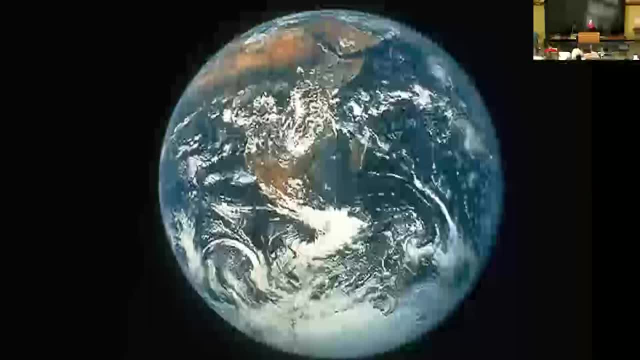 species which are affected to by how we're using land. So if we so, for example, when you Go on that you know there are cases where maybe forests are opened up to logging. You used to have really low density. 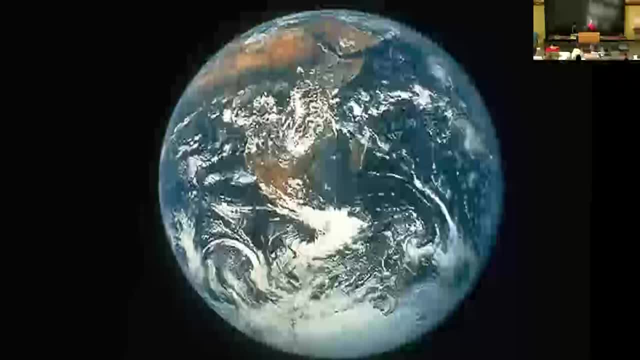 You know human populations for logging or mining, You have roads come in, you have much greater populations, much more hunting and exploitation of the wildlife, And so that's bringing more contact together. So really, that contact with the disease vectors is oftentimes responsible for that. So in a changing climate, 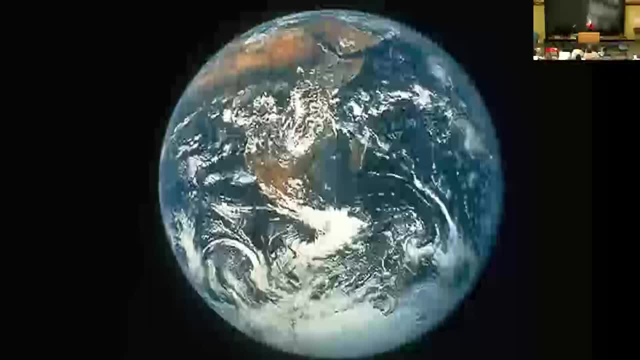 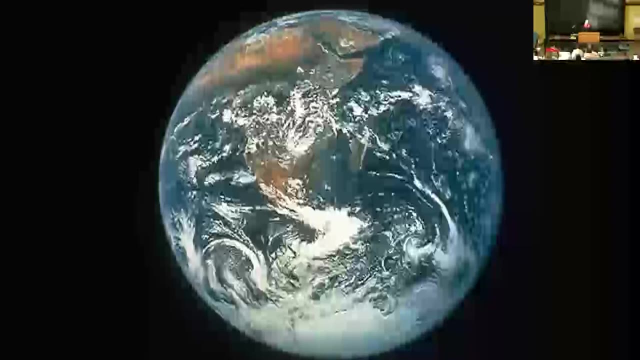 you know any of those, any drivers- climate drivers- that are affecting where people are moving, what they're using. you know the resources that could affect them, disease outbreaks, And it can be really complex and really fascinating too. So I'll just give one example too, with. so you think. 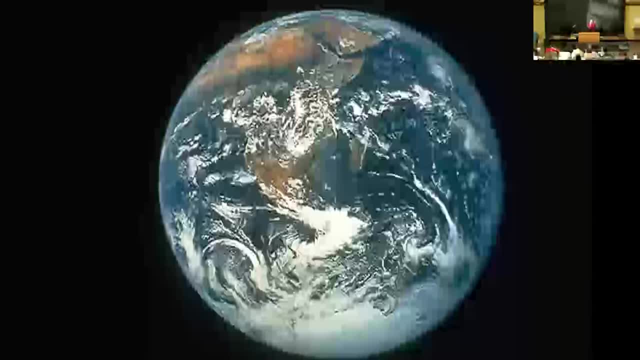 of human conflict. you know, wars, refugees, climate. I mean, right there there are strong links. There have been a number of studies that look globally and as temperatures rise, and well, I guess the climate, it's all about the climate, And so I think that's a really important thing to think about. 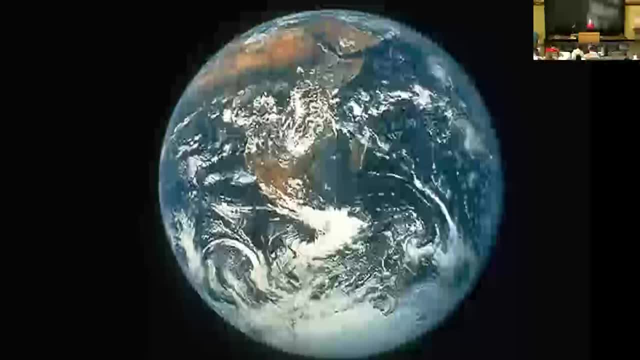 There's also droughts And as droughts become more severe, a couple of things are happening, But I mean, one of the big ones are that resources become much more stressed. So you have people can't have access to the resources they need because of severe droughts, you know, and hot temperatures. 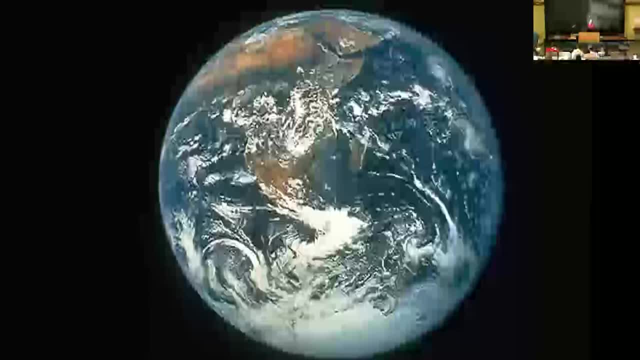 And that results in more conflict with human populations, which can prompt refugee crises. You know where now you have dense concentrations of people- you know who are- who are not doing well in terms of their health right, They're struggling because it's incredibly difficult. 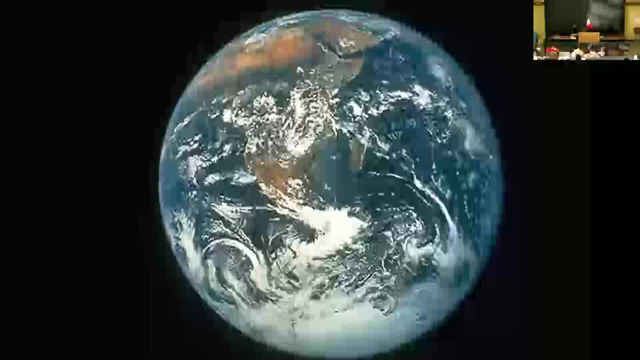 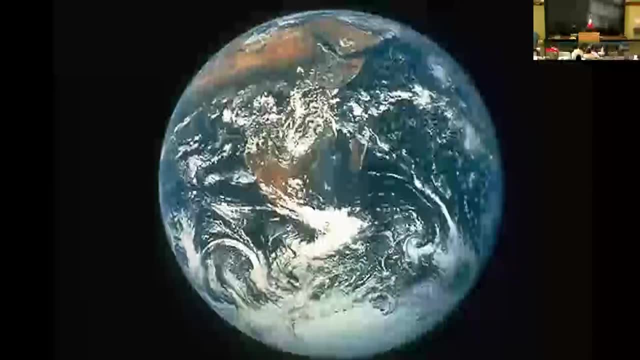 hard on their health, They're more vulnerable to disease, and in high density camps, often that are great places for epidemics to bloom. That would be one Wars. the same way, When you have conflict in areas you tend to have a lot of- and there have been many examples- then when 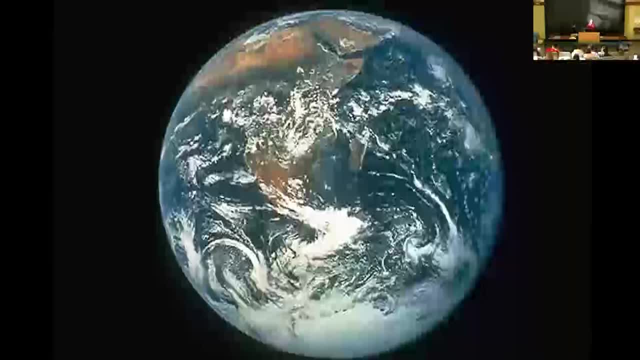 you have local, you know armies or military groups. you know they've moved into some new area. they need food, they start hunting more wildlife. So again, that's going to bring people together or in contact with some of these vectors. So there are many different ways that this can play out. 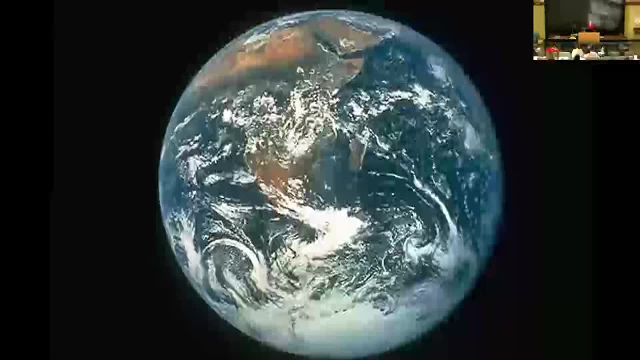 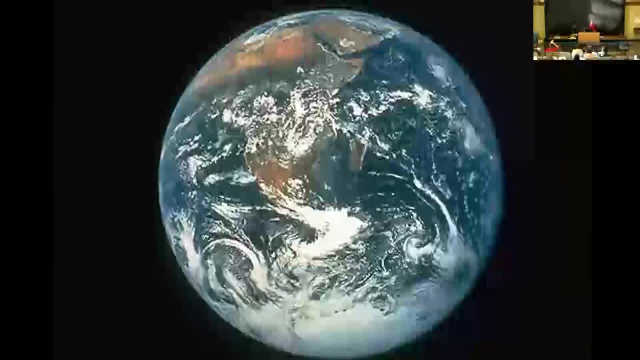 like a species out of a community that it would like obviously be rippling effects to an extent. So what makes you know the label of keystone species, like given to one over the other? Sure, So so all species right within a community. it's true that every species you know like 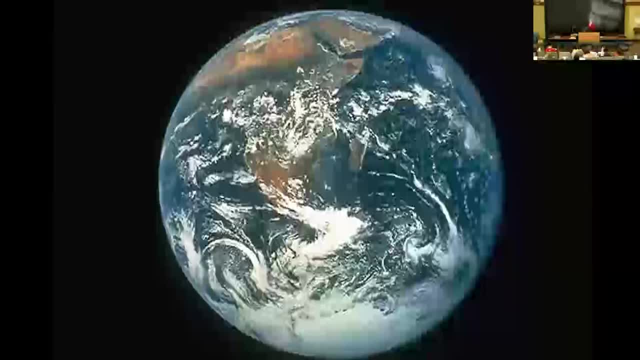 know, in theory should be directly or indirectly connected to another. So there, you would think there might be a signal if you pull out any one given species. However, in diverse communities there's oftentimes redundancy in the roles that species play right. So you could have, let's say, 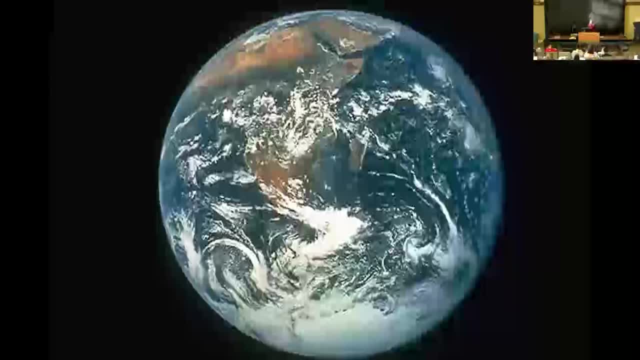 let's say there was, you know, an important. you know there might be multiple pollinators of one plant species. So if you pull out one of those pollinators you might still be able to maintain that community structure overall. So there are examples where, probably of species that 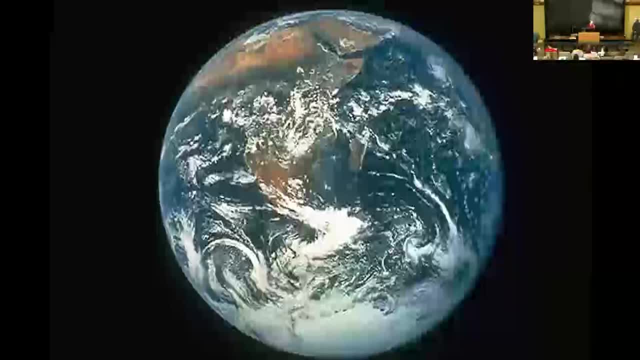 if you were to lose them, at least to the extent that we are aware of their impacts, which we are not oftentimes. so that's a really important grain of salt you know to attach to this. But so there could be. 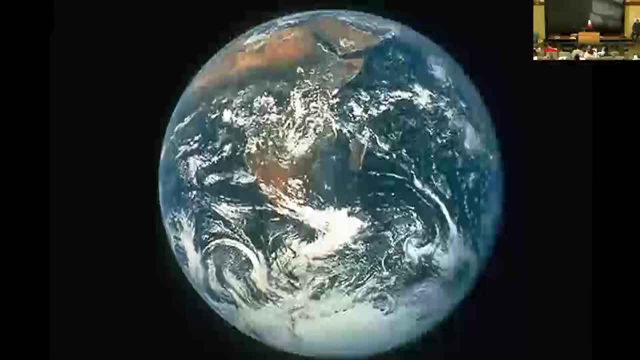 cases where one species could be removed without enormous consequences, But again those tend to be in certain kinds of community with a lot of redundancy in the role species are playing, The keystone species. that idea again is linked to a disproportionate impact on that community. 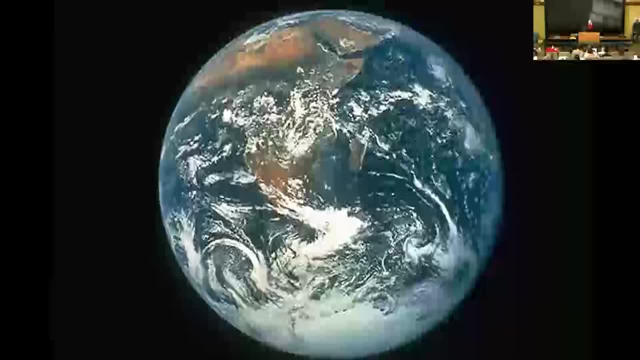 structure relative to the biomass of the species, right? So it's not just that you know it's really abundance, but it's really playing the, the nature of its interaction. it's playing a critically important role in that system And I 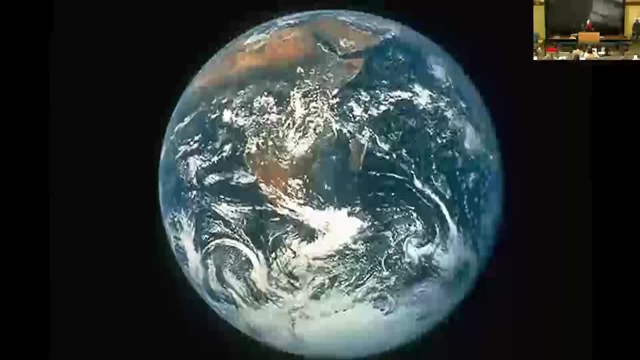 am. I will not advocate. you know that it's okay to just lose any species in part. well, I mean, there are lots of different reasons when we think of species conservation. you know from, you know ethical moral, you know all those reasons to more utilitarian. you know how will it affect us. 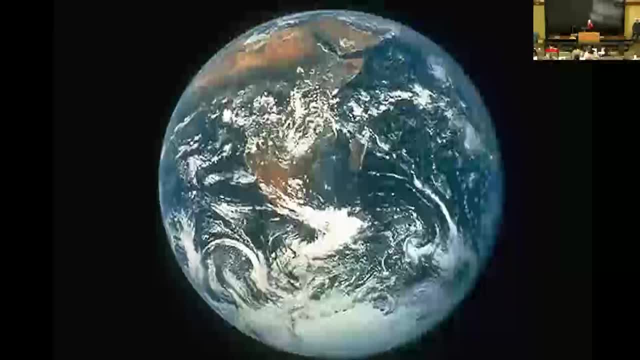 Yeah, I mean there are all sorts of reasons you know to to conserve species. but just from an objective, looking at different processes, yeah, some species were aware of are that have played more important roles than others. 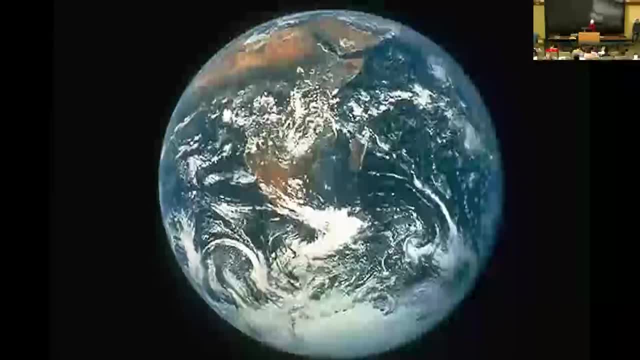 When you were talking about the mosquitoes affecting the Hawaiian birds, you kind of mentioned how the inoculation of the mosquitoes was the main solution, I guess. but wouldn't just vaccinating the birds be more effective? Well, so, in theory, so yeah. 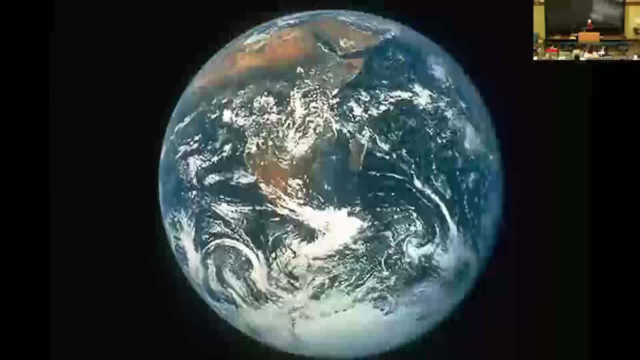 the, the mosquitoes. what they're trying to do is they're using, you know, new technology and like gene drive technology to really accelerate and basically change. I can't. I mean, it's not quite my area, all right, They're basically making these mosquitoes to either those populations will. 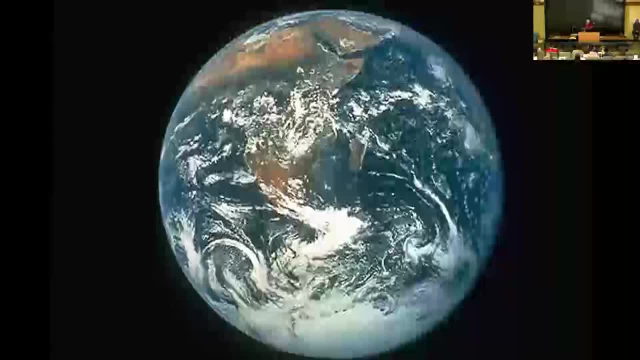 crash, I think, is what they're trying to get rid of, this one particular species of mosquito that's the vector for avian malaria. but that will- those changes will be able to move through those mosquito just in and of themselves when they're releasing those altered mosquitoes, Vaccinating the birds. 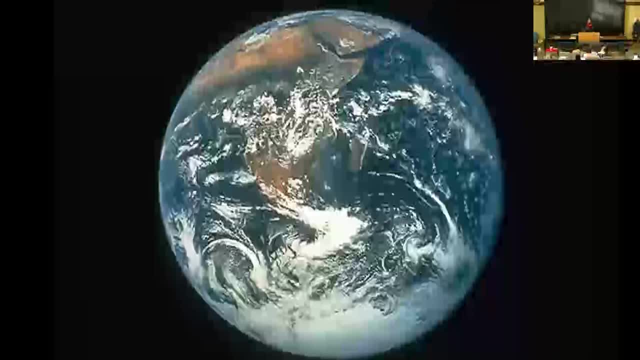 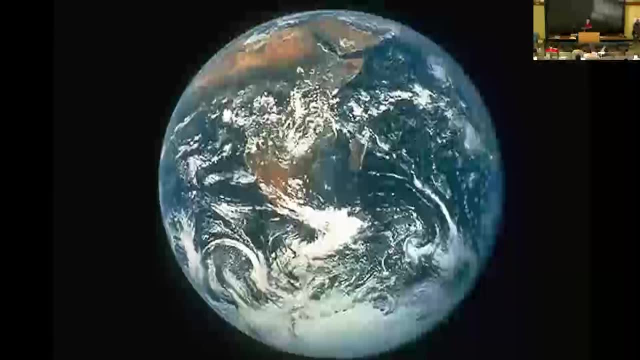 becomes hard. That means you have to catch them and you'd have to develop that vaccine. We don't have a vaccine for malaria, So that becomes not really possible or feasible. I mean, it'd be a great idea in some situations where we're able to do that, but in general that becomes really 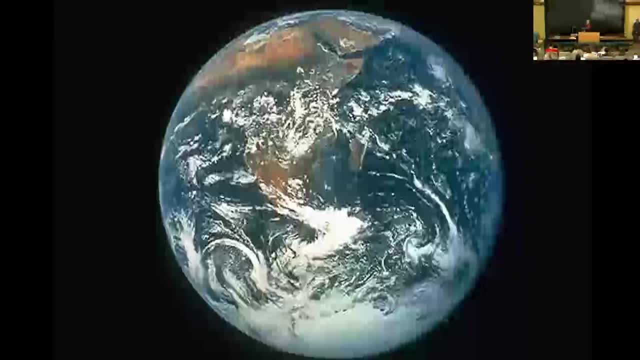 difficult. And two, you would have to continue to do that with all, with every year, with the young of the year you know, assuming that you know it wasn't. immunity was not passed on. you know maternally, So I also have a follow-up question regarding the mosquitoes and the zebra mussels. 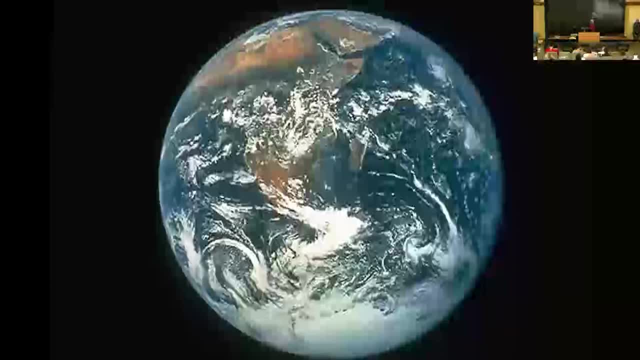 that were discussed as invasive species. How do humans aim to mitigate the effects or eradicate invasive species without harming, like, the natural environment? I feel like many of the attempts to say eradicate zebra mussels may have an effect on other species that live in the same water or rely on similar prey. So how do they go about making? 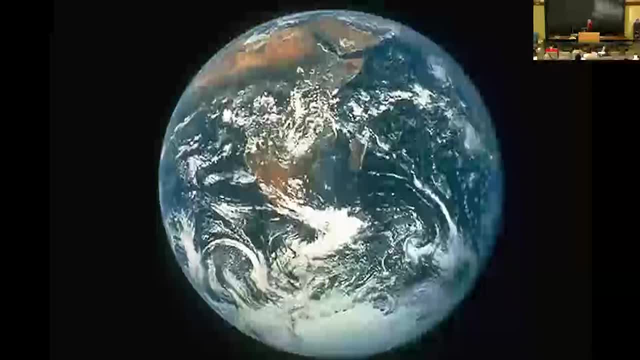 sure that they're not harming the natural ecosystem as well? Sure, that's, yeah, so good question. So with invasive species management, there are lots of different approaches that are used, But people use, you know, the best approaches are probably like if someone's 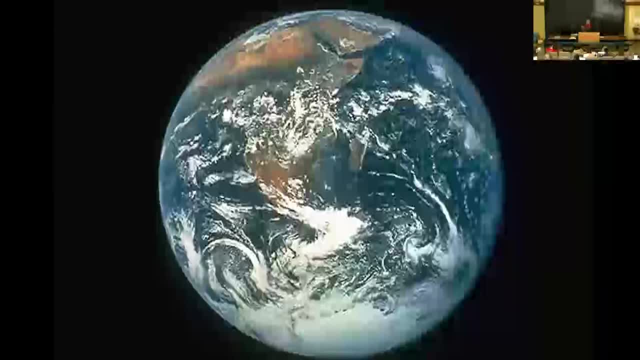 trying to, you know, get rid of an invasive species. they're not going to be able to get rid of it. So you know, some of you are in like more deal with, like pest management or that like. 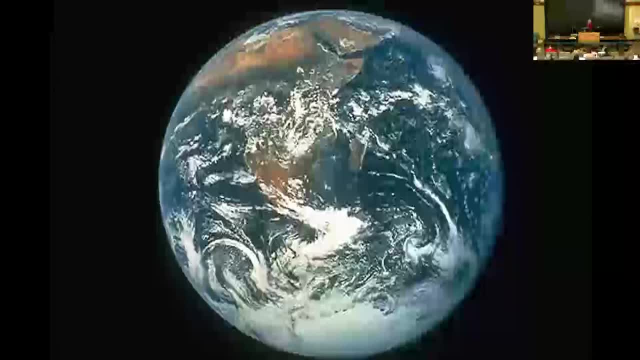 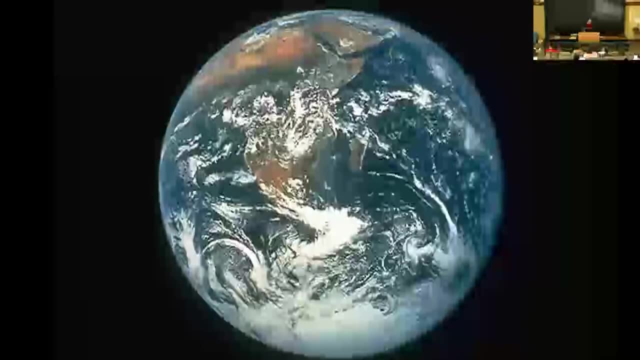 integrated pest management. It's more of an integrated approach where people are trying to look at: all right, how can we address causes of introduction? right? So reduce the flow of those species coming in through education, awareness, regulation, whatever, And then can you manipulate. 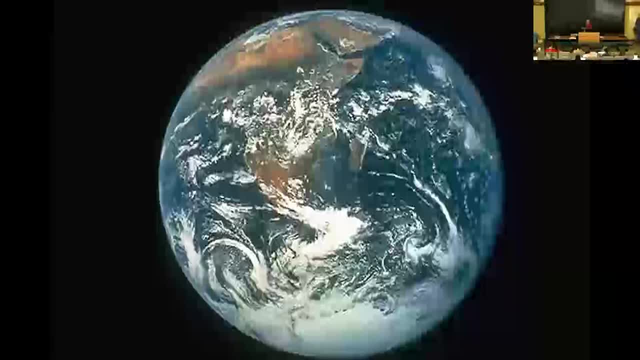 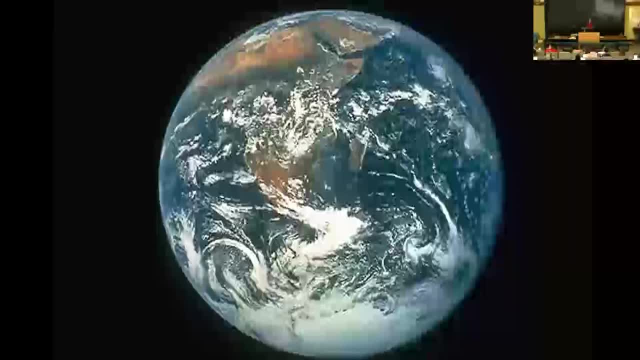 removal or control to suppress numbers might work in some cases. Biological agents: you know there's been more and more work, like with the mosquitoes. you know where you're looking at different biocontrol. like with the hemlock woolly adelgid- they found that there's an insect in the 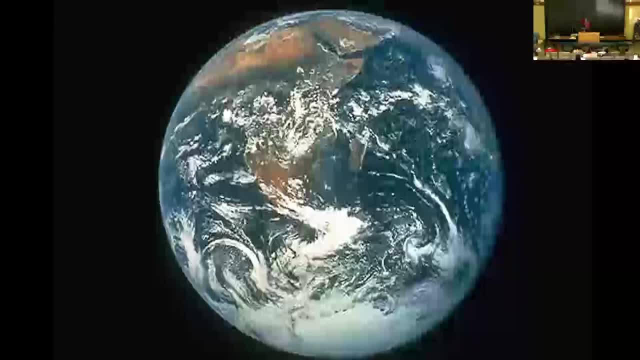 Pacific Northwest that eats the adelgid and doesn't eat other species, And so they're trying doing trials to see if we can use that here. So there are lots of different approaches that are used, But you're right, there have been some really bad outcomes in the past of efforts to 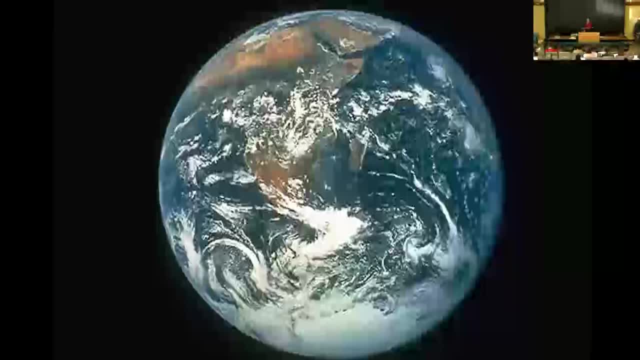 control invasive species And sometimes it can be really difficult, like in our. in the desert southwest there's a federally endangered bird, southwestern willow flycatcher. It now depends almost entirely on this invasive species, the salt cedar that was introduced to riparian areas. 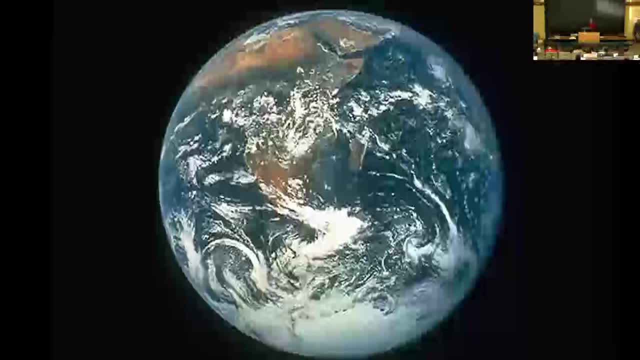 all the native vegetation is gone. So for those people who want the native vegetation to come back, it's like: well, if you remove this invasive species, then you lose this endangered species, and it becomes really complicated. But that, actually your question, reminds me of something. I was just reading, a news you know, like: 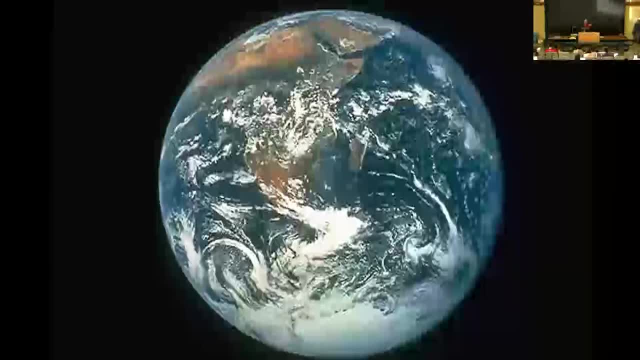 probably like all of you, I'll flip through the little news headlines on my phone And there was one about invasive species in the face of climate change just a day or two ago, And now there's a. there's a growing controversy and or dialogue. 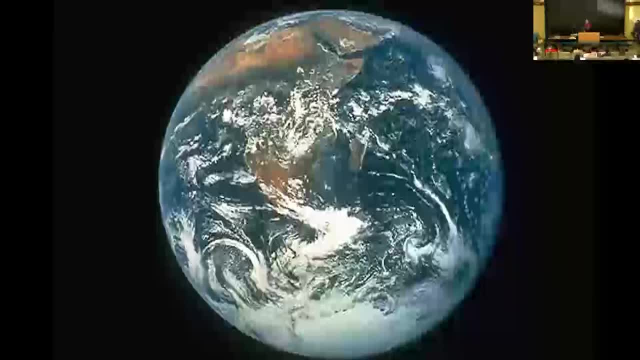 At least among ecologists- about: well, do we need to rethink what's invasive or not? So right, if we have a changing climate and now we're expecting- you're hoping- species are going to move to track those changes, At what point do we say, well, that species doesn't belong here. 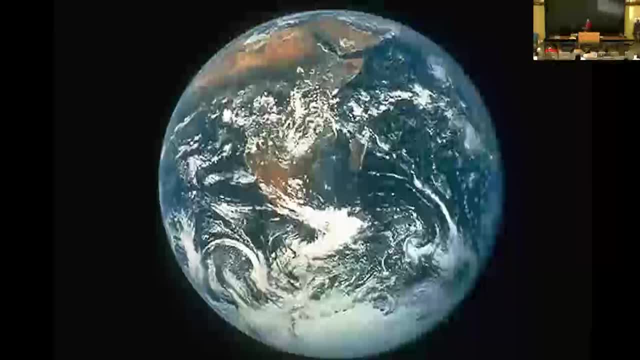 right. If we have some species that used to maybe not occur in New York. they occurred farther south, but the temperature warms. now they're moving. You know they're here. should we eradicate them? Are they non-native? Are they invasive? Are they? 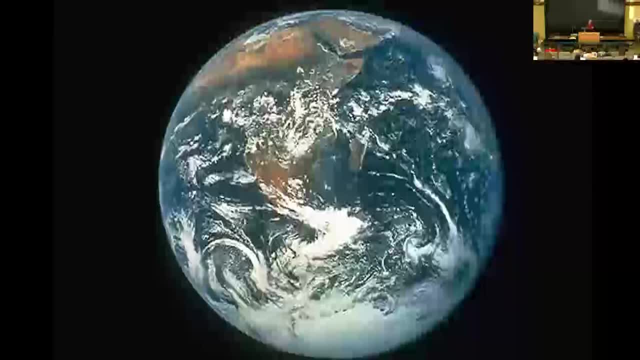 right, It's so it's. it's a very interesting problem. There are some people who say it's all. all bets are off. It's new communities, no analog communities. we shouldn't even waste our time trying to control invasive species. That'd be a minority view still among ecologists, But I 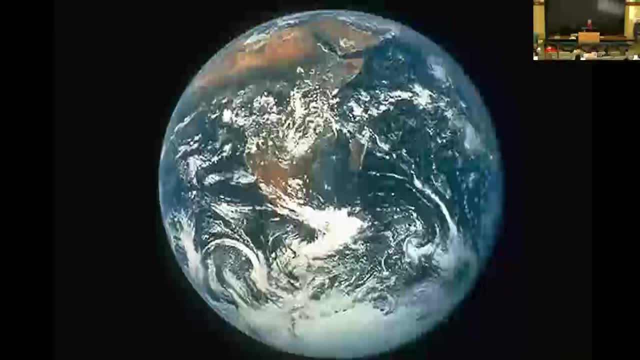 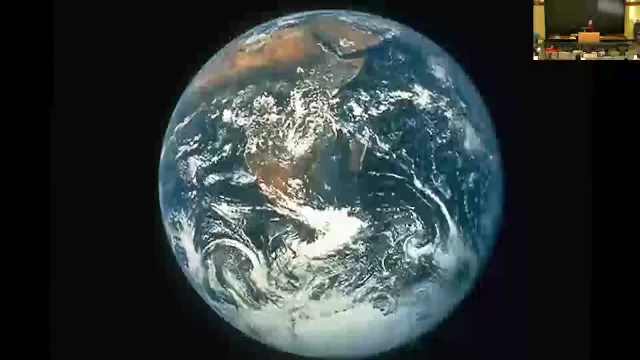 But do you think it's a problem of awareness that people aren't aware that bees are essential pollinators for the plants we're eating? Because, for lack of a better term- the average person like doesn't think of bees as important to our lifestyle and the food that we eat? Do you think? 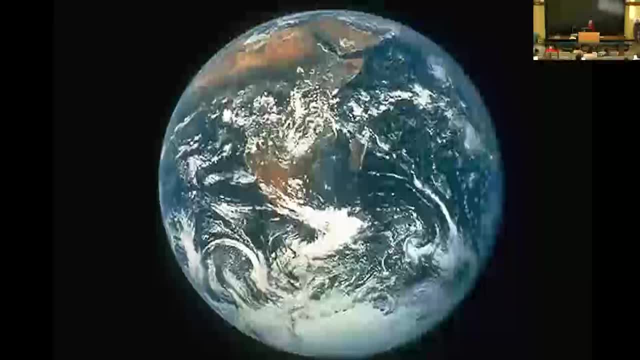 that the awareness is the problem, Or how do you think it's important to our lifestyle and the food that we eat? How would you promote the importance of them? Right? So I mean so in conservation, right, we have. I mean, there are lots of different. 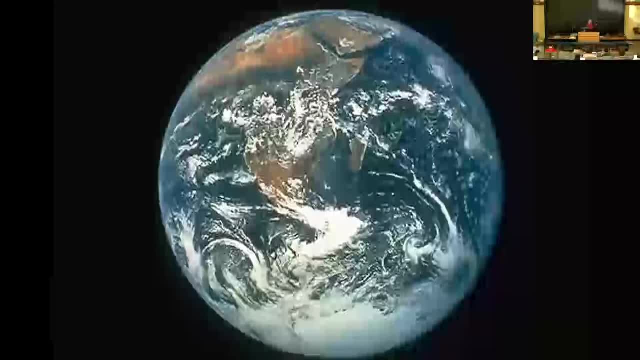 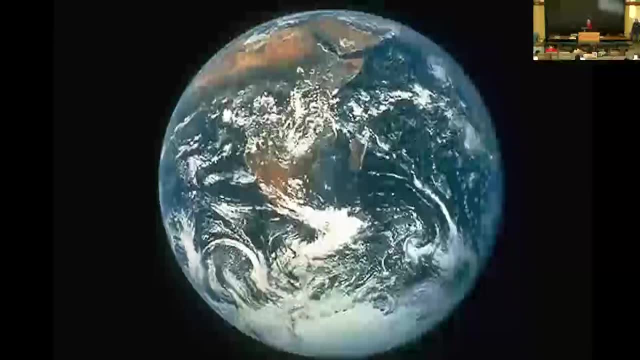 sort of pieces of that right. So awareness is one of them, And there are a lot of people who focus on environmental education And if we make people aware, then they'll make different choices And that might, you know, really create change In the case of pollinators.